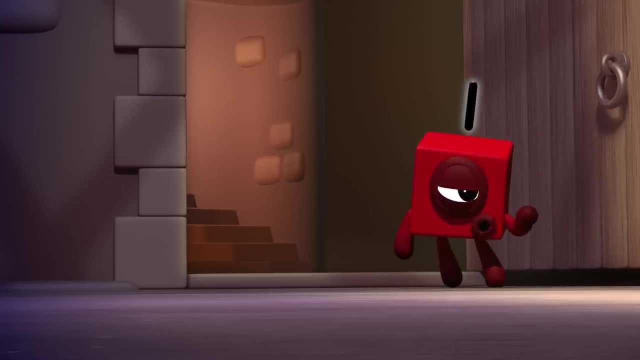 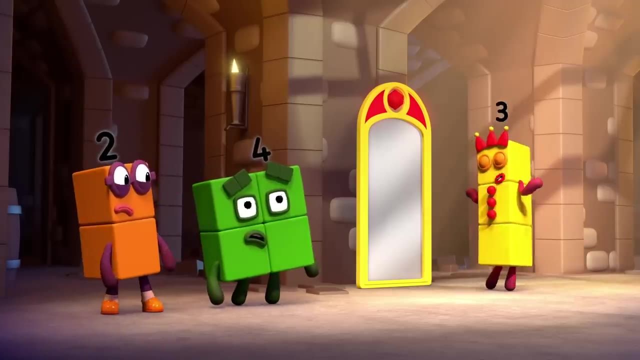 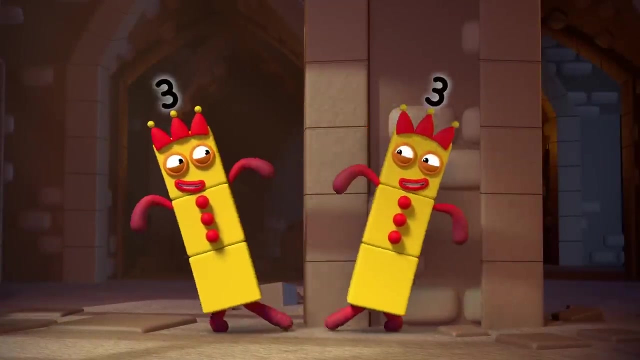 Keep an eye on it while I'm away And don't mess around with it. Right, my turn. One said not to: Oh, go on, It's only fair. Two lots, please. Two lots of three is six. Number six is on the floor. 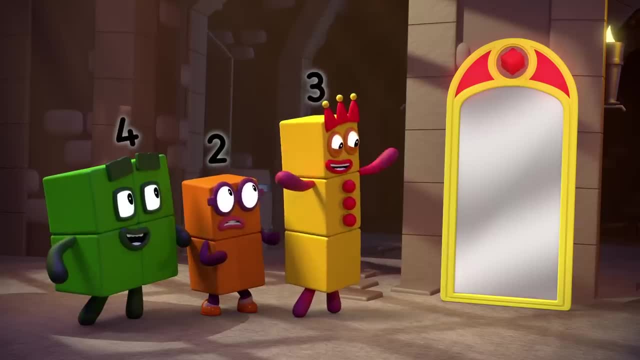 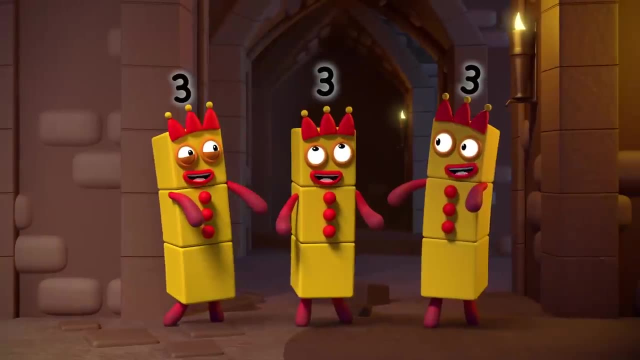 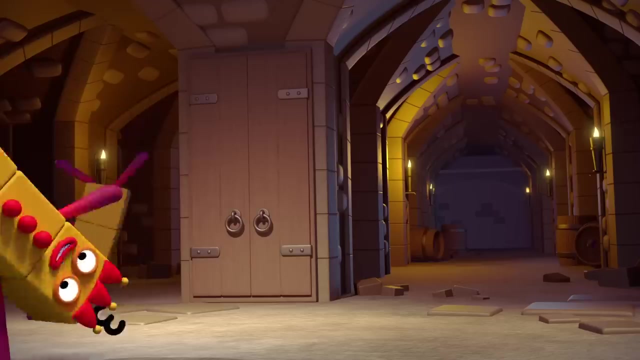 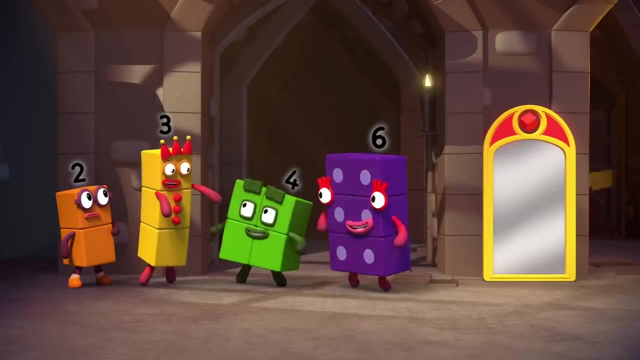 Don't be shy, Let's have some more Good idea. Three lots, please. Three lots of three is nine. I'm three, threes, see. Yay, We should probably stop now, But look, there are so many of us here already. 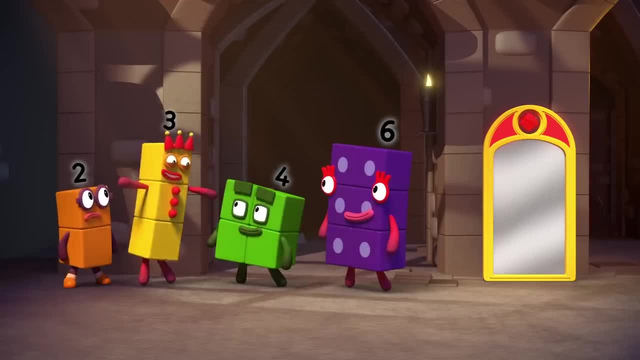 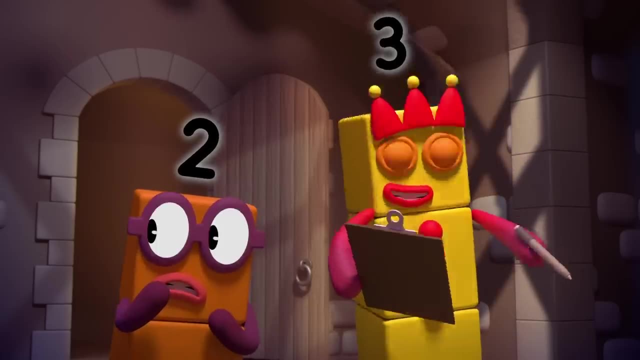 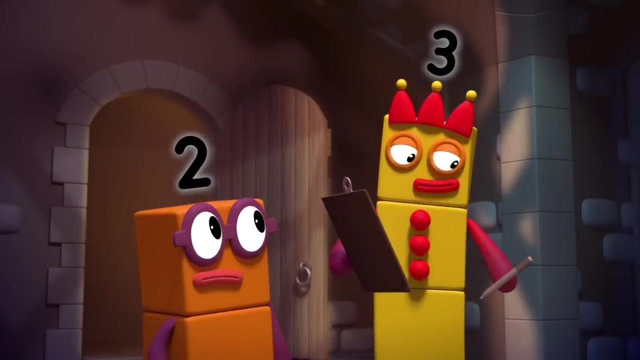 What would be surprised if she comes back and everyone's here. All right, then We've got two, three, four, then six. Oh no, We're missing five. How many, lots of? who is five? Hmm, Let's try you. 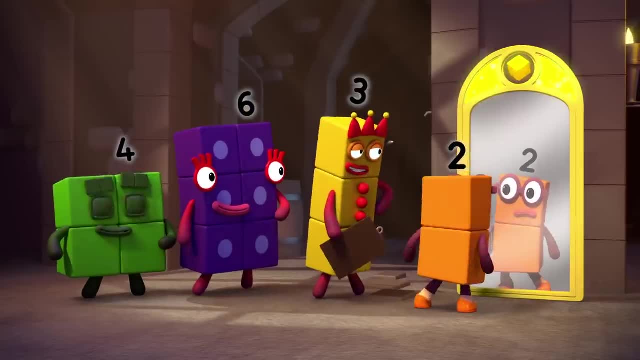 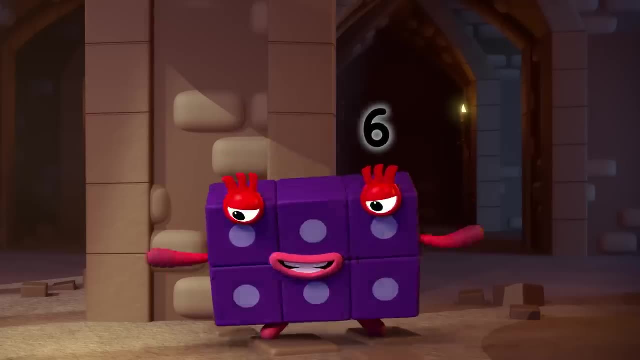 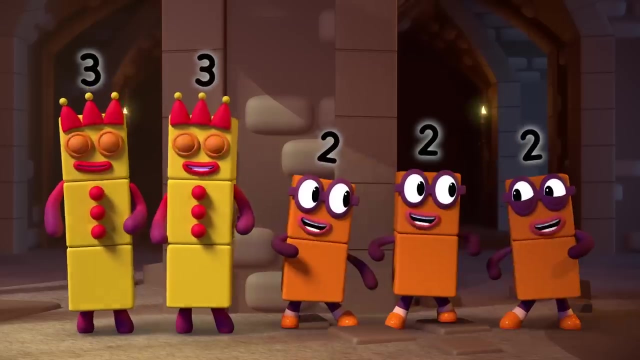 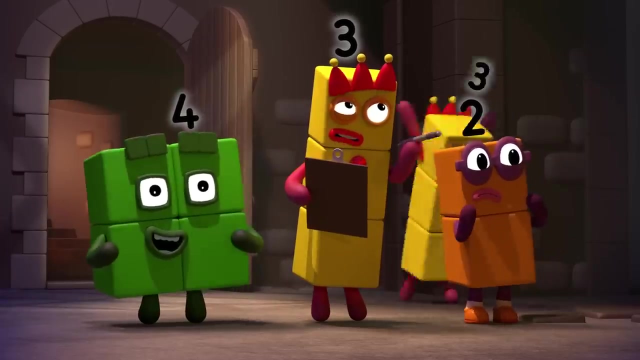 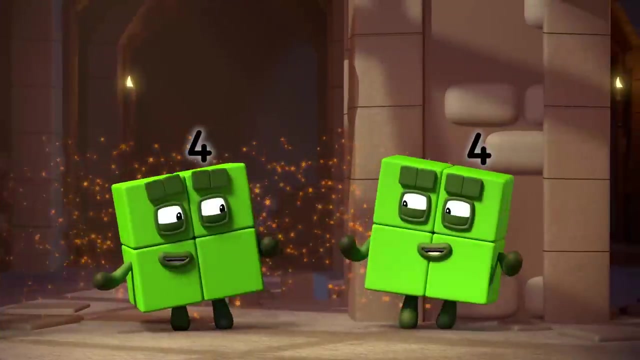 Oh, Three lots, please. Two lots of three is nine. Three lots is of two is six. Number six is on the floor. Wait, Have I said that before? Two lots of three. Three lots of two. I was hoping for a five. 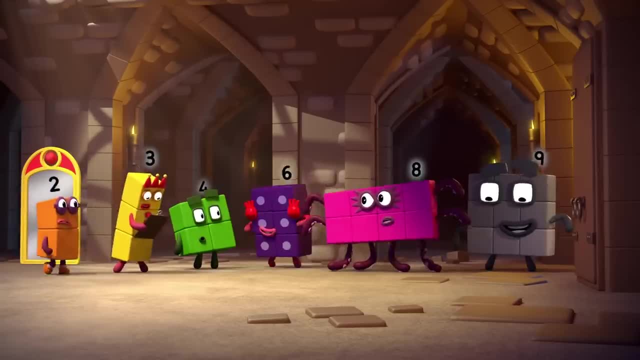 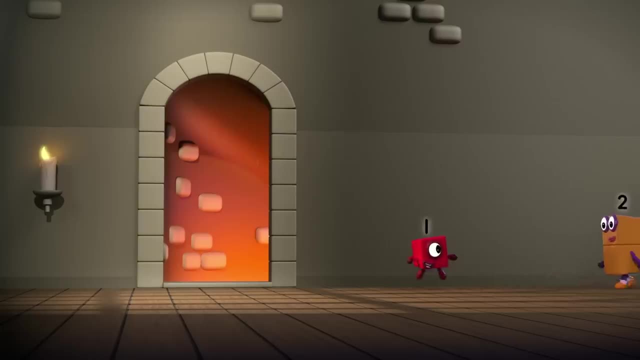 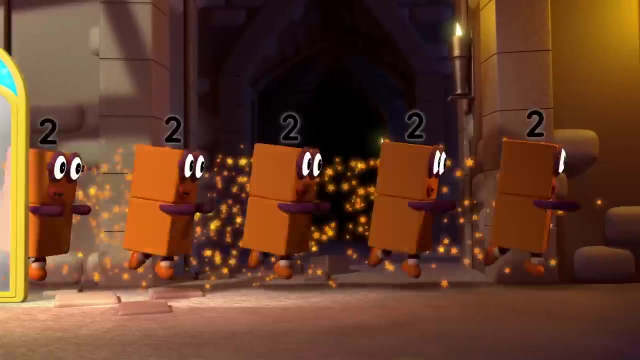 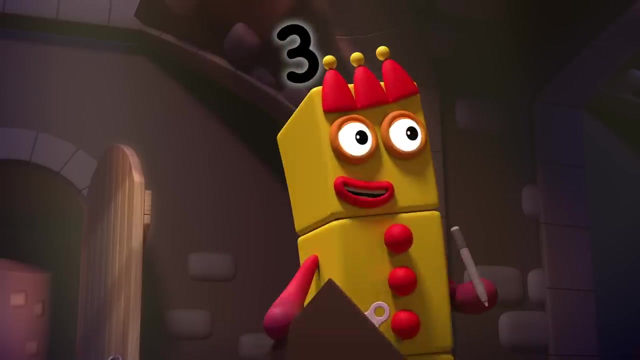 Maybe I can help. No Two lots, please. Oh, And we're missing seven and ten. Who wants to try next? It's a big surprise. Five lots of ten Is ten. That's ten sorted. All we need now is five and seven. 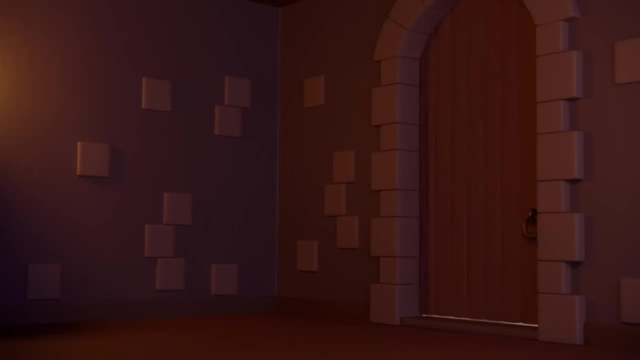 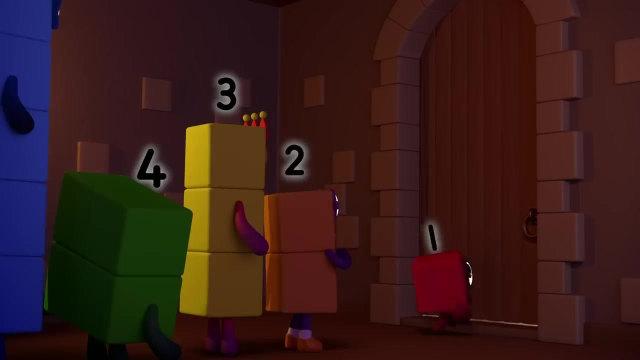 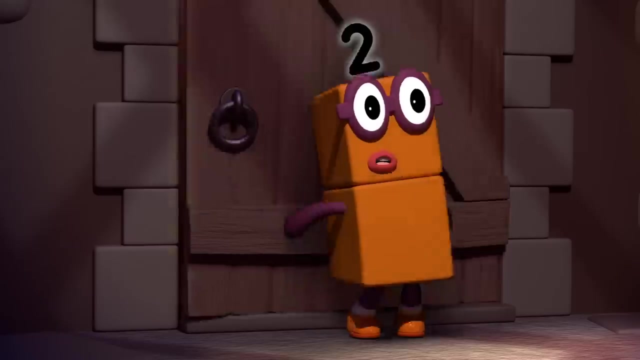 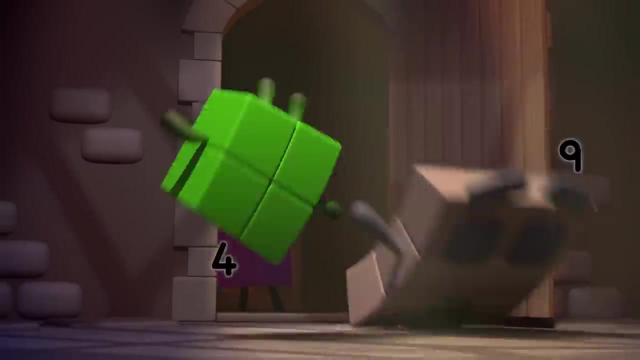 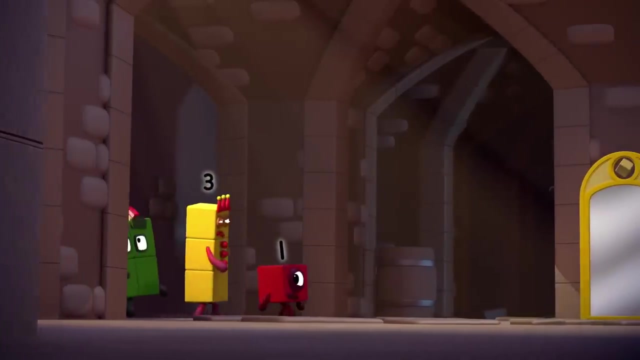 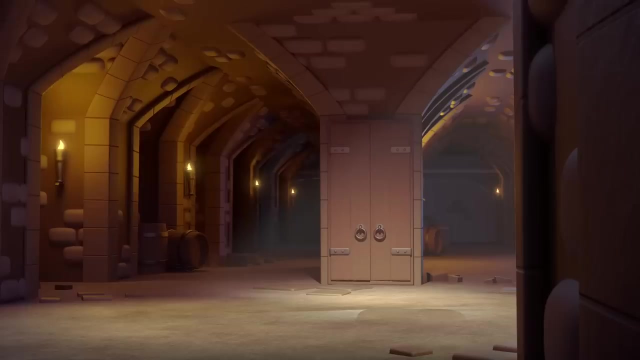 Next, Get ready for a really big surprise. One's coming Hide. Why can't we make five and seven There? Surprise, A magic mirror, Some big surprise. Ah, But what if I said I could make lots of number blocks appear all at once? 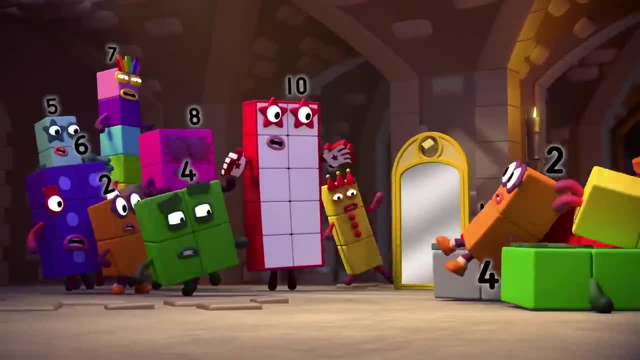 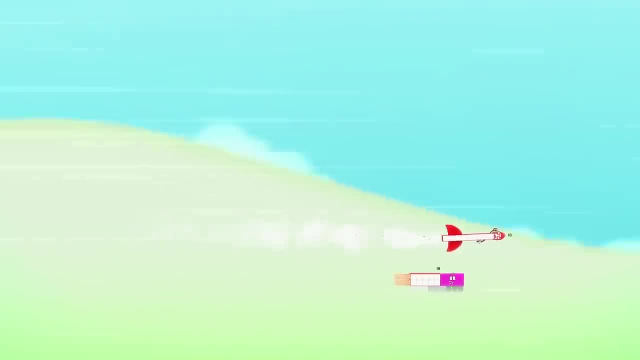 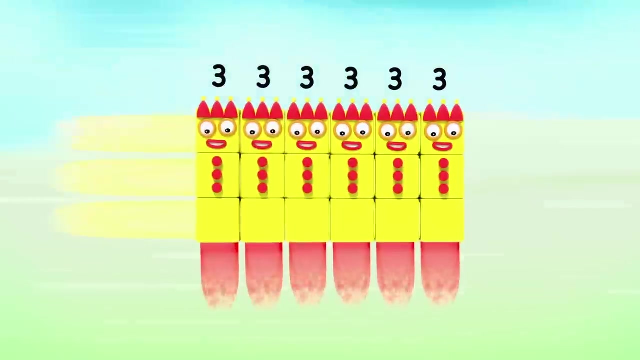 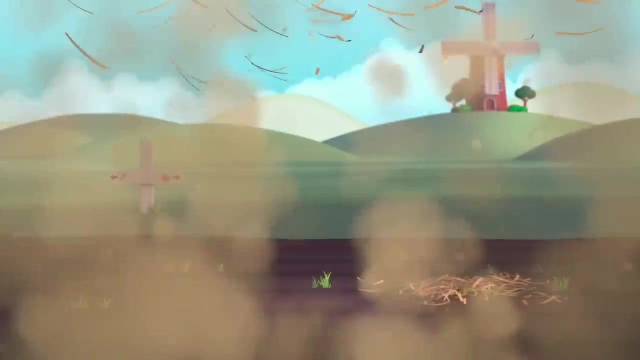 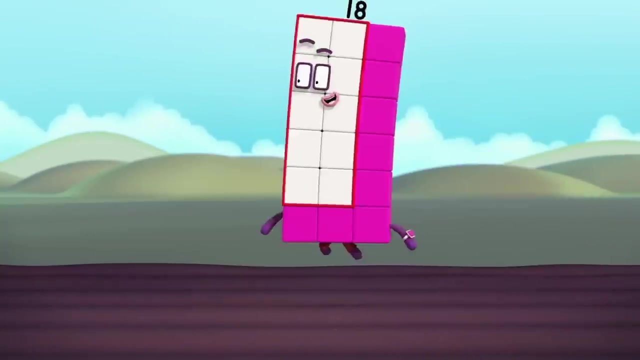 Now that would be a big surprise. Surprise, Woo-hoo, Here I come. I need more speed. Switch Three, Raise And away. Woo-hoo. Three, Six, Nine, Twelve, Fifteen, Eighteen, Oopsie. 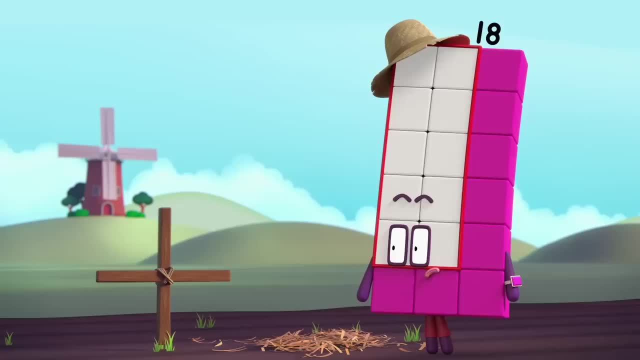 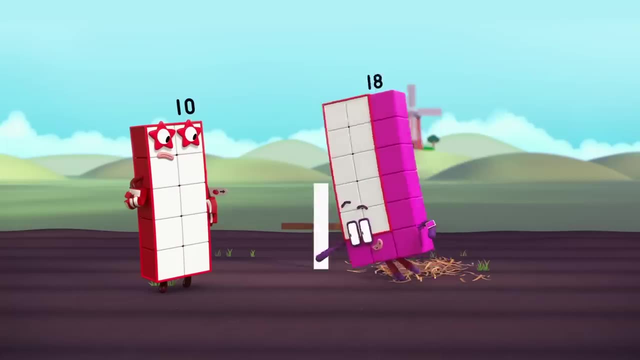 You know, I'm sure there was an old scarecrow here Scarecrow. No, Can't see any old scarecrow, Just this Great big plus sign. Hey, we can use it to practice adding up really fast. Oh. 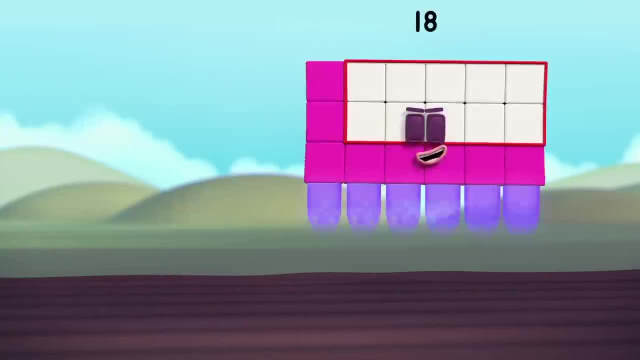 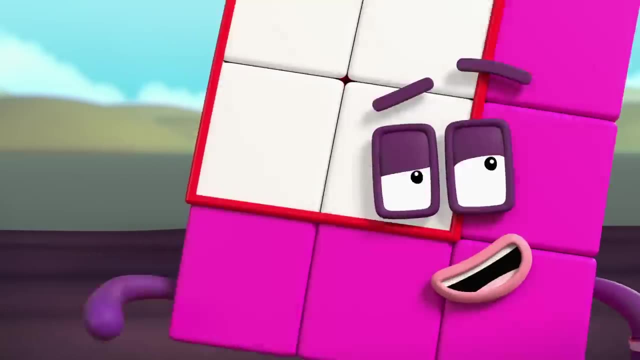 Three, Six, Nine, Four, Fifteen, Eighteen. I love that trick. Could you slow it down so I can see how it's done? Well, just this once On your marks: Ten, Three, Four, Three. 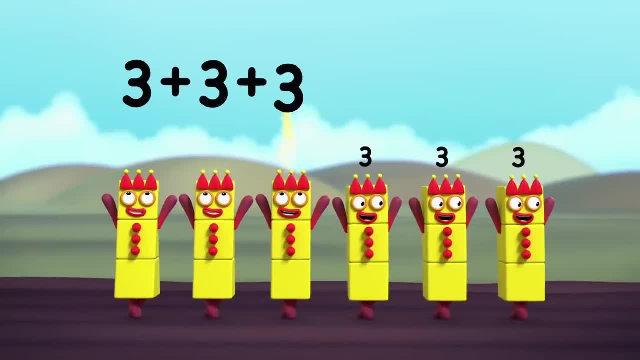 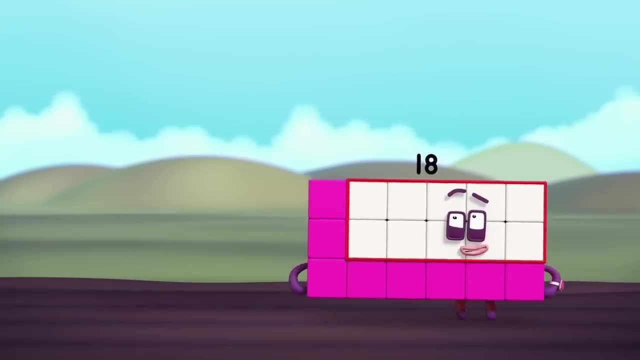 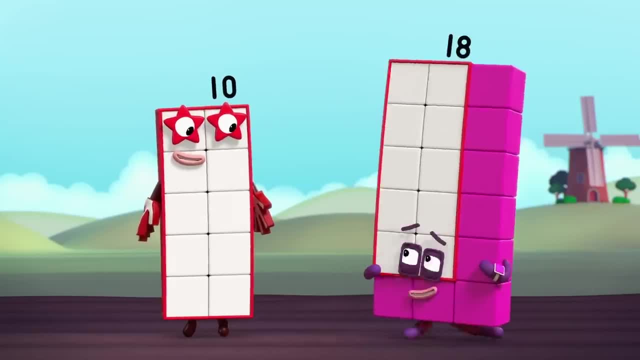 Um, All right, my friends, I've come to pan some square potatoes. Imagine the chips. Hey, where's the old scarecrow gone? So Ten Ready, yet I can't make a rectangle with three, No, No. 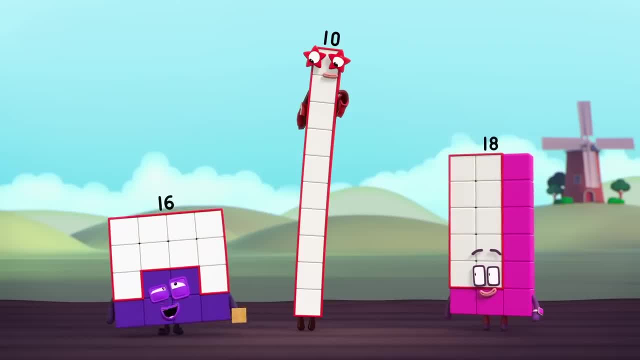 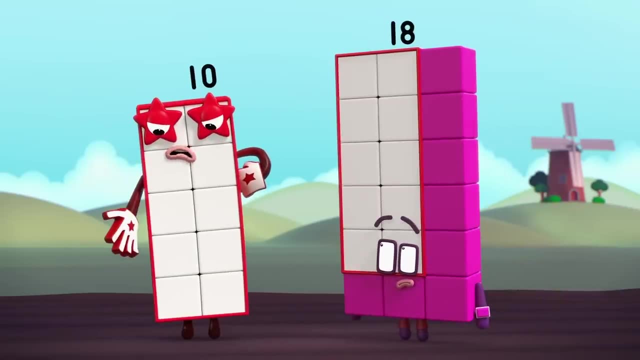 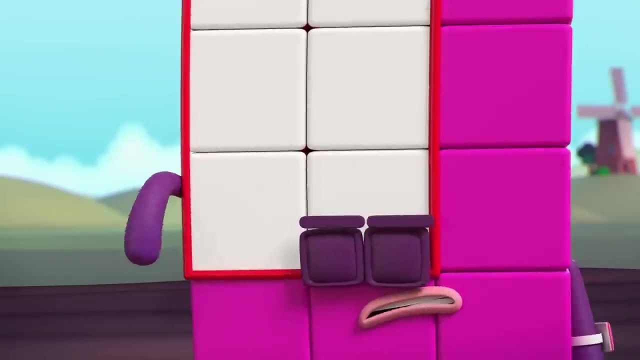 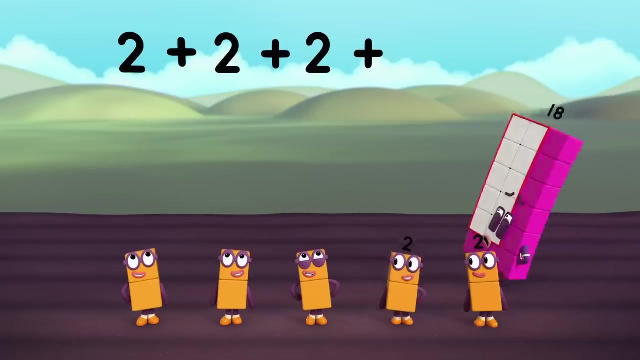 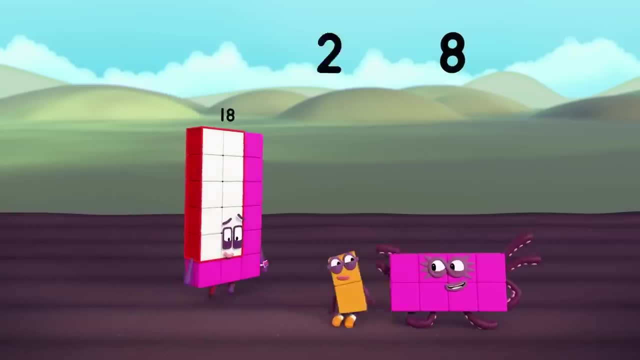 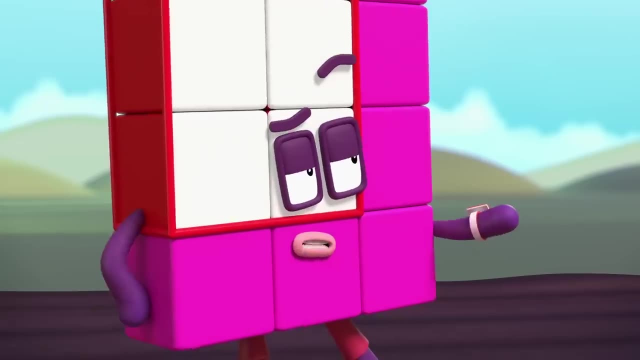 Four, Six, Eight, Ten. I added five, lots of two and I got ten. We got there in the end, But did you have to get extra for the next one in the end? but did you have to go so slow? 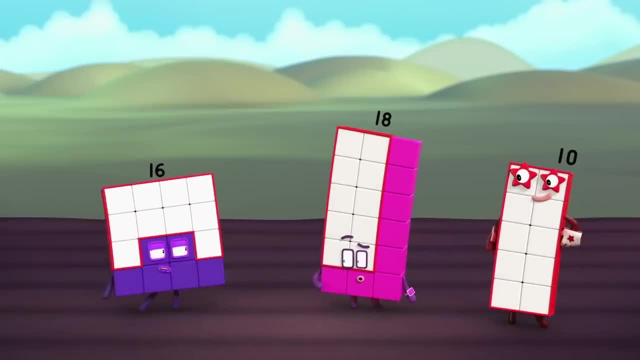 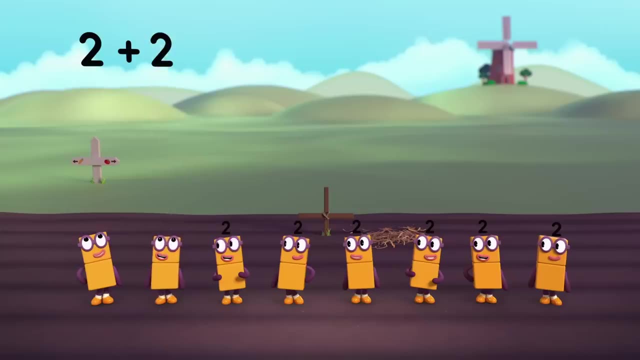 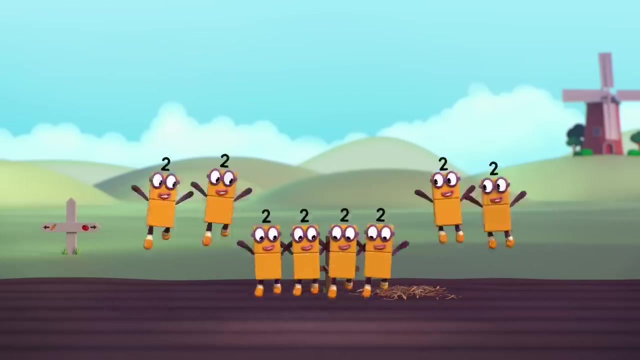 You like it fast, Let me have a go. You would believe your eyes. Two plus two plus two: This is going to take all day. I'm sorry, 18, but you made me lose count. Not to worry, I'll start. 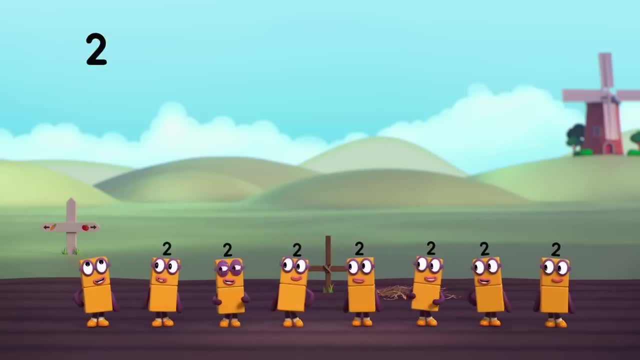 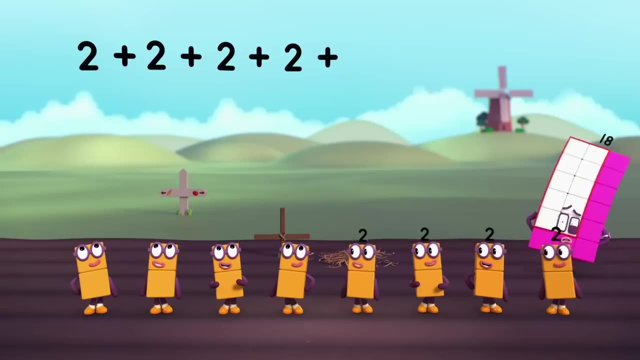 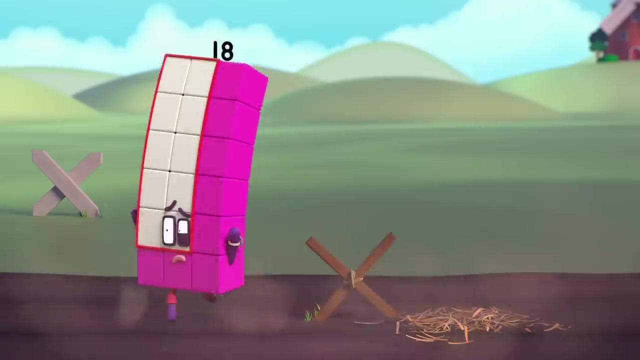 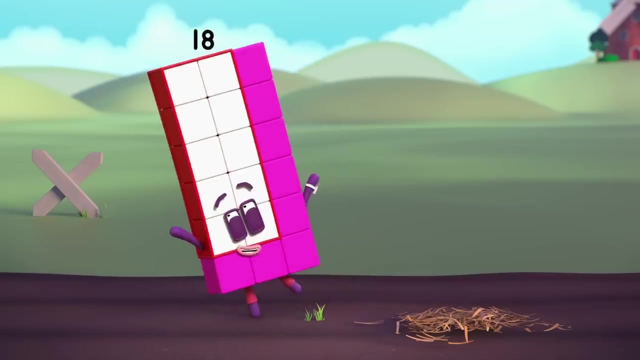 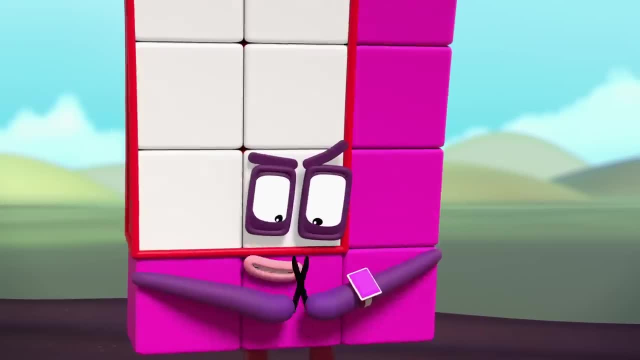 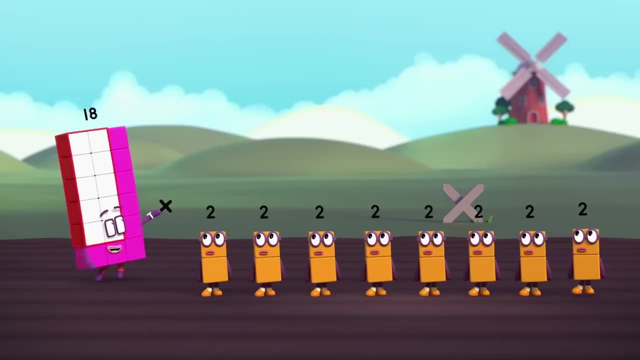 We don't need all these Squash. We can add a number lots of times Much faster with just one of these. I'll call it the times sign. I can use it to add something lots of times Super quickly. So how many twos are we? 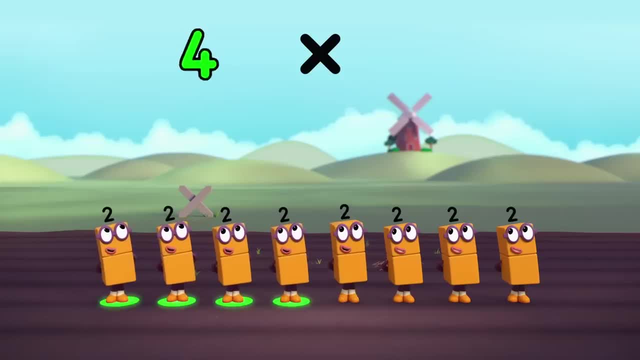 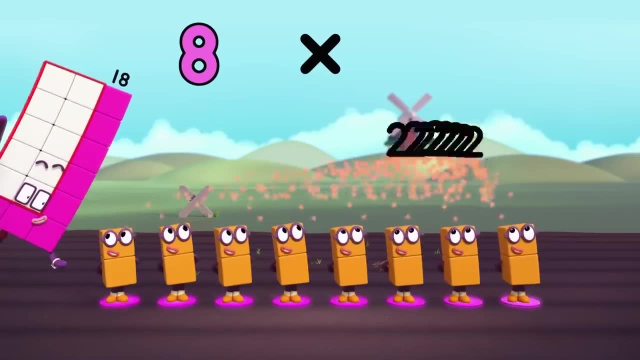 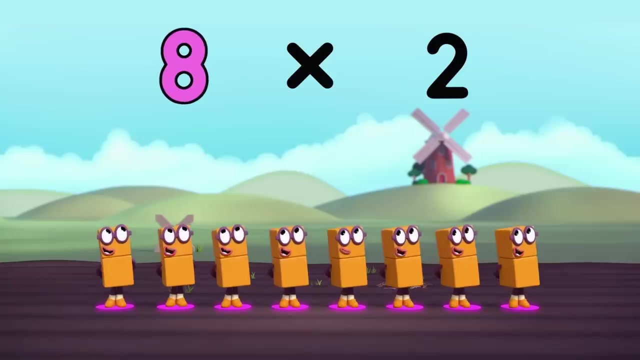 adding One, two, three, four, five, six, seven, eight, And remind what are we adding again? Twos, Eight, lots of two On your marks. get set: go Eight times two equals sixteen. 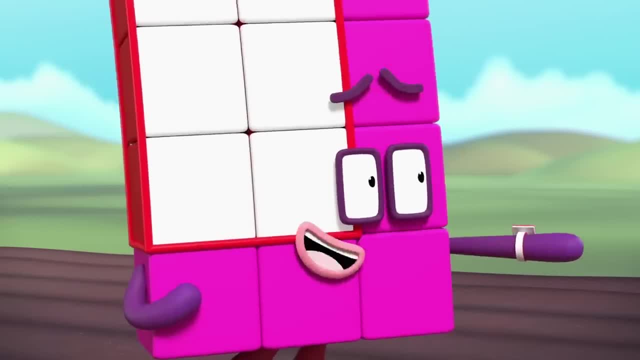 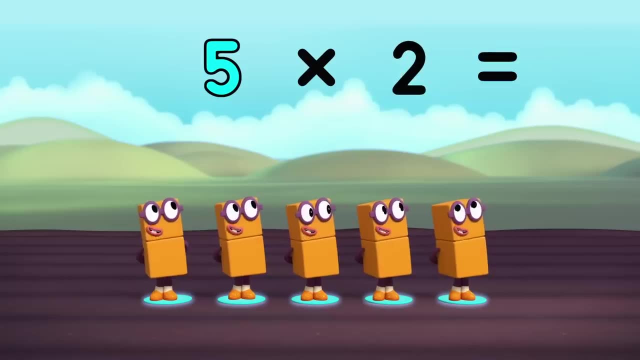 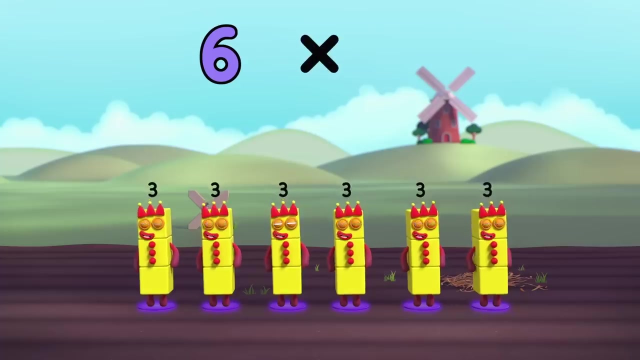 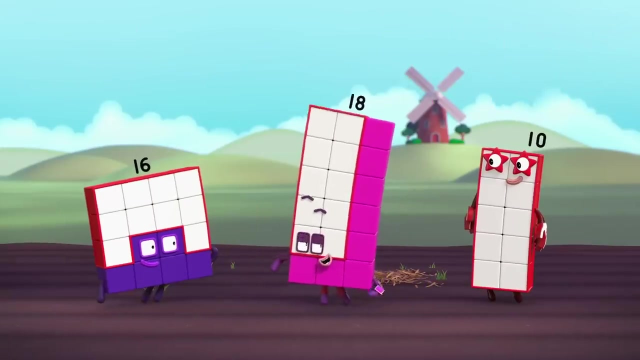 So much faster. Ten go again On your marks. There are five of us. Five times two equals ten. My turn. Six times three equals Eighteen. Refreshingly fast, This makes up for breaking some silly old scarecrow. 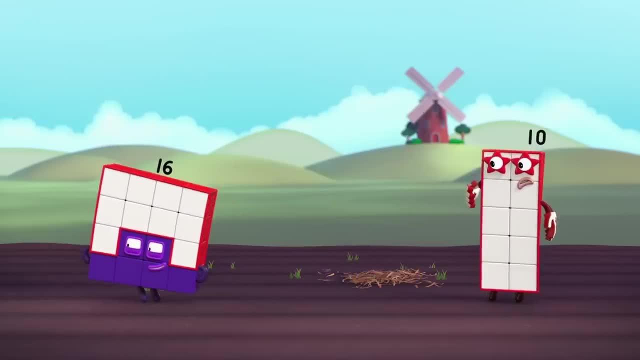 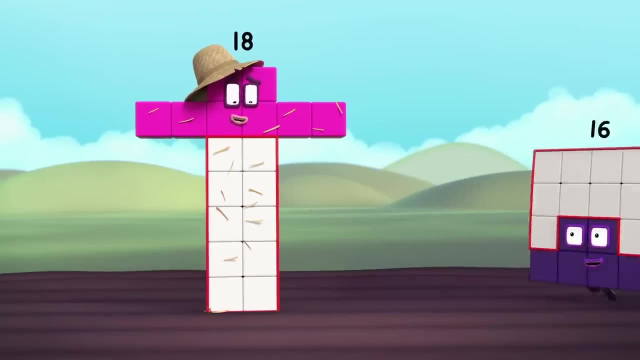 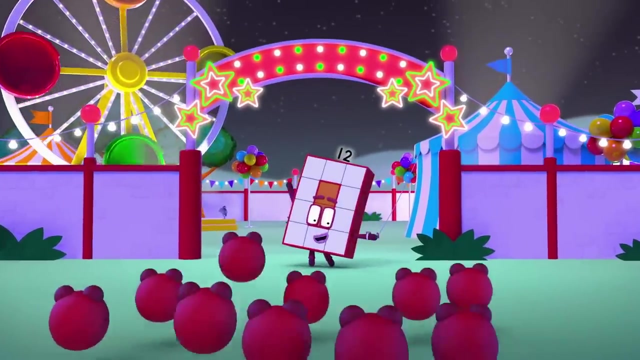 Whoops, Eighteen, Eighteen, No, I can't see any. eighteen, Just this good old scarecrow. Just this good old scarecrow. Just this good old scarecrow. Welcome, Welcome to the Fun Times Fair. Is everyone here? 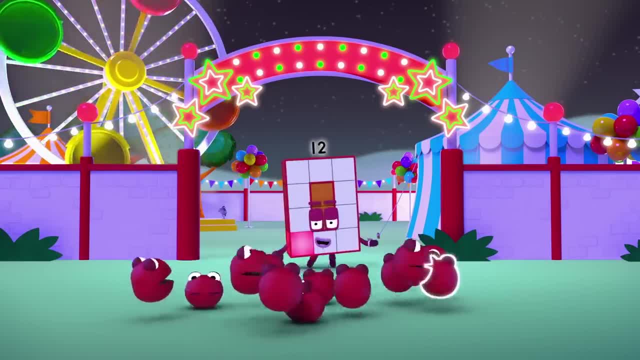 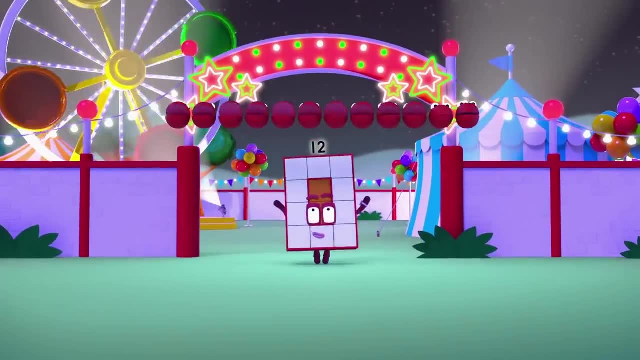 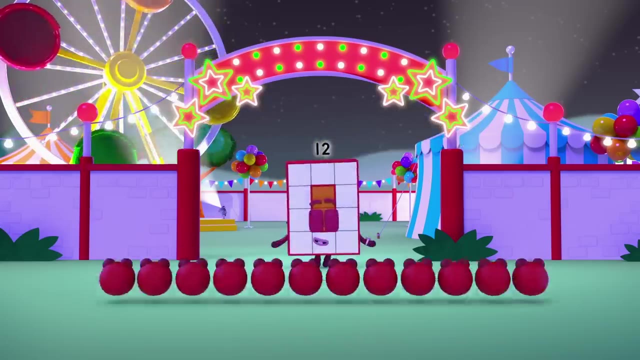 Yay, One, two, three, one, two. Oh, come here. Yay, One, two, three, four, five, six, seven, eight, nine, ten, eleven, twelve, Twelve, number blobs Good. 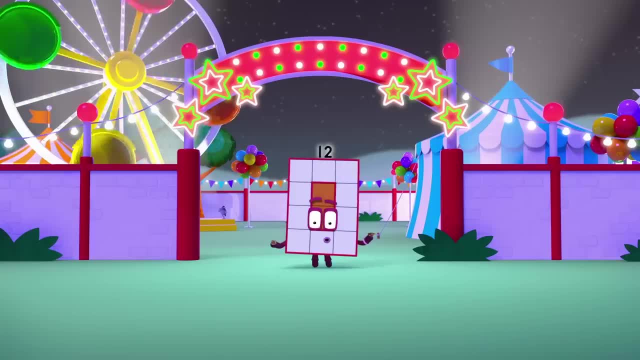 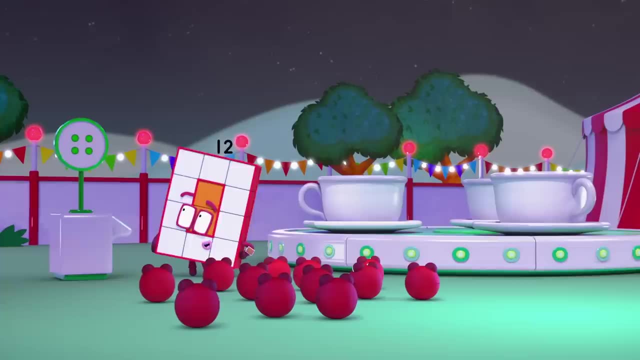 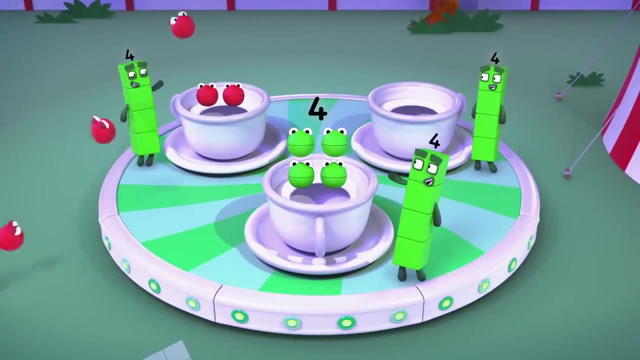 I've got lots of ride tokens. What would you like to The teacups, The teacups, The teacups. It looks like four to a cup, One, two, three, four. One, two, three. 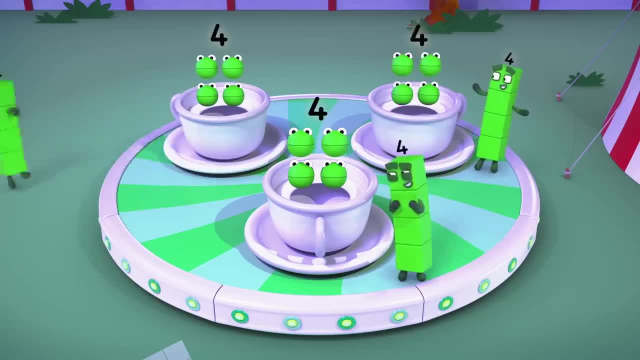 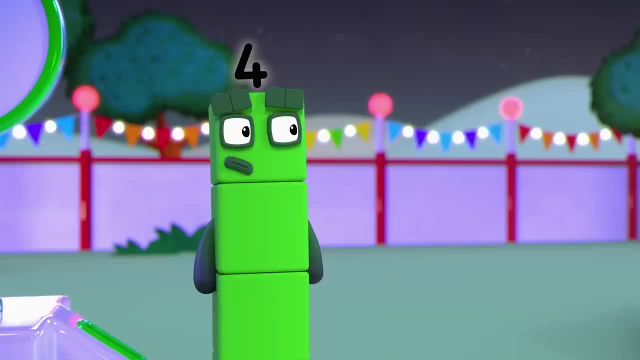 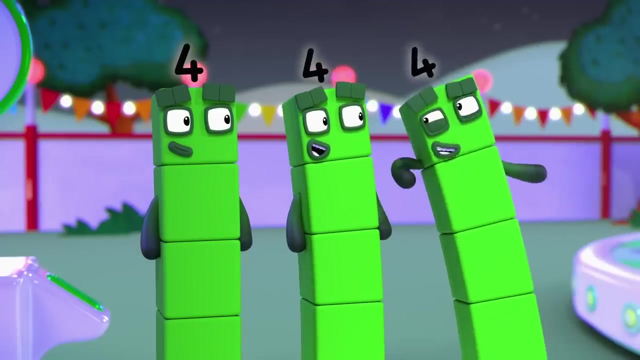 four. One, two, three, four. Now, how many ride tokens do you need? Um? Look at it this way: How many cups are there- One, two, three, Three cups- And how many riders in each cup? Four? 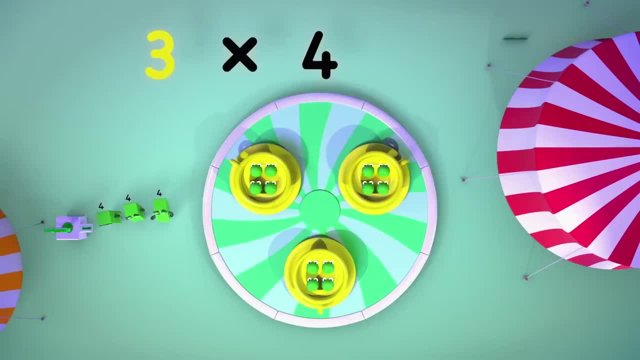 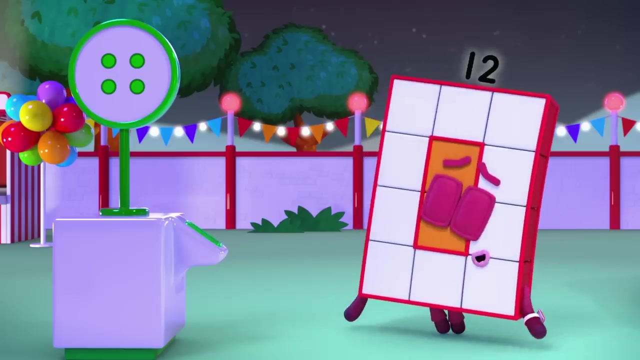 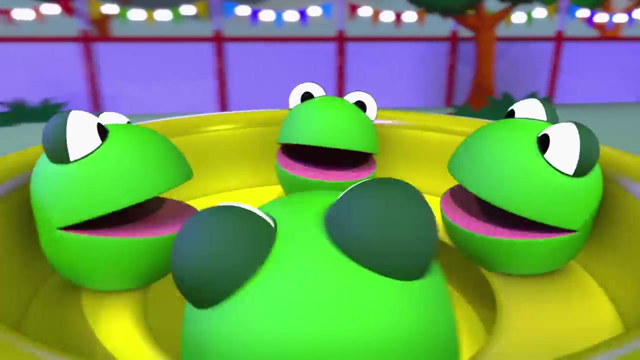 So that's three lots of four. Three times four, which is Three times four, equals twelve. Three lots of four is twelve tokens, And off you go, Watch us spin. three lots of four, twelve number blobs and not one more Whee. 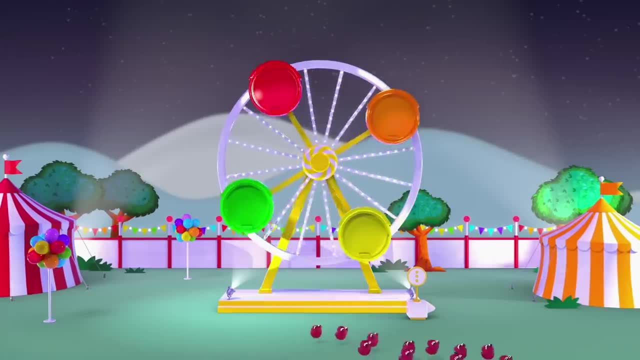 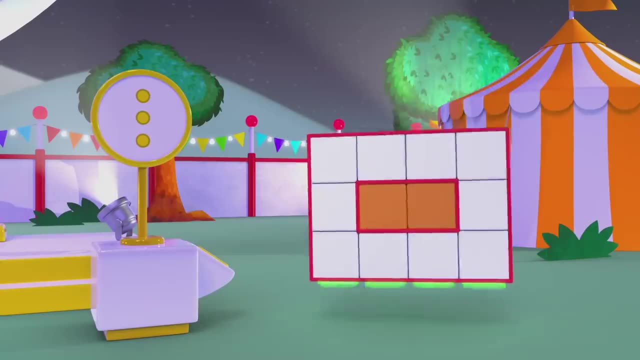 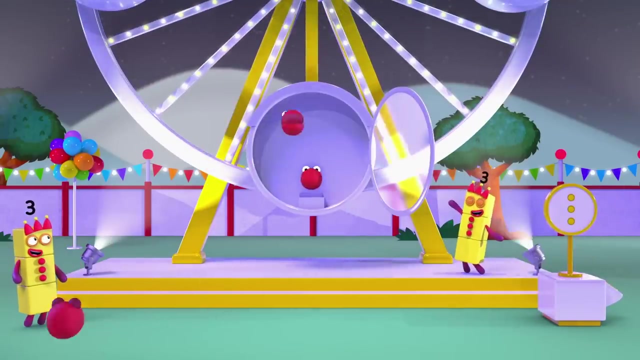 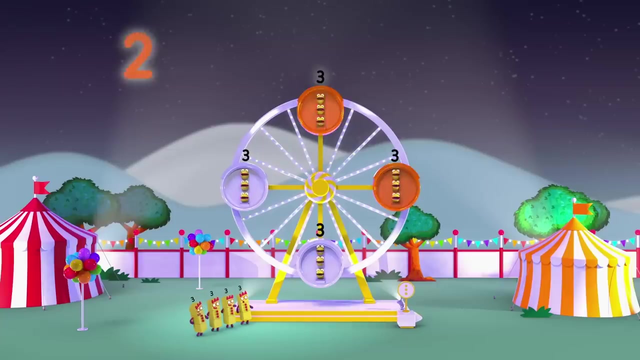 That was fun. So The big wheel, The big wheel, Aha, Looks like three to a carriage. this time Turn Three, Three, Three, Three Time for tokens. How many carriages? One, two, three, four. 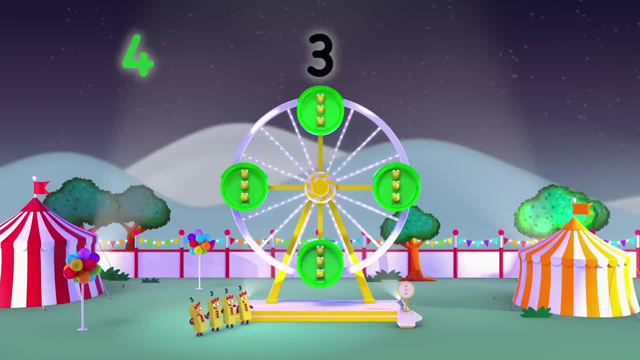 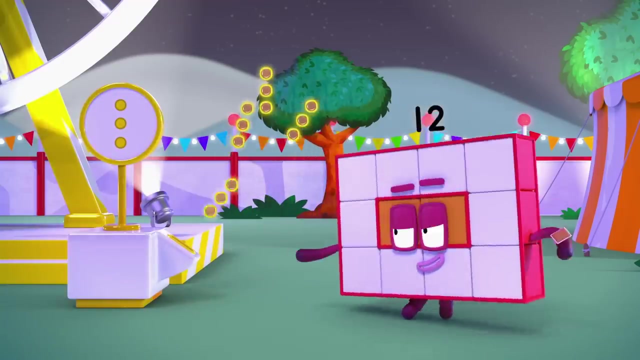 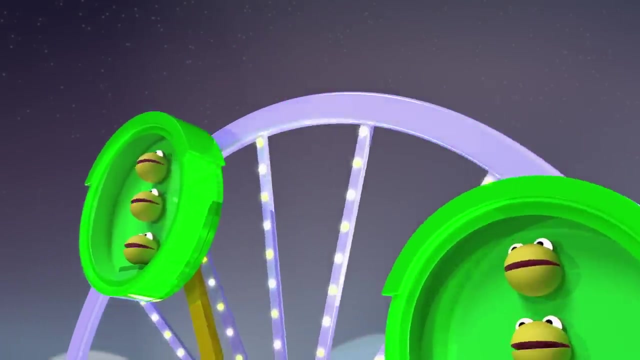 How many in each carriage? Three, So how many tokens do you need? Four times three equals twelve. Twelve tokens, Four, lots of three. Around we go four groups of three, twelve number blobs all going whee, Yay, Woohoo. 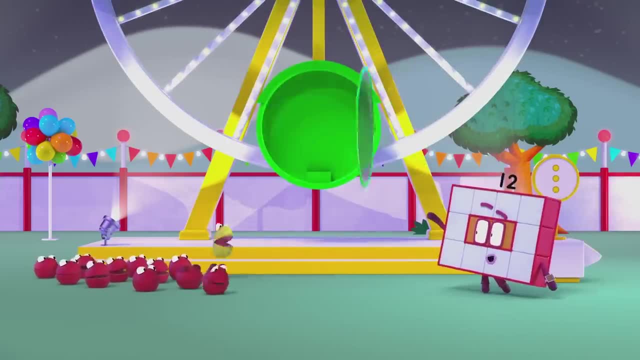 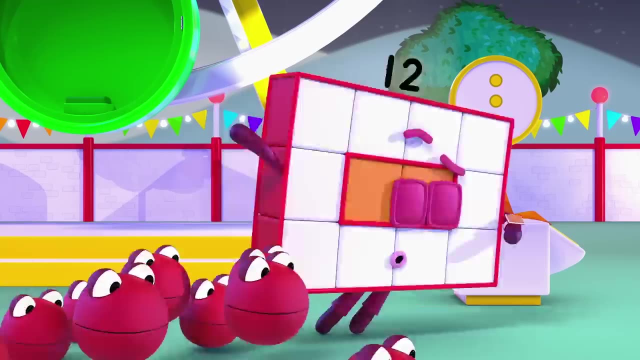 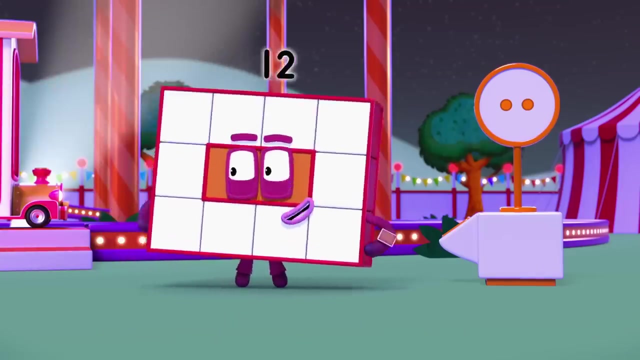 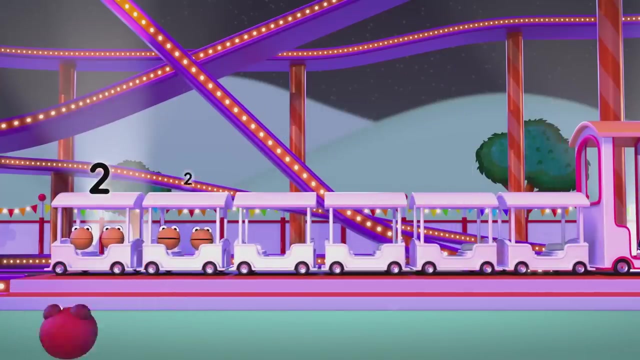 Woohoo, Now, little ones, are you ready for the fastest, most thrilling most? The Runaway Train. The Runaway Train, Hmm, In pairs, please Switch All aboard. Two, Two, Two, Two, Two. 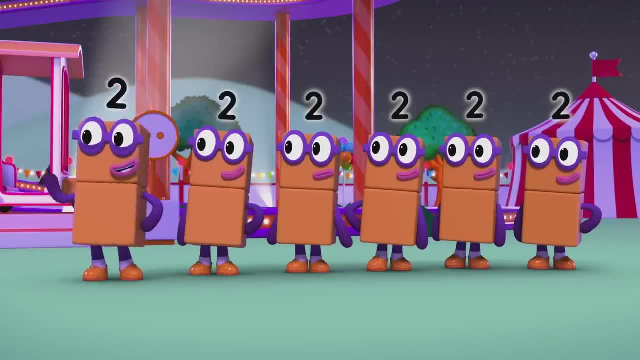 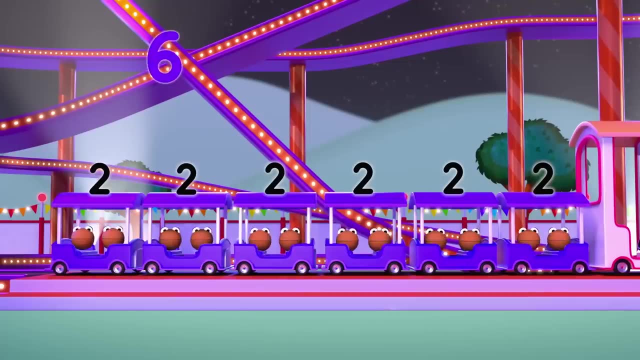 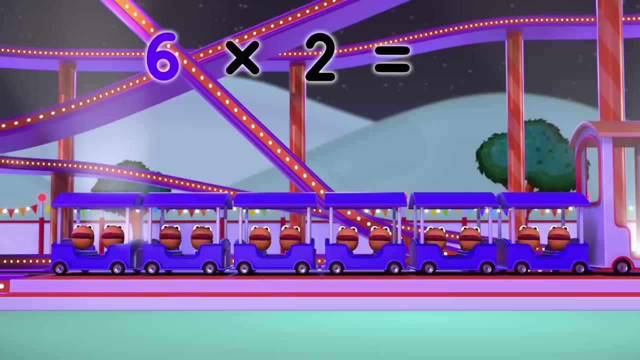 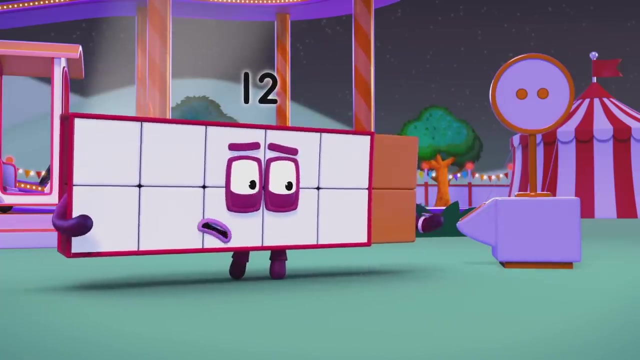 Two, Two. Now how many carriages are there? One, two, three, four, five, six, And how many in each carriage? Two, Six times two equals twelve, So you need twelve more. Oh, I'm all out of tokens. 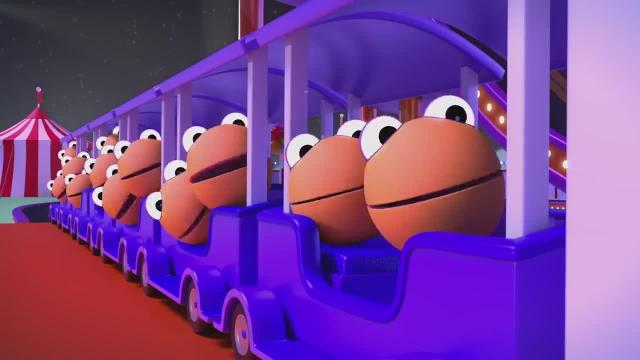 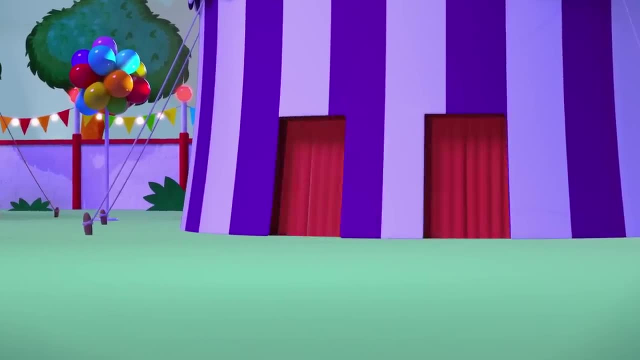 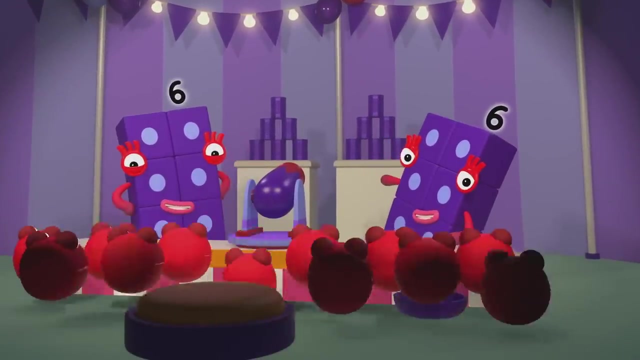 Oh, Ooh, Ha, Woohoo Ha. Roll up, roll up and have some fun. There's lots of tokens to be won. Ooh, We need twelve tokens. You'll win one for each can that falls and 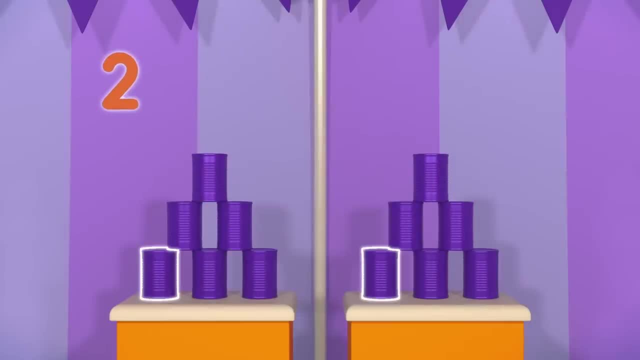 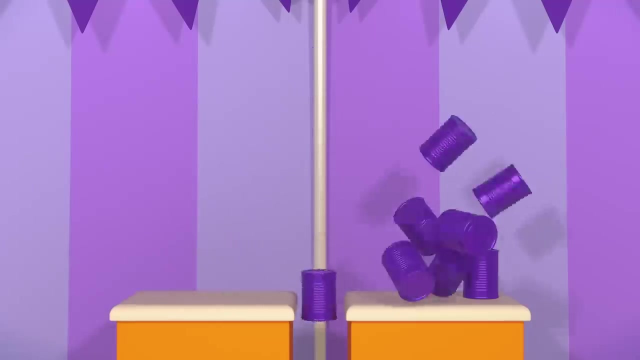 there's one, two, Two stacks. One, two, three, four, five, six, Six cans in each stack, And two times six equals twelve. Woohoo, Hooray, Hooray, Woohoo. Here we. 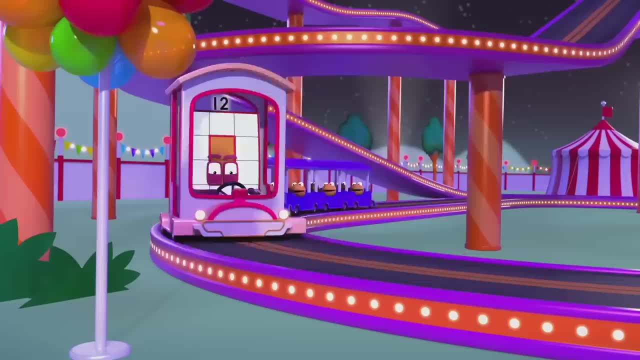 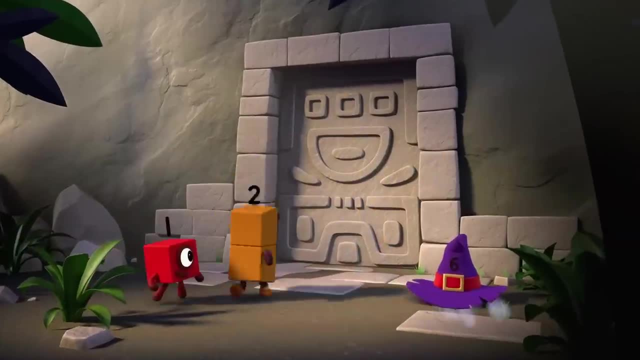 go Six lots of two, Twelve number lots: Choo-choo, Choo-choo, Woohoo, Ha-ha-ha, Ha-ha-ha, Ha-ha-ha. Greetings all, Let's see. 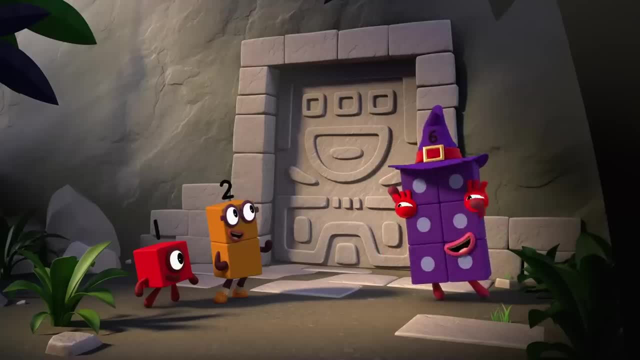 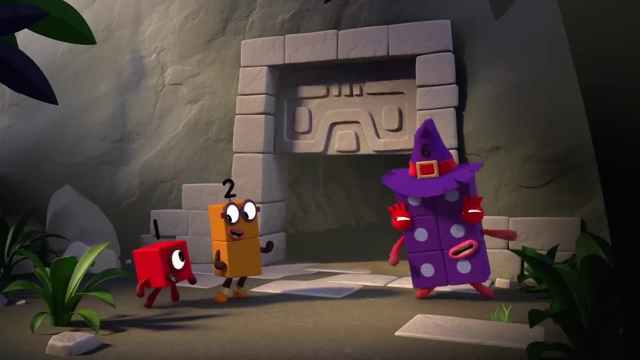 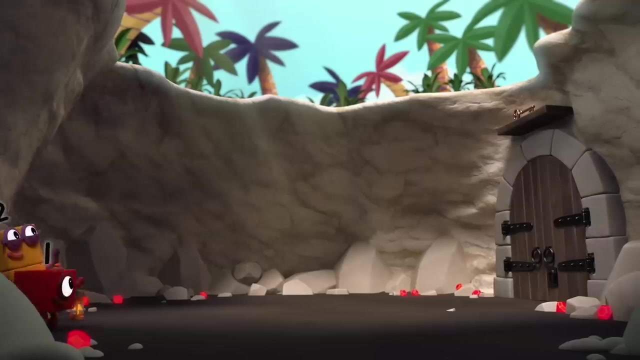 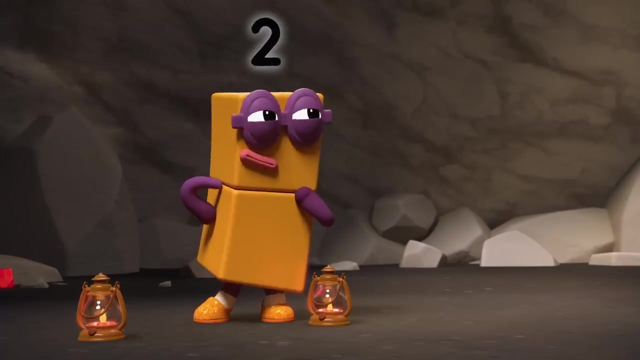 who dares to step inside the lair of shares. Solve the puzzles, but beware: The treasure goes to those who share. One for you and one for me. Wow, Ooh, It's locked. Look, There's a key, But how? 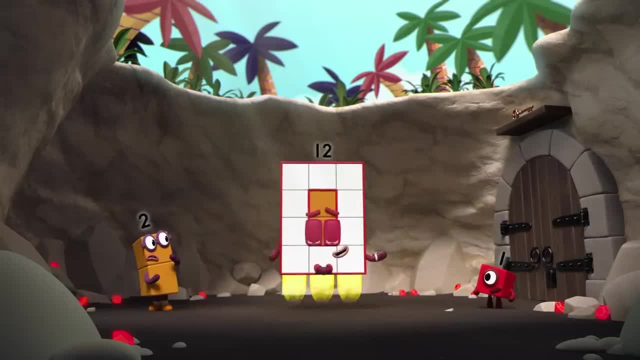 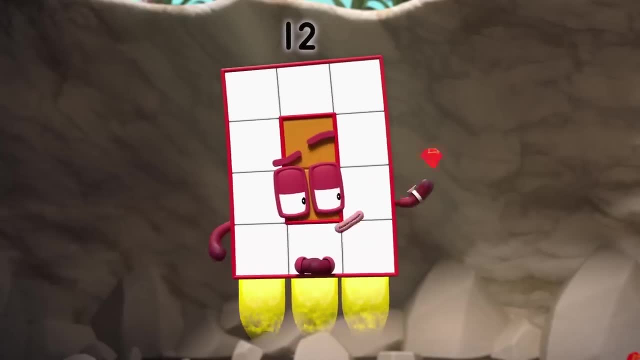 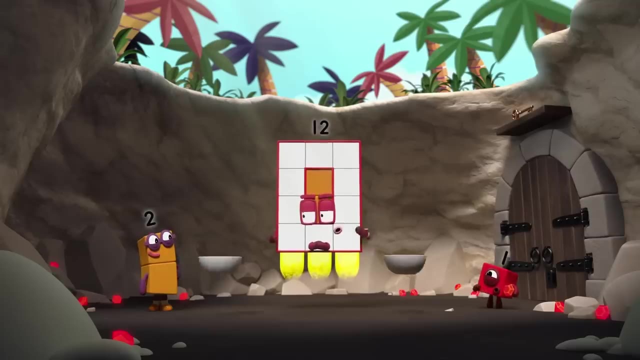 do we reach it? I am the genie of the air. Ooh, To win the first key, you must find all of my gems. But to make things trickier, you must share the gems equally between these two bowls And hurry When the sands. 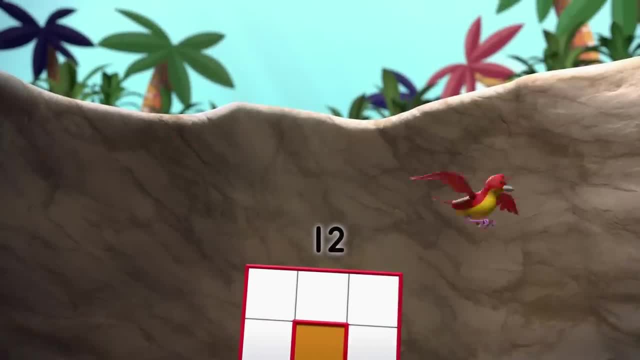 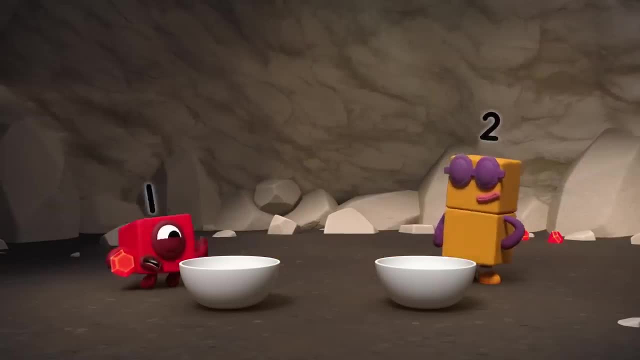 of time run out. a bird will fly off with a key. How can we put the same number in each bowl if we don't even know how many there are? Remember how we shared the lanterns: One for you, one for me. 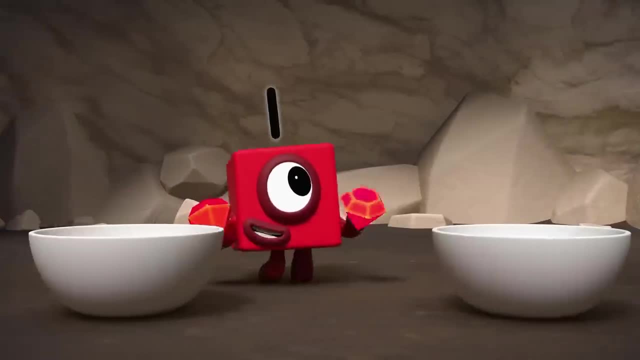 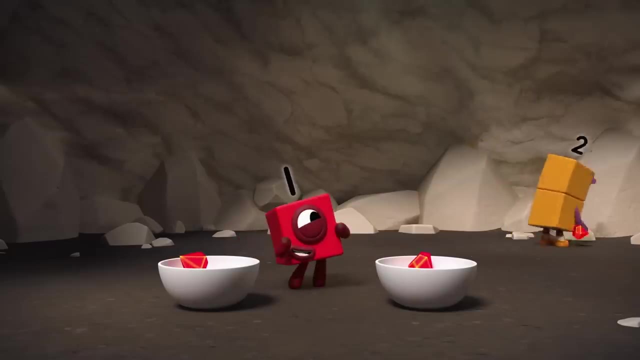 Yes, If we put one gem into each bowl in turn, they'll always have the same number of gems: One for you, one for me, One each, One for you and one for me. It's working, Two gems in each bowl. 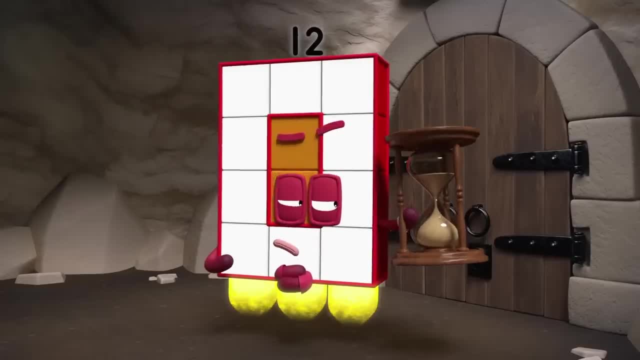 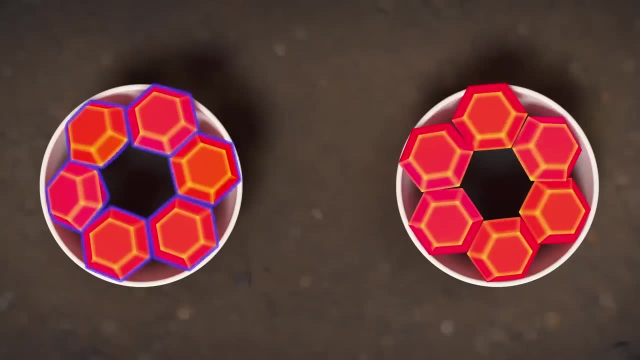 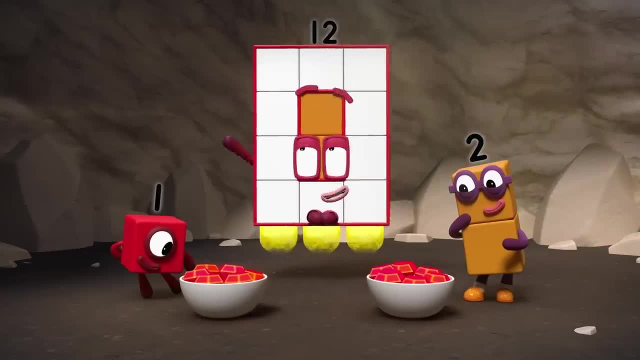 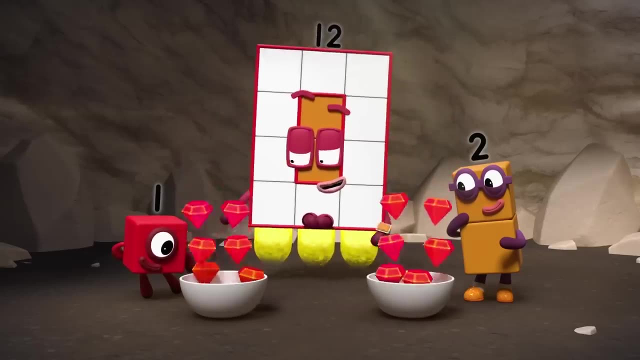 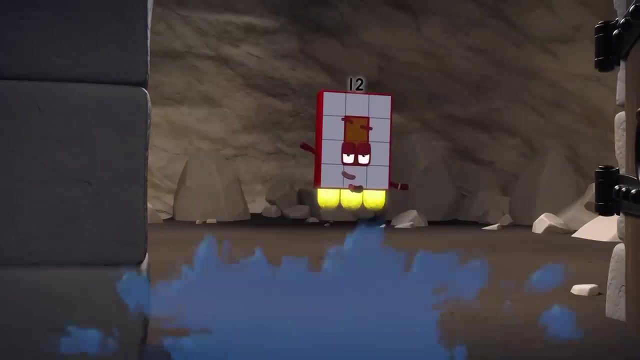 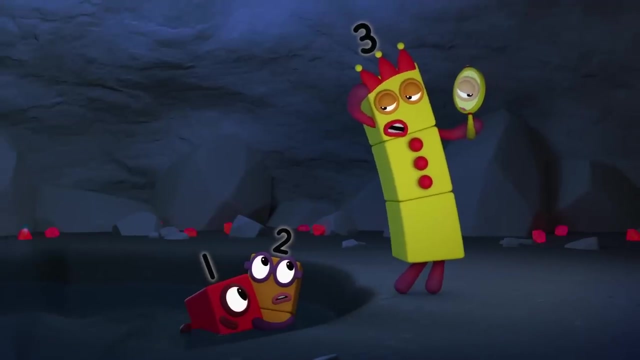 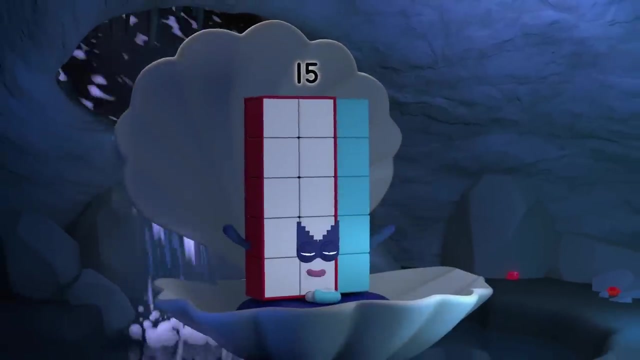 That's twelve gems altogether. That's right. Twelve gems shared between two bowls is six in each bowl. Congratulations, Ha, ha, ha, Ha, ha ha. Oh, There you are. I thought you'd never get here. I am the. 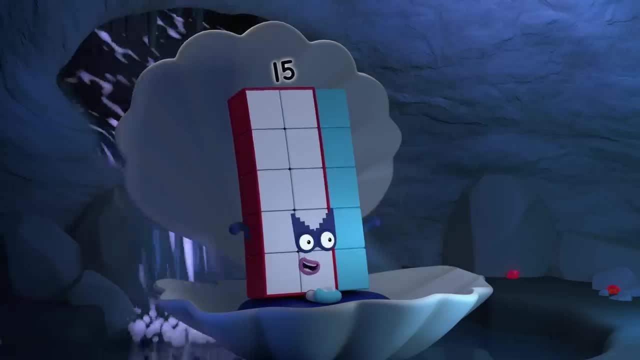 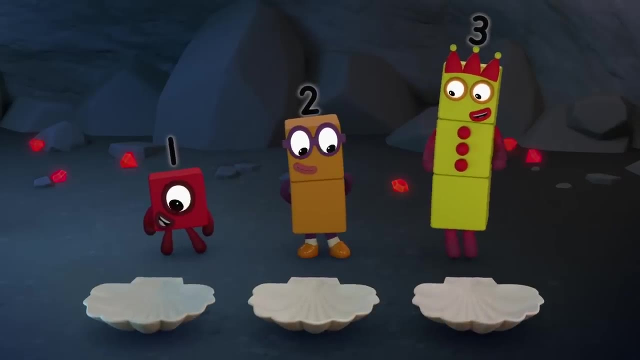 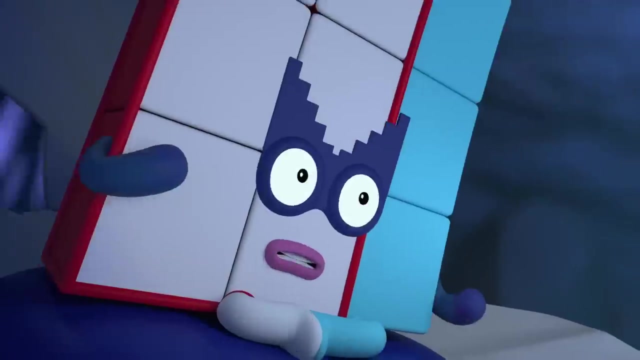 genie of water. Your next challenge is to share my fifteen watery gems between these three shells, So each shell has the same number of gems. Oh, The next key: Share the gems before the waters run dry or the key will be sucked. 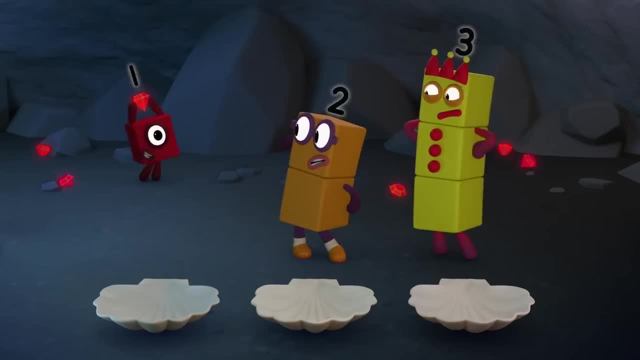 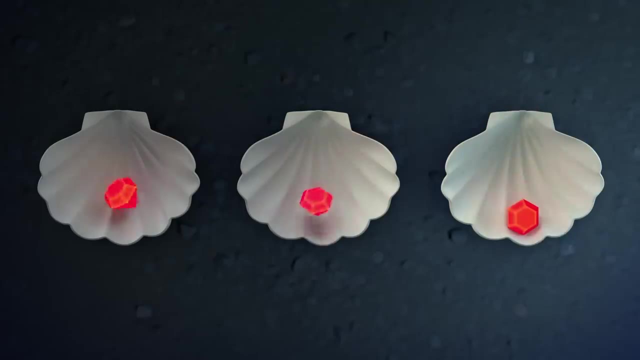 down the bottomless plug hole. Quick. One gem at a time. No, no, no, That's too slow, Let's get three at a time. Three shells, three gems. One gem in each shell. Good thinking, Three, Three shells. 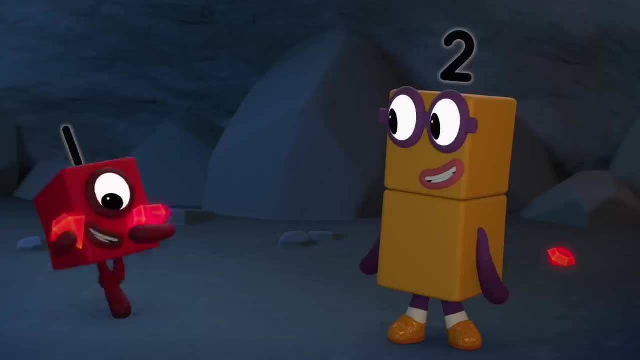 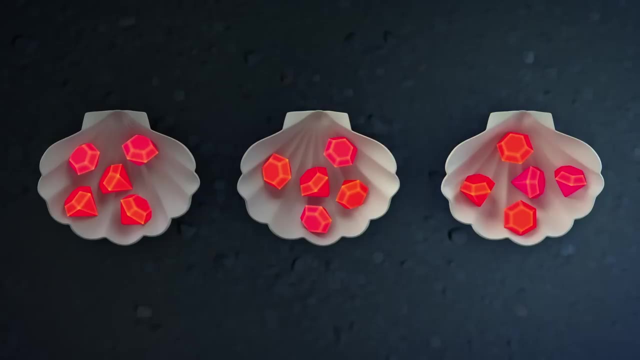 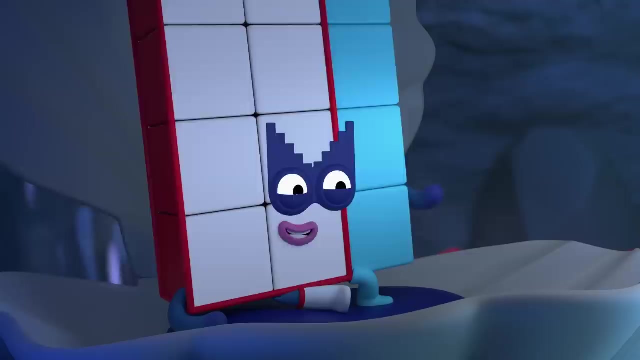 three gems, Two gems in each shell. Each time there's one more in each shell, Three more and three more, and that's all of them. Oh, Fifteen gems shared between three shells is five gems in each shell. Good sharing team. 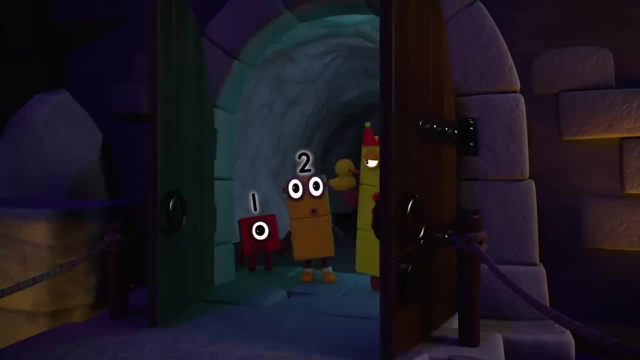 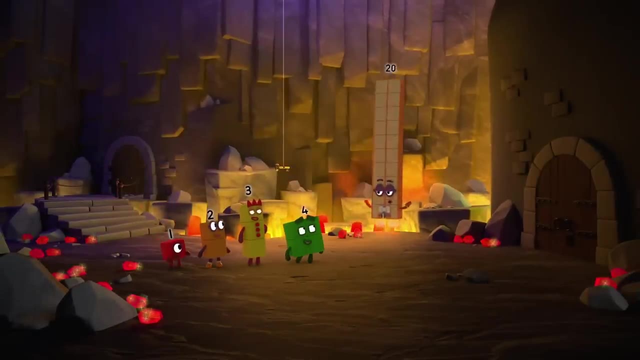 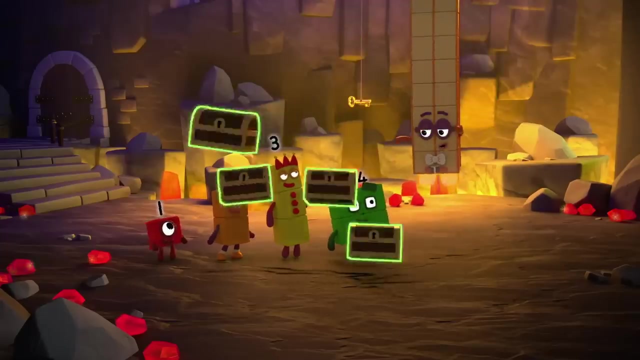 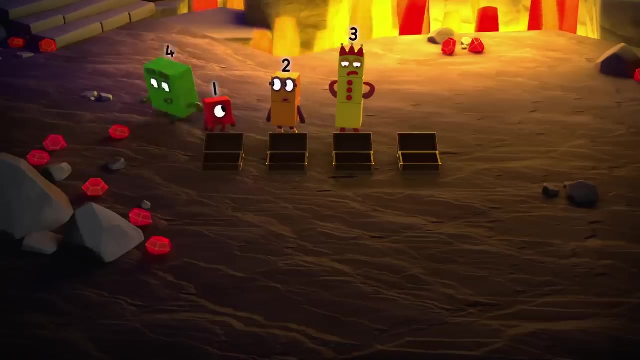 Ha ha ha. Oh, Hello, Nice and warm. here I am, the genie of fire. To win the final key, you must share my twenty fiery gems into these four chests You have untilmy toast is ready. Go, We need to make sure we find. 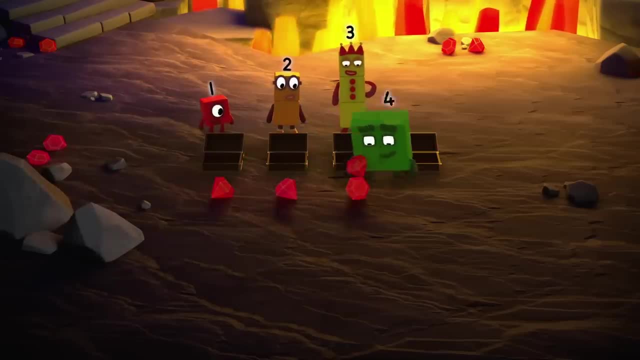 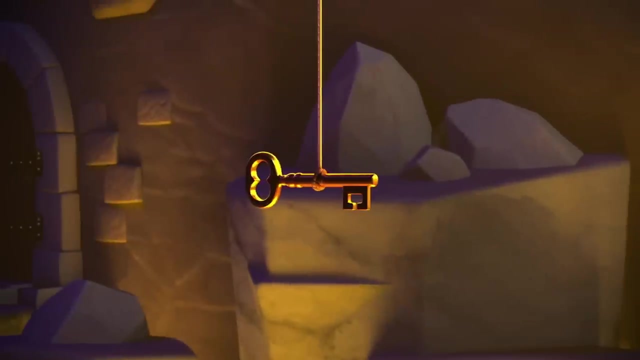 all twenty, so let's lay them on the ground as we go, Then we can check one for each chest. Now you put yours there. We need five rows of four to make twenty. My toast is nearly done and the key is nearly toast. 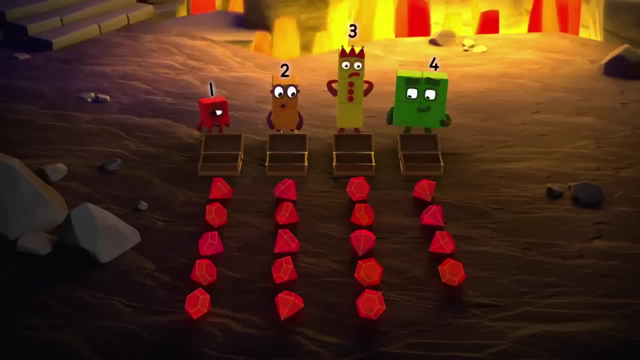 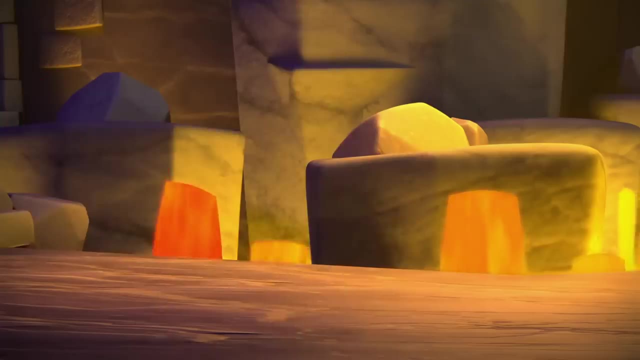 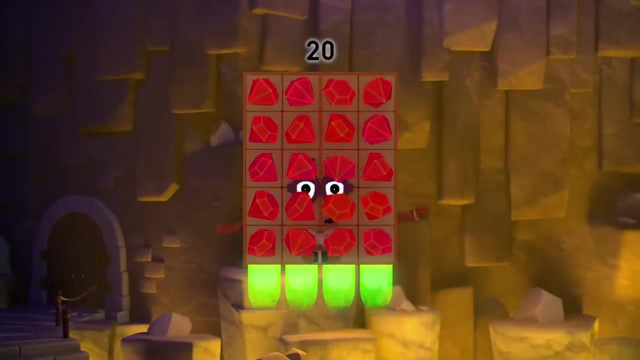 I can't see any more. Do we have them all? We can't have. Look, This line has one gem missing Here. Now all four lines are equal, That's right. Twenty gems shared equally between four chests is Four lots of five. 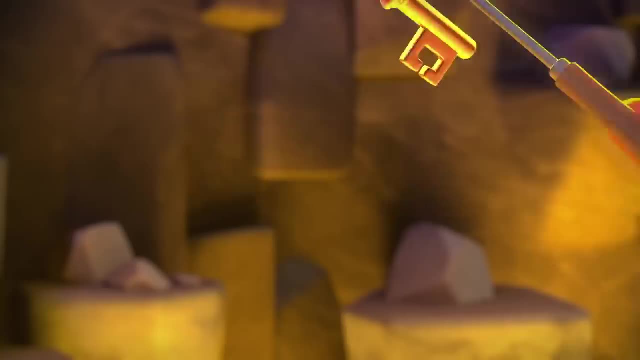 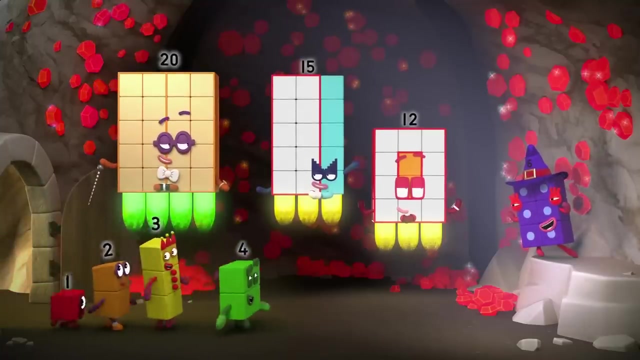 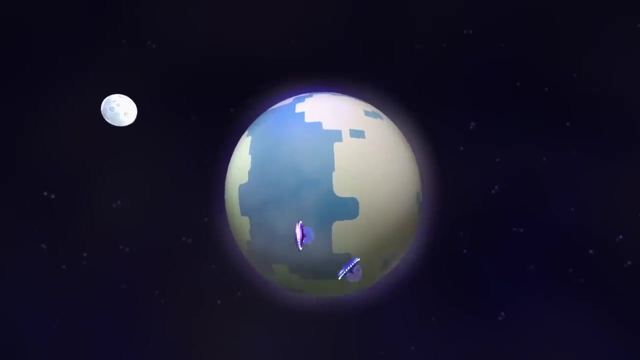 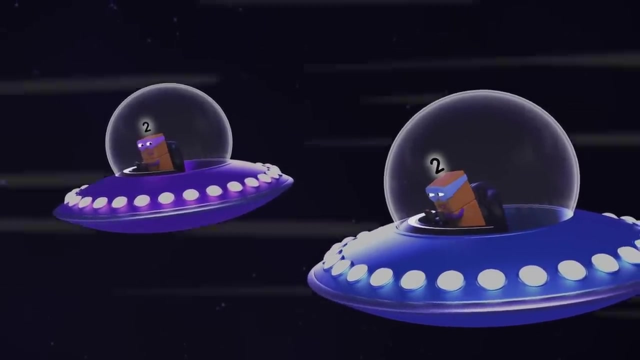 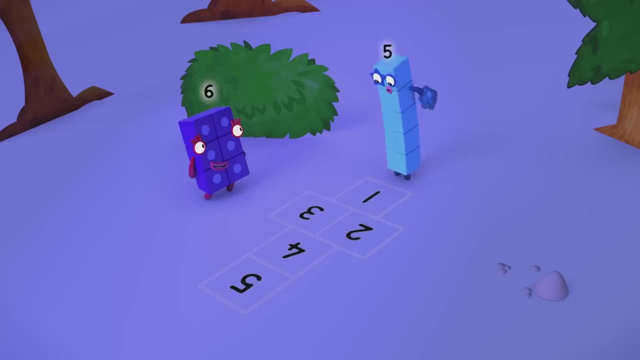 You've won the game. Gems of water, fire and air Enough for everyone to share. How many twos is too many twos, amigo? Let's find out with a game of How Many Twos- One, two, three, four, five. 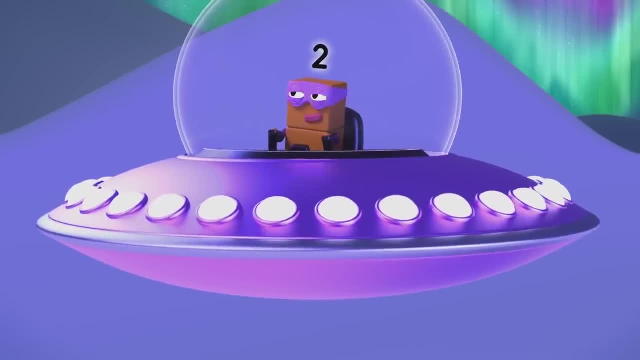 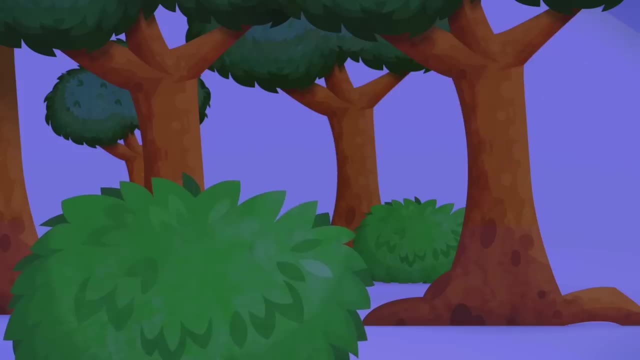 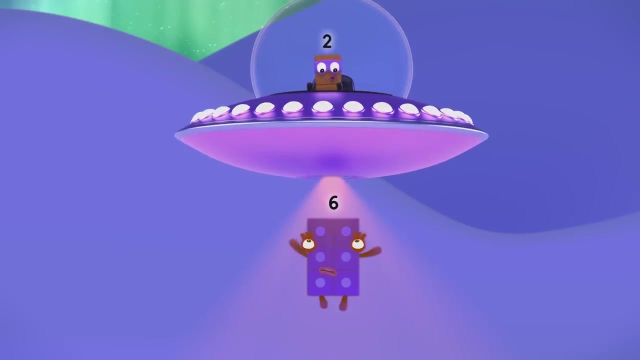 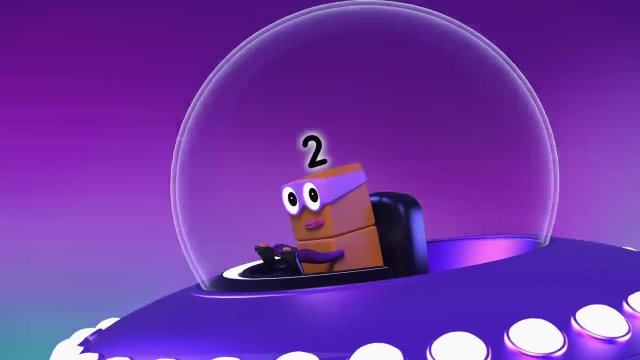 Back to being set Divide into twos. What a day, Yikes. Let's find out how many twos there are in six: One, two and three. There are three twos in six. Happy, Terrible Tuesday everyone. 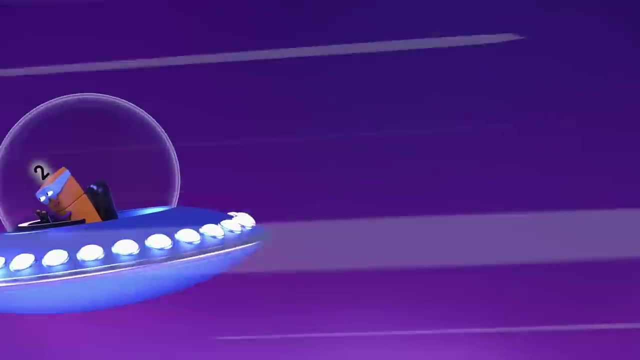 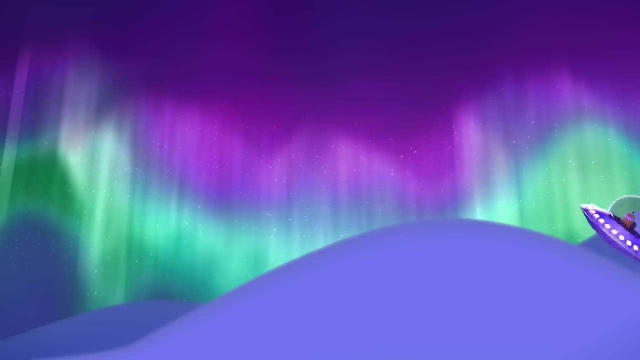 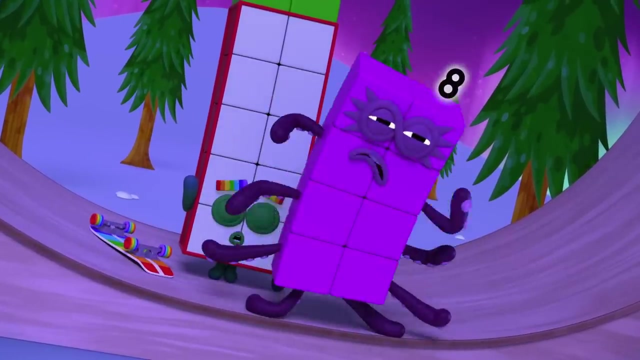 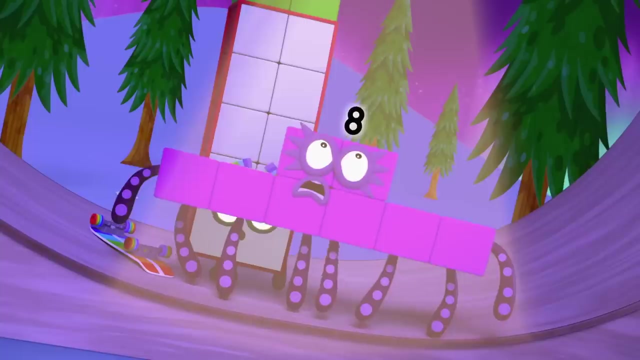 Or should that be every two? Whoa Target acquired Never fail Fourteen. I've dealt with the terrible twos before. Off to block shield. One, two, three, four, five, six, seven, eight, Yikes. 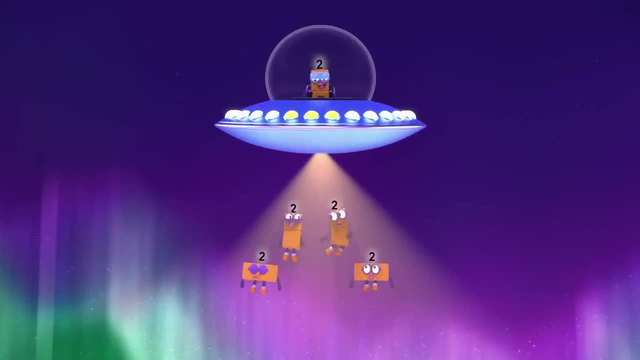 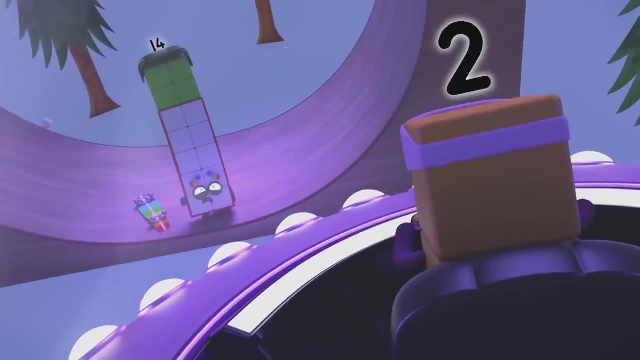 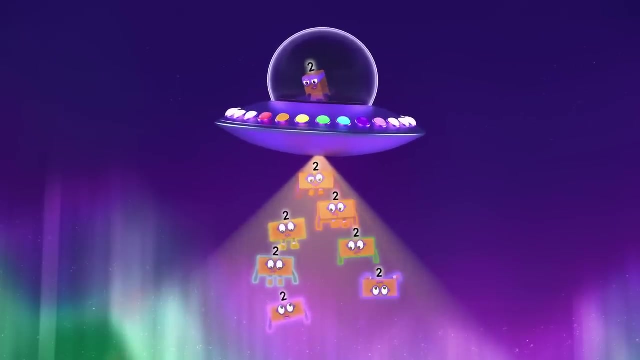 One, two, three, four. There are four twos in eight. You're in the lead, amigo, But not for long. One, two, three, four, five, six, seven. Pretty, There are seven twos in fourteen. Beat that. 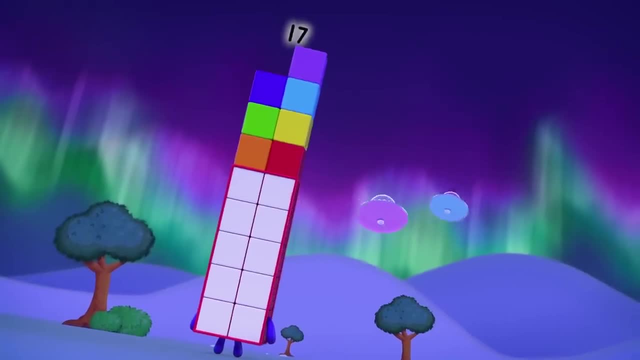 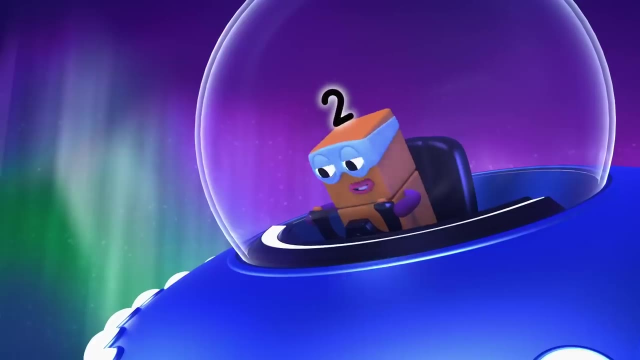 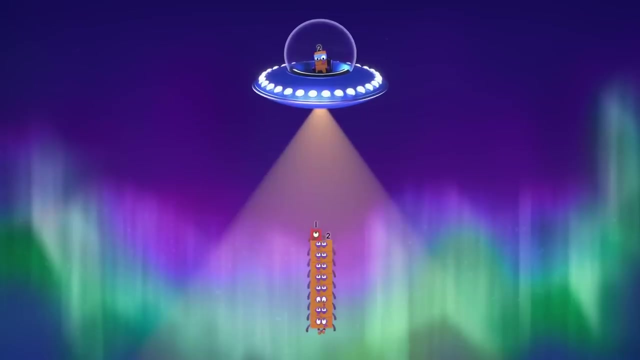 Excuse me, I need to lend a hand. Whoa Hold, still, Seventeen is greater than fourteen, So this should put me back in the lead. Whoa, Hey, Hey, Remainder alert, Remainder alert. There are eight twos. 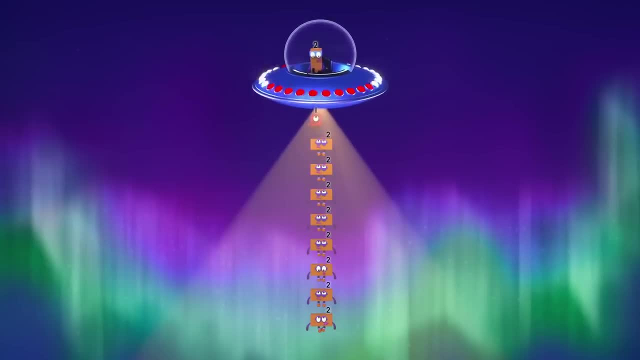 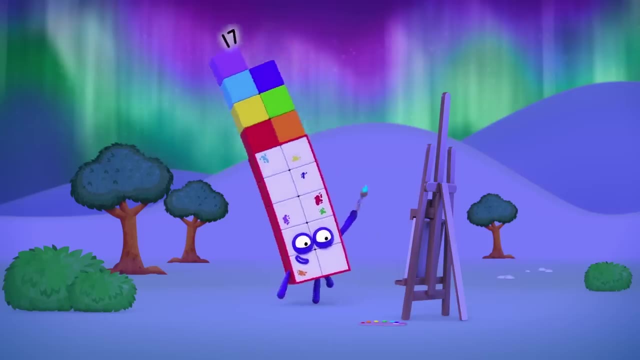 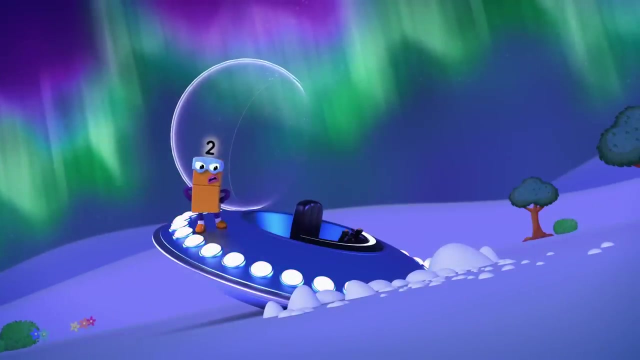 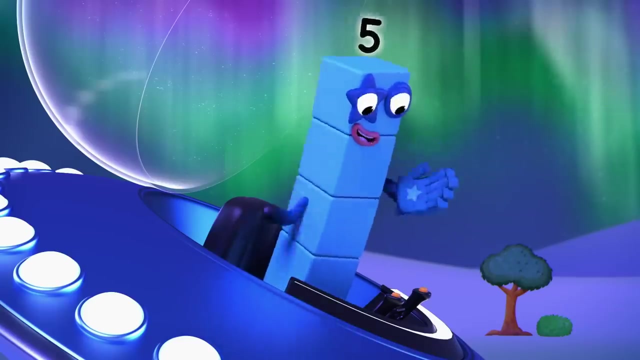 in seventeen and one left over. Remainder one. No Ten experience. I must paint it. Whoa, Whoa, Whoa. Where's that reset switch? Aha, You've gotta hand it to me, Whee Hey. 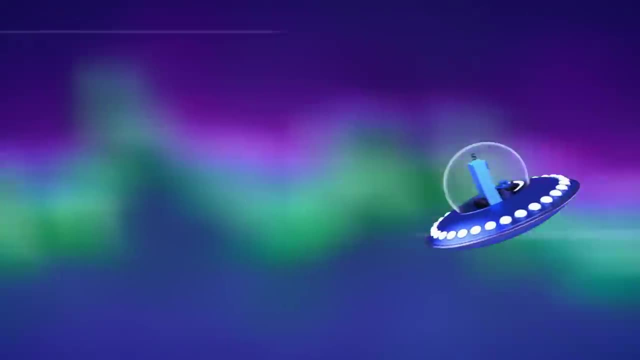 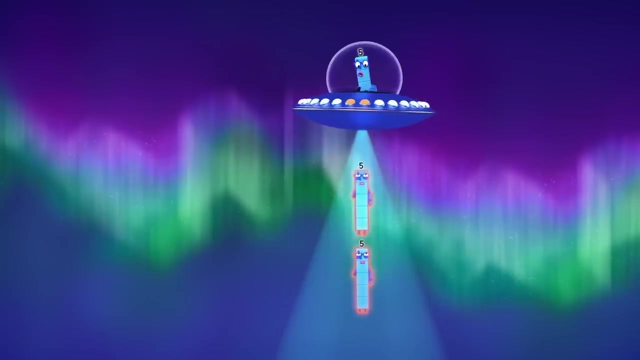 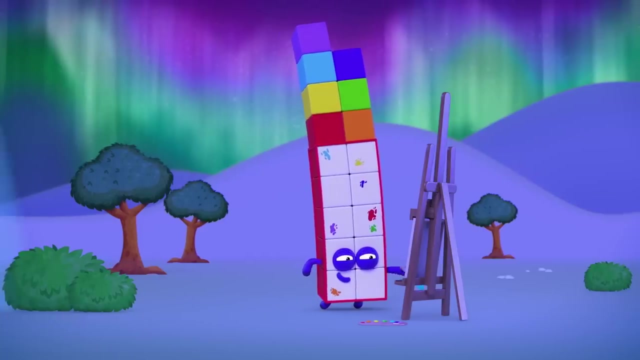 Factor beam reset. Divide into fives. Ha, You can't catch me. Oops, I've divided ten into two fives. Huh, Huh, Whoa, Sorry, Learn a driver. Remainder alert. Remainder alert. 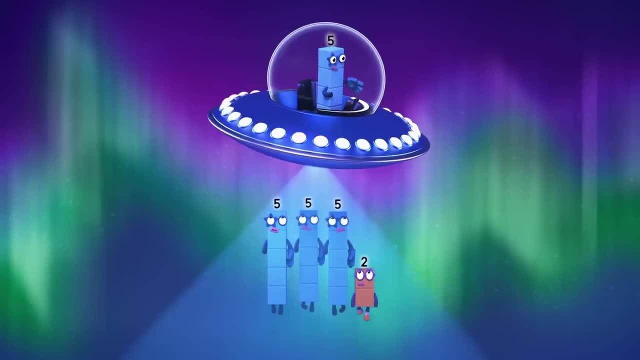 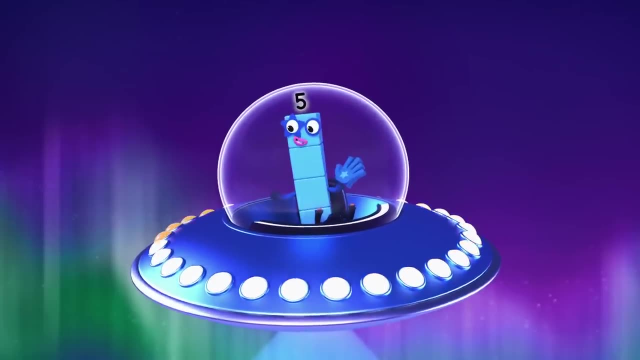 There are three fives in seventeen and two left over Remainder two. I think I've got the hang of it now. The twos factor beam divides you into twos and my factor beam divides you into fives Only if there are no blocks left. 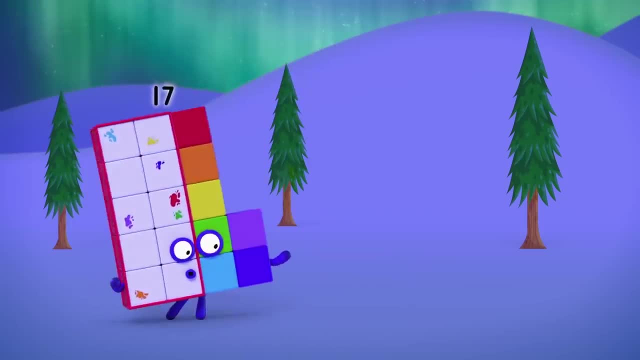 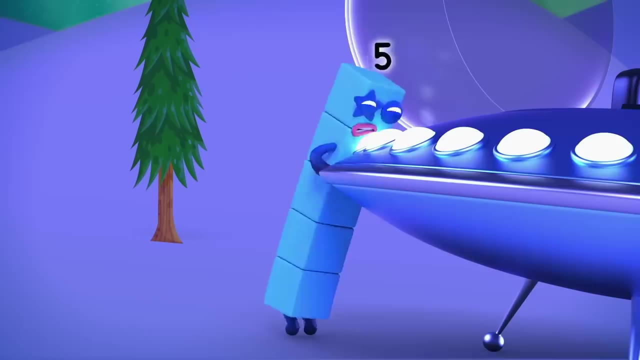 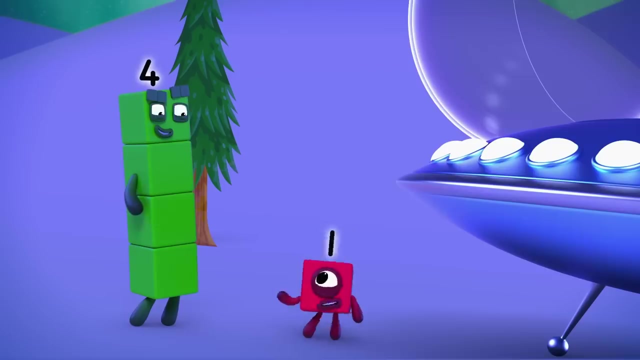 over. Whoa, Whoa, What. What can I say? There's just no divide in some people, Haha. I know how to stop the terrible twos And I know who can stop them. Mission accepted Factor beam reset. 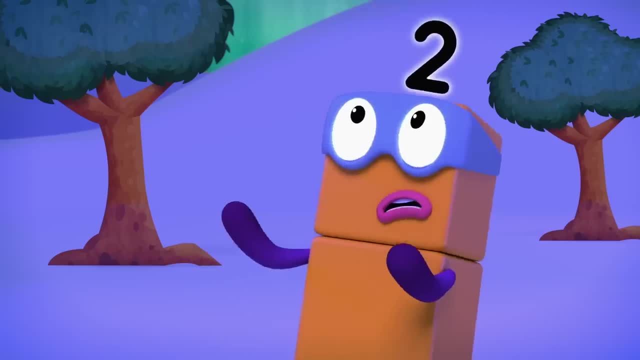 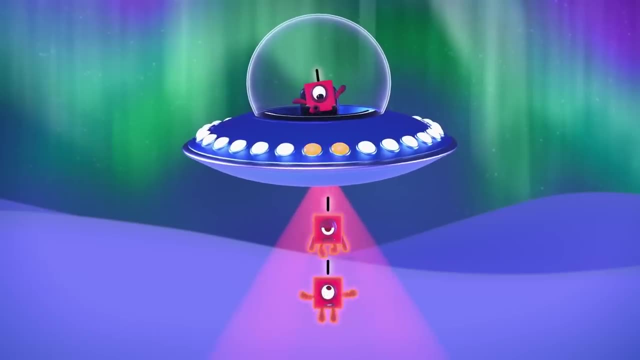 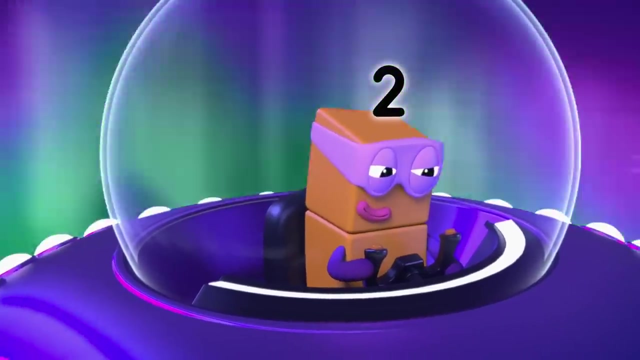 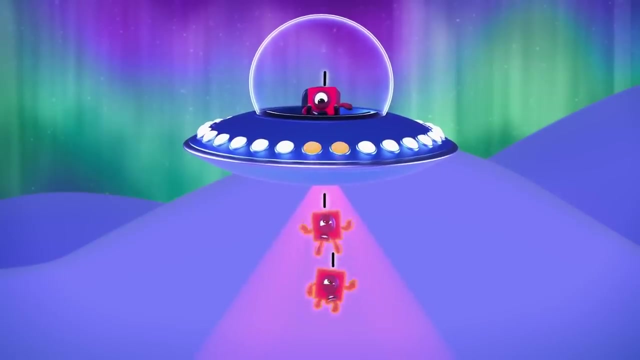 Divide into ones. Uh-oh, Oh Whoa. How many ones in two. Two, of course, Bah, Double, Bah, Whoa, Oh Whoa. Never any remainders when you split into ones. Bah, Well, well. 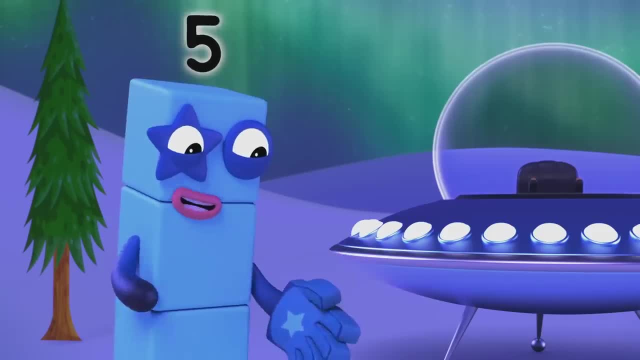 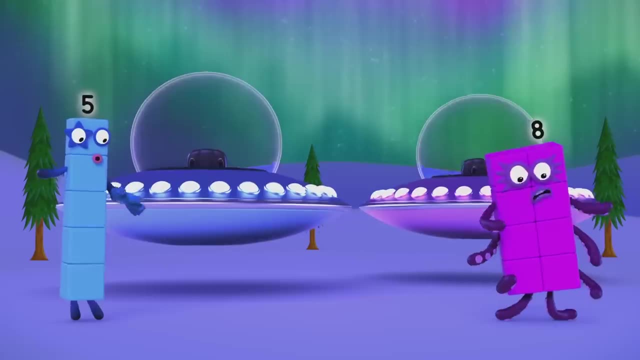 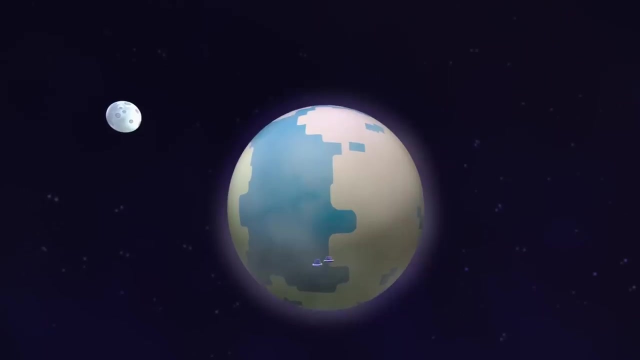 Aren't you the naughty ones? Haha, Don't worry, The factor beam wears off in time. Well, I don't think we'll be having any more trouble from Wait, Where have they gone? Watch the skies, Whee. 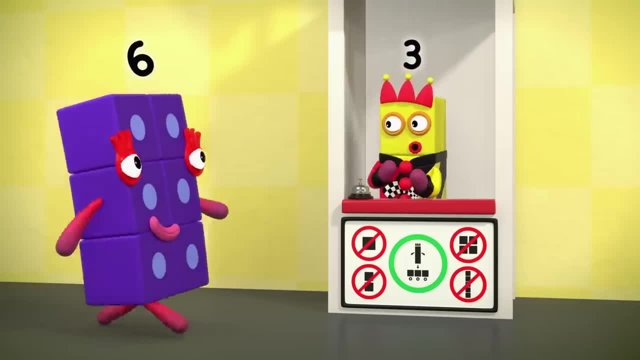 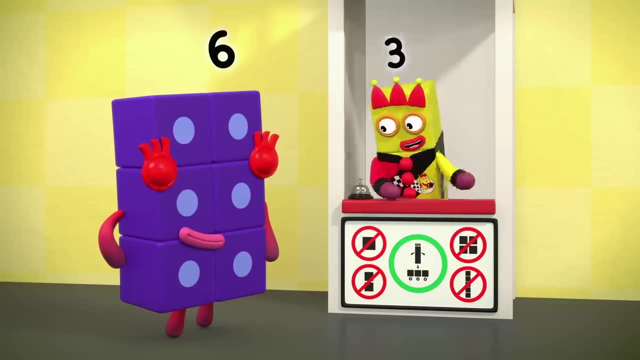 Welcome to my divide and drive go-kart track. How many karts do you need? What do you mean? how many? Isn't one enough? No, no, no, Only threes can fit into my go-karts, so you'll need to divide. 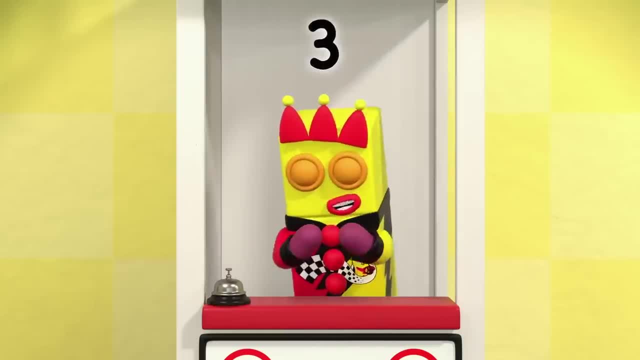 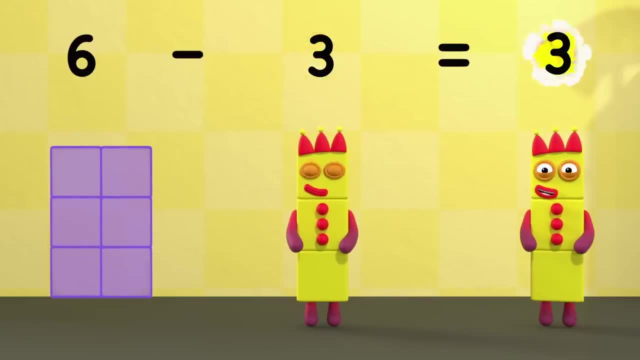 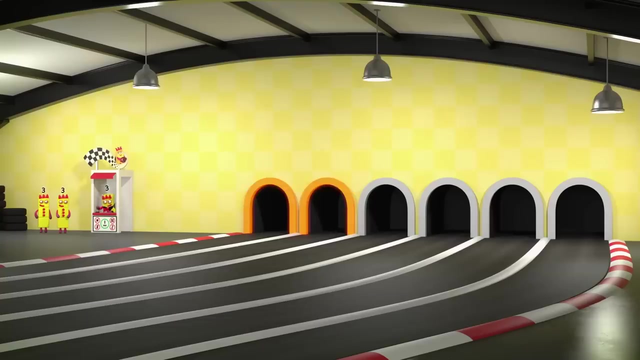 into threes before you can drive. Divide and drive, Take off three and we'll see what's left. Six minus three equals three. There you go. There are two threes in six, so you need two karts Off you go. 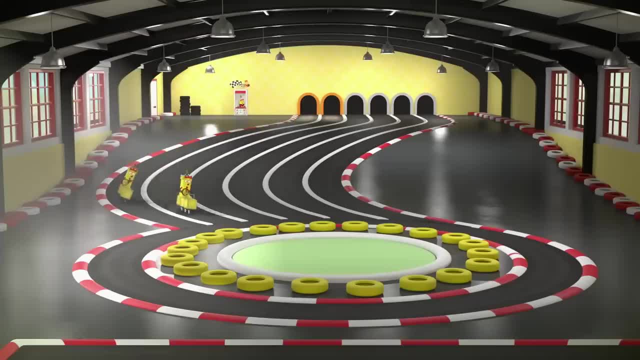 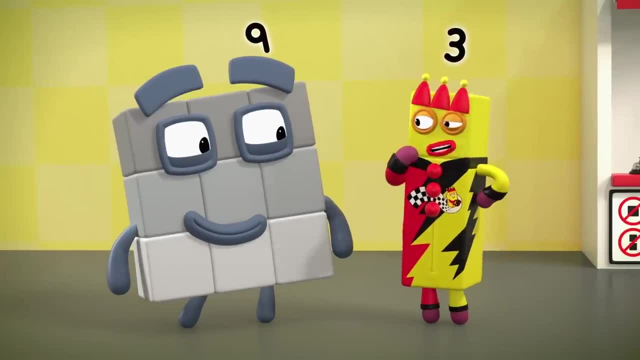 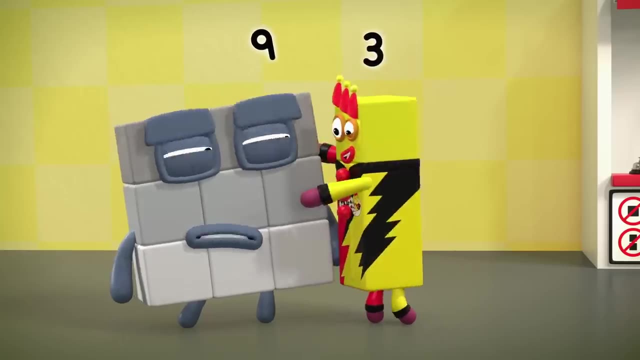 Oh, Whee, Yikes, Lots of customers. Nine: How many karts do you need? How many threes in nine? Leave it to me. I'm good with threes. Let's take a three off. Nine Minus three equals. 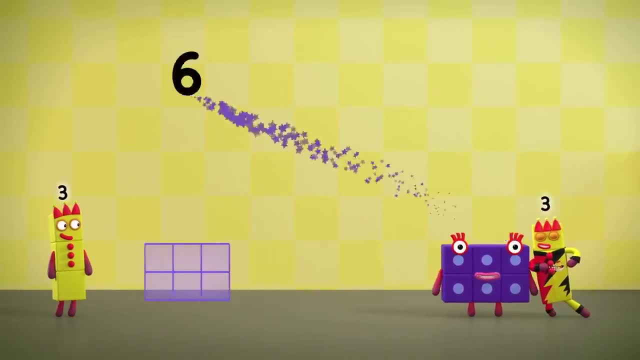 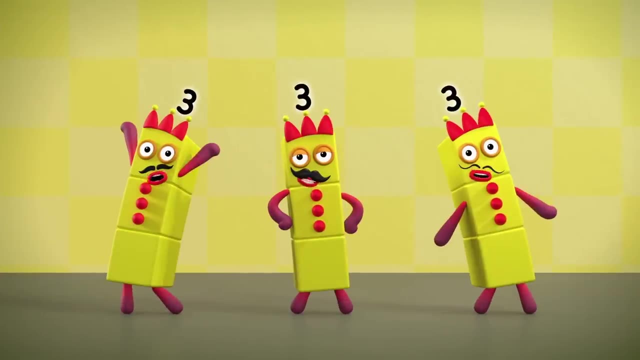 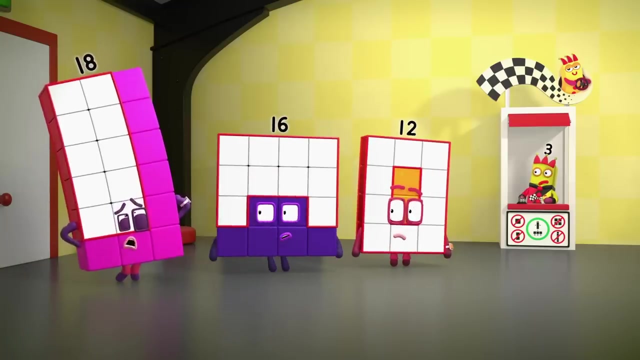 six And again. Six Minus three equals three. Hey, One, two, three, The three threes. Yes, yes, yes, Oh, Can you please move faster? Some of us can't wait to go, go, go-kart. 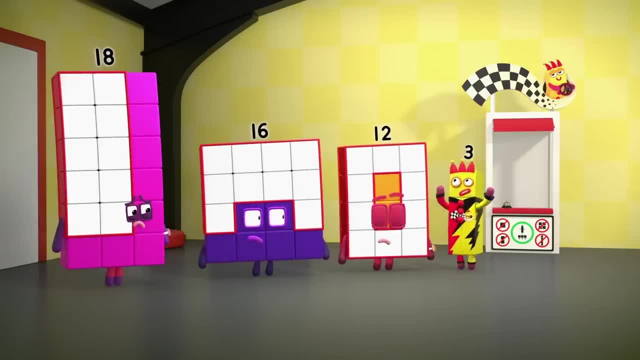 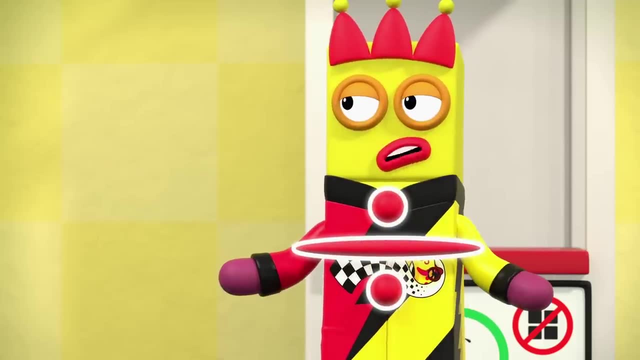 Hey, hey, hey, I'm going as fast as I can. you know, Subtracting threes one by one is a slow business. I mean, if you know a faster way of dividing into threes, you tell me Time. 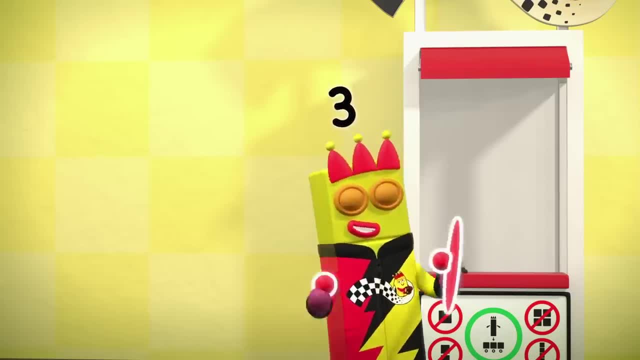 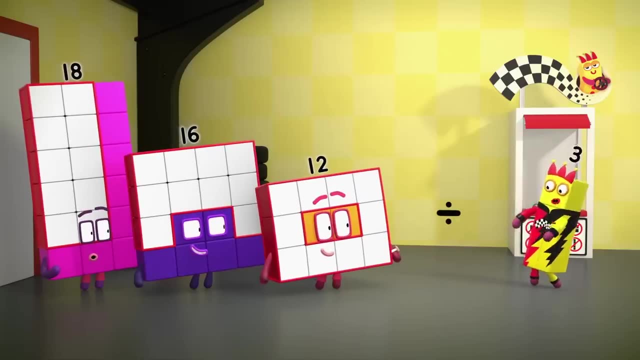 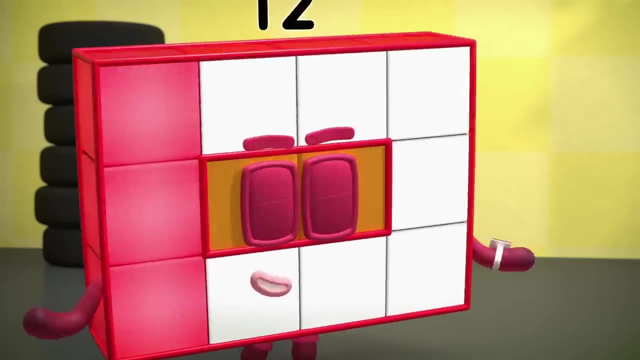 Oh, I know Juggling helps me think. Oh, It's a sign, A new sign. Maybe this can help me divide you up faster. Let's see, Look, Can't you see? I'm keen to try something new Instead of taking 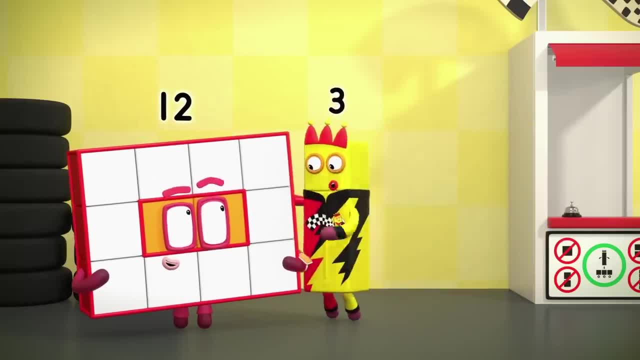 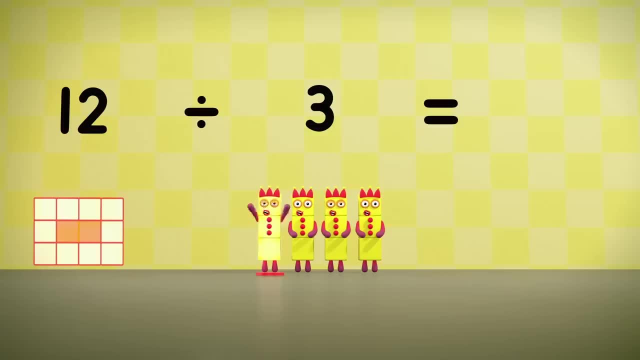 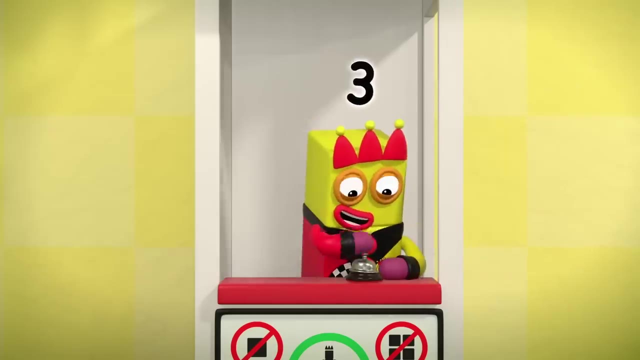 threes away over and over. let's divide you into threes all at once. Twelve divided into threes equals one, two, three, Four. There are four threes in twelve. Woo-hoo Whee, I can divide anyone like. 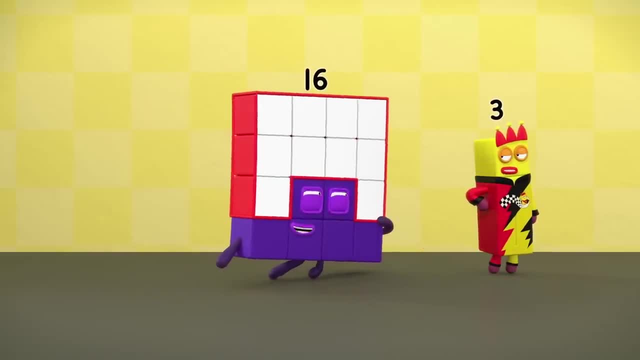 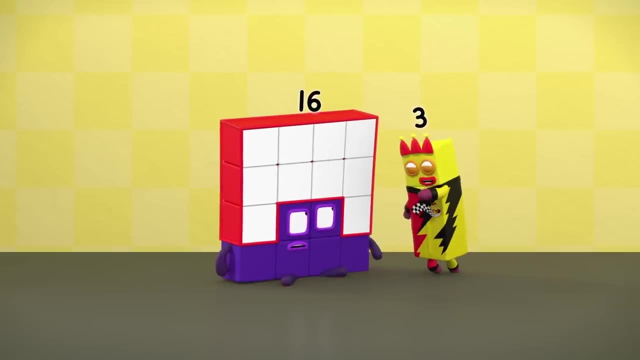 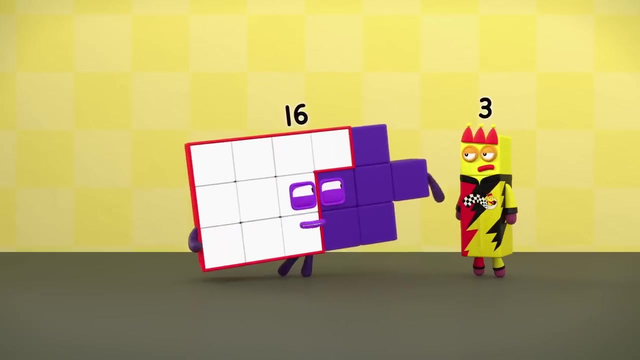 this Anyone. you say Why I'm anyone Give it a go. Sixteen, No, no, no. You need to make a rectangle that's three blocks high, like twelve did. Nope, Not gonna happen. Got this one block. 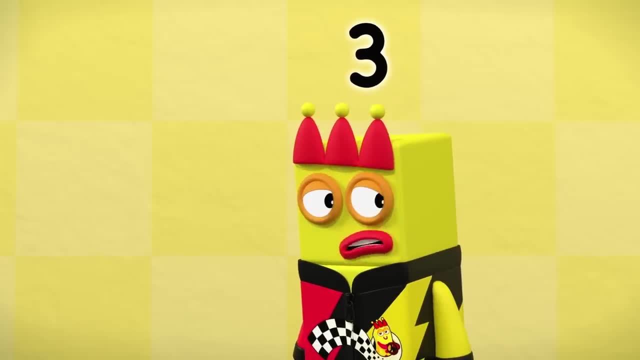 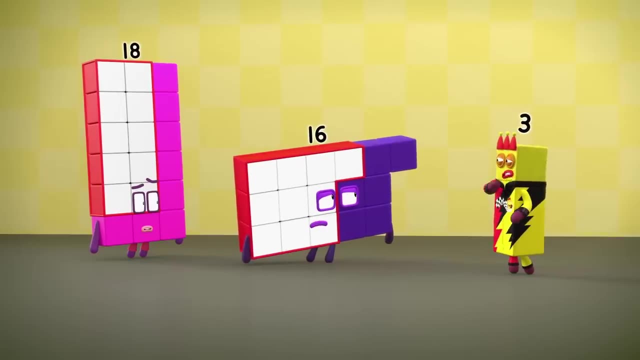 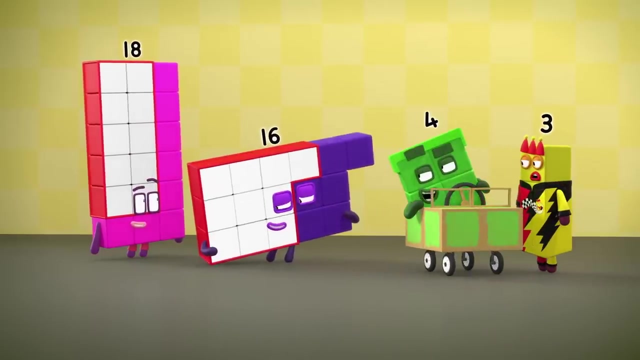 remaining on the end. I guess I can't divide you into threes without leaving some of your blocks behind. Sorry, sixteen, but you won't fit in my go-karts. Oh, Excuse me Coming through. Who wants to go on my go-kart track? 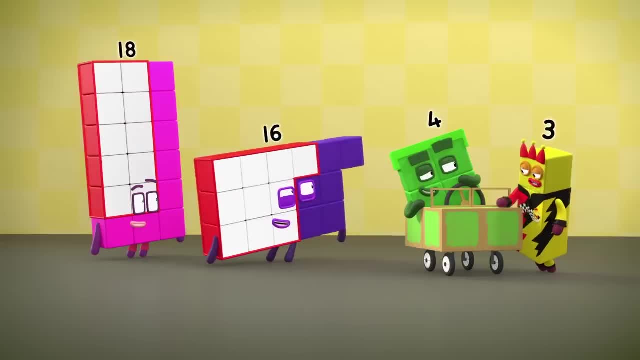 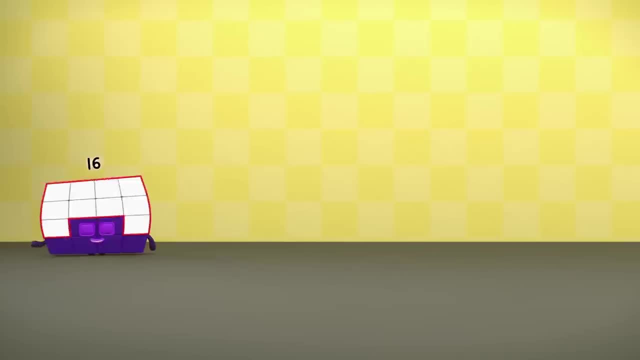 For four-wheel drivers. Ooh, Can I try? Sorry, three. Only fours can drive my karts. Oh, Maybe I can. Sixteen Divided into fours equals one, two, three, four. The four fours, Oh yeah. 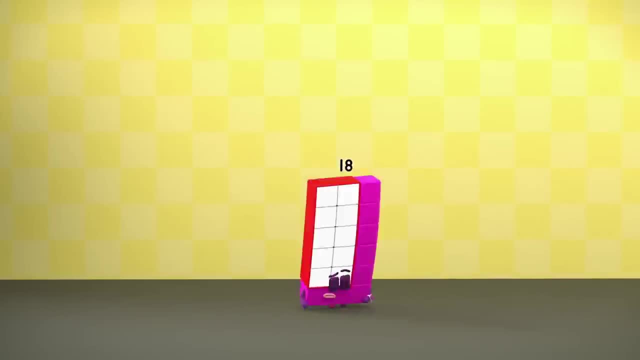 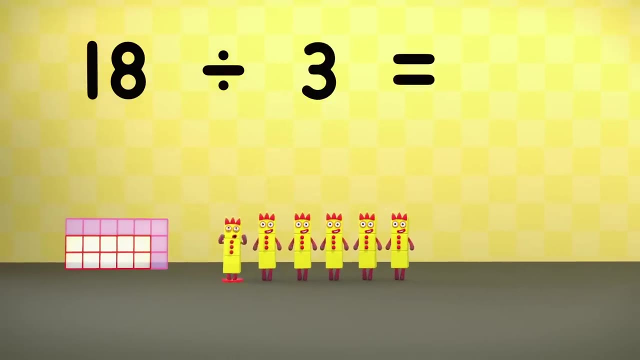 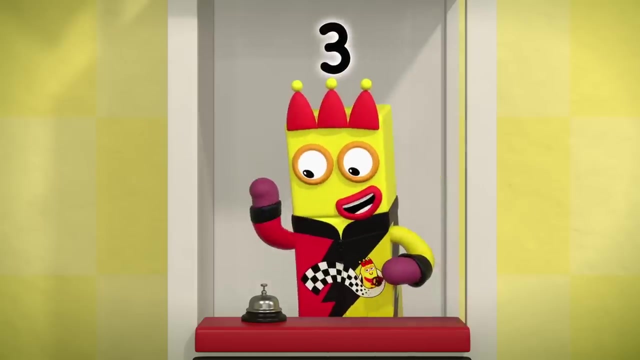 Woo-hoo, Literally unable to wait a moment longer. Eighteen Divided into threes equals one, two, three, four, five, six. All right, Yeah, Six times three equals Eighteen. Oh, what do you know? 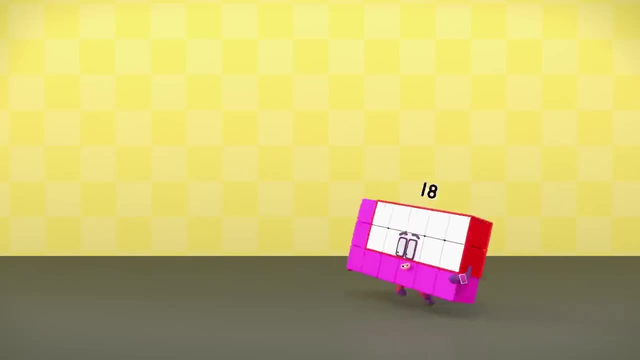 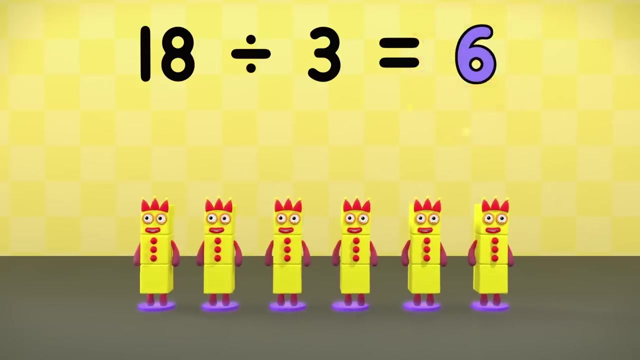 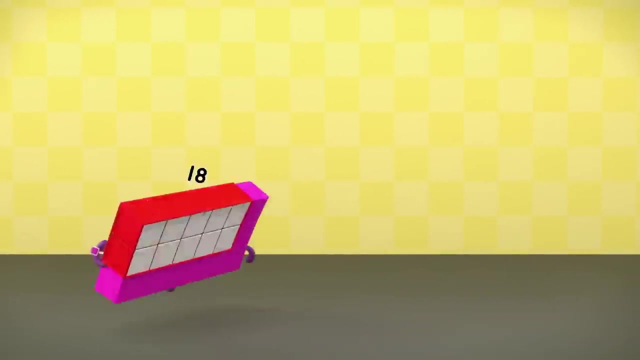 Division is the opposite of multiplication. Here I go again. Eighteen Divided into threes equals six. Six times three equals Eighteen. I could do this all day, So I will. Eighteen Divided into threes equals six. 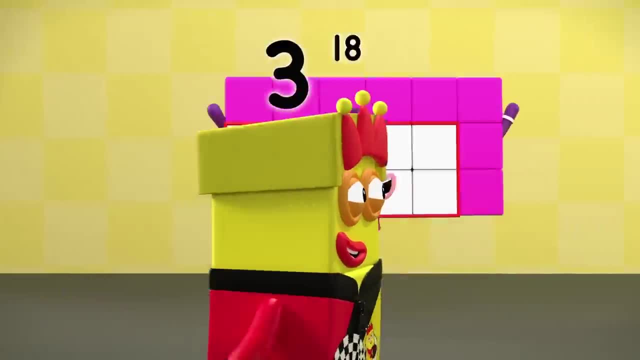 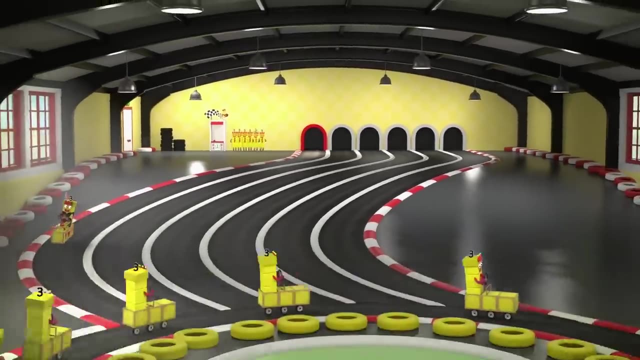 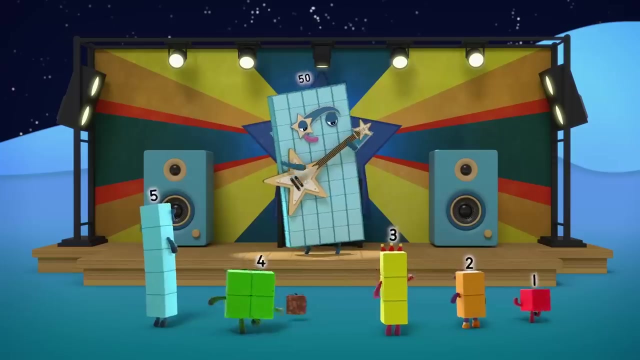 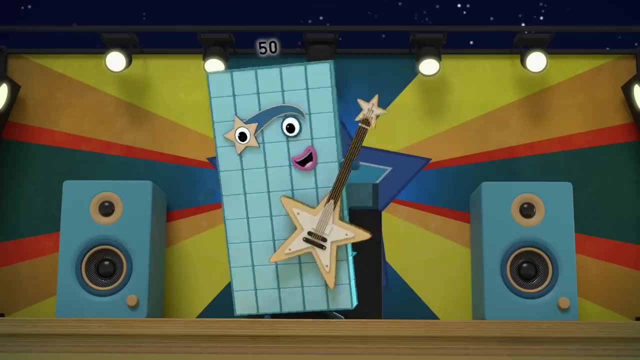 Some numbers are just born to show off. Six times three equals. Eighteen Divided into threes equals. Look at me. Fifty's so big, Squarey, Ten times thicker than me. That's right, I'm ten-fives. 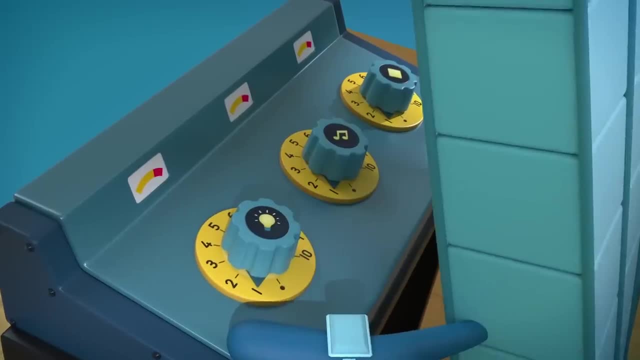 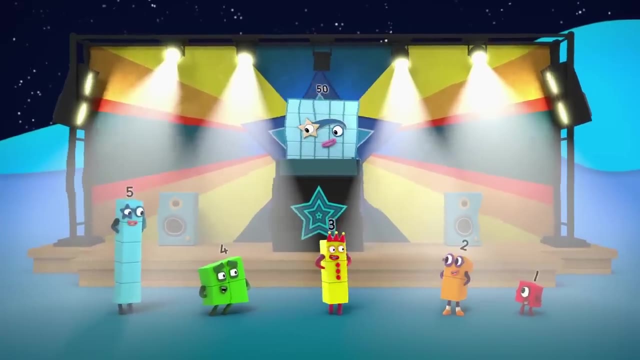 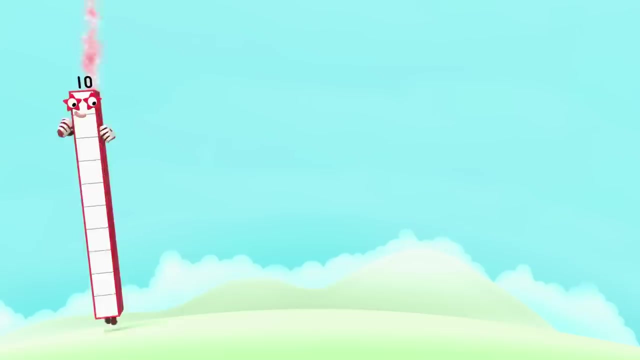 Rock and roll. These controls can make anything ten times bigger: The lights, The sound. Number blocks. Number blocks Ten, twenty, thirty, forty, fifty Number blocks Ten, twenty, thirty, forty, fifty Number blocks. And another ten is. 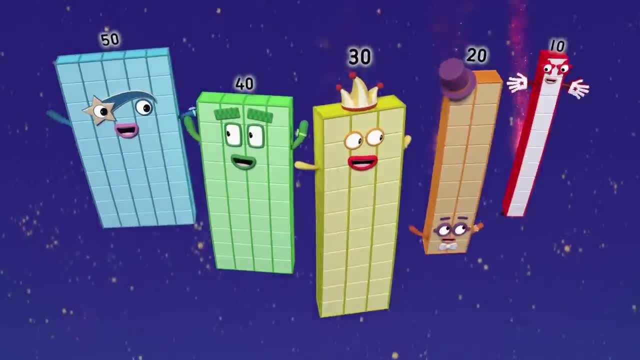 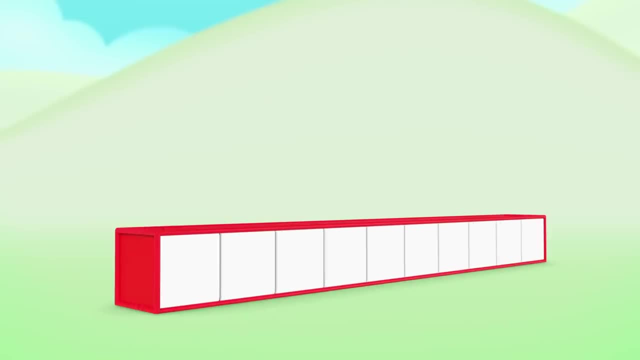 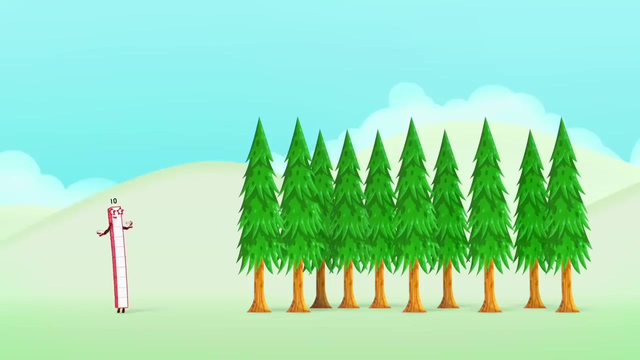 me at thirty, Fifty, forty, thirty, twenty, ten Number blocks. start again Ten. I am ten, One, ten and nothing more. Ten, Ten trees, Hello trees, Oh Ten birds, Hello birds, Ooh Ten brackets. 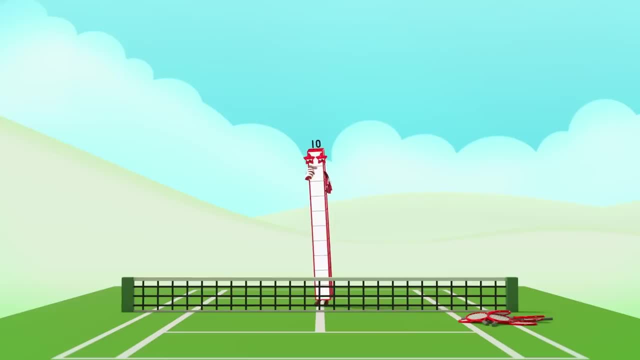 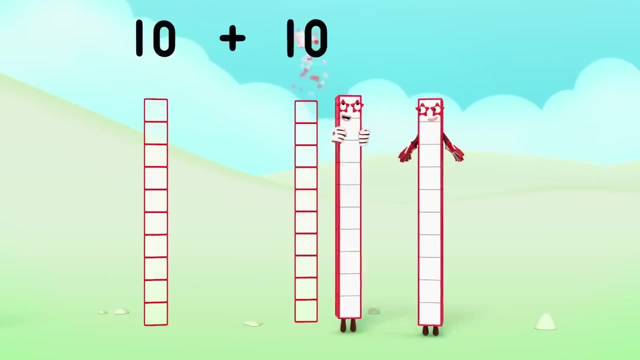 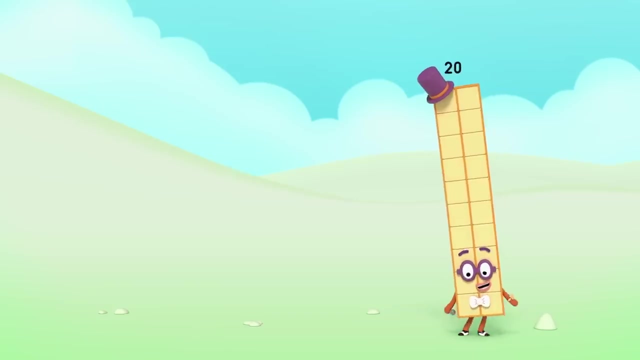 Anyone feel ten-ish? Oh, I need to make friends. Ten plus ten equals Twenty. Pleased to meet. Oh, I know, Ten plus ten equals Ten plus ten. Hee, hee, hee, Oh, Hahaha. 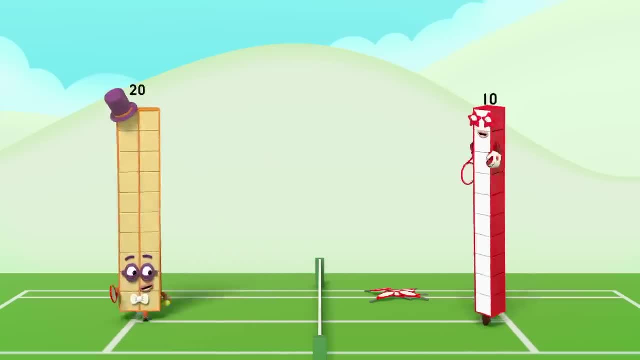 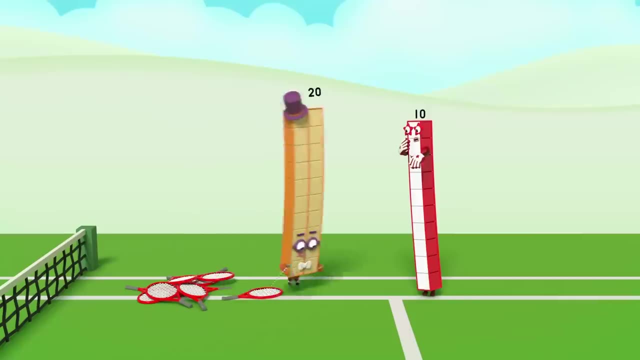 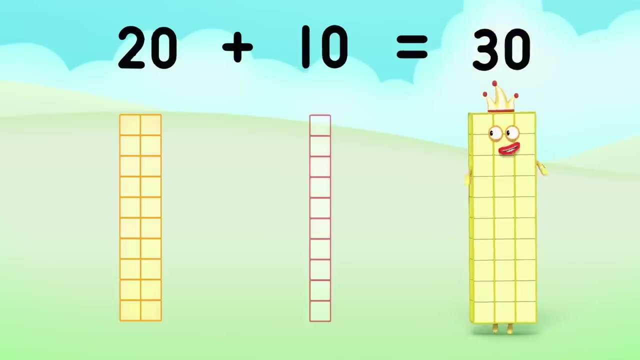 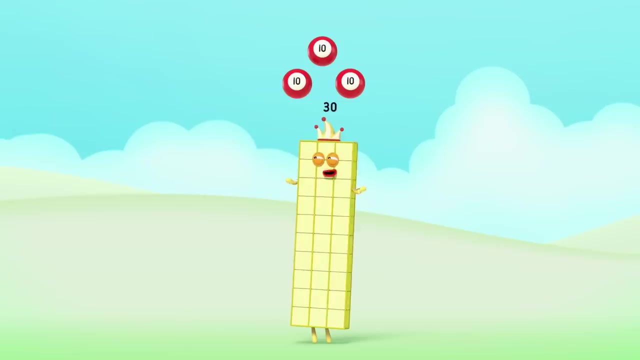 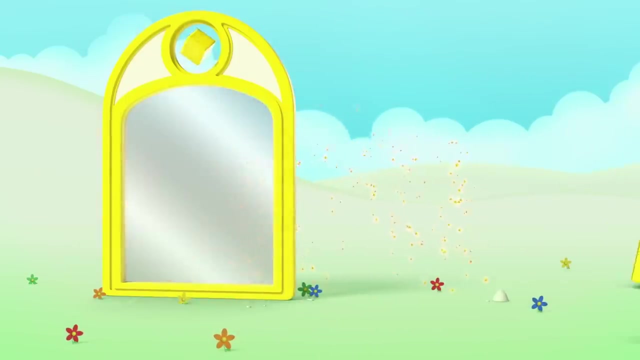 Oh, Hello, there, Let's play. Oops, Ten times too hard. Come back ball. Twenty plus ten equals Twenty plus ten equals Thirty. Ten, Twenty, Thirty. Hmm, No show without an audience. Oh, Hahaha. 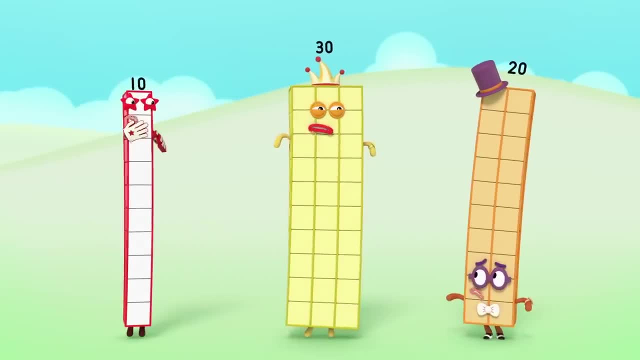 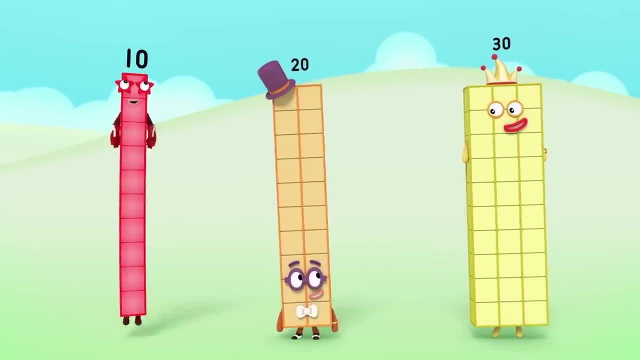 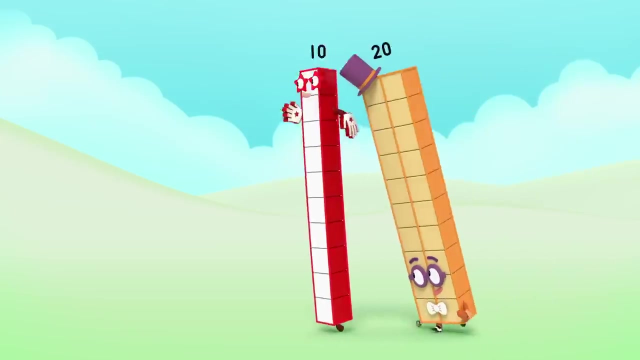 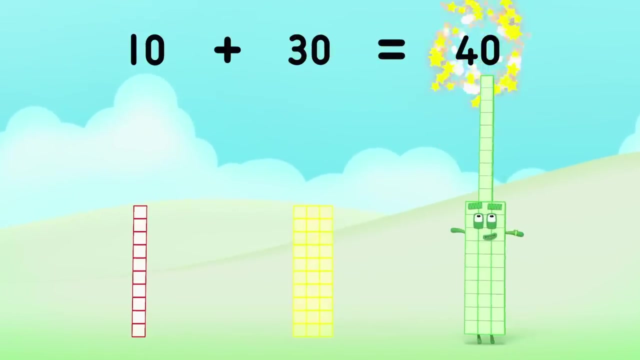 Ten, Thirty, Twenty, That doesn't sound right. I'm bigger than you. I'm smaller than you. Thirty, I'm the biggest number. Nobody's bigger than me. Huh Huh. Ten plus thirty equals Forty. 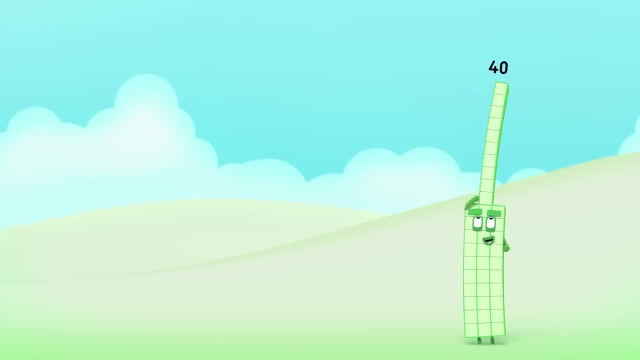 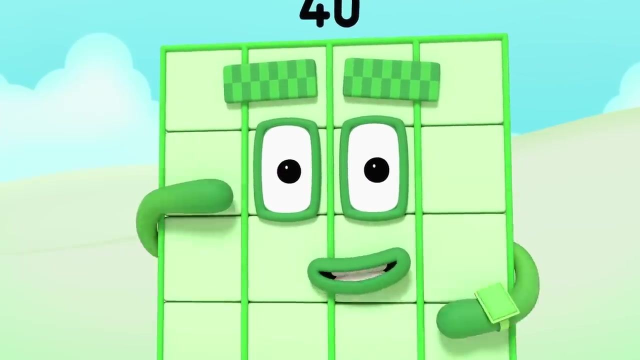 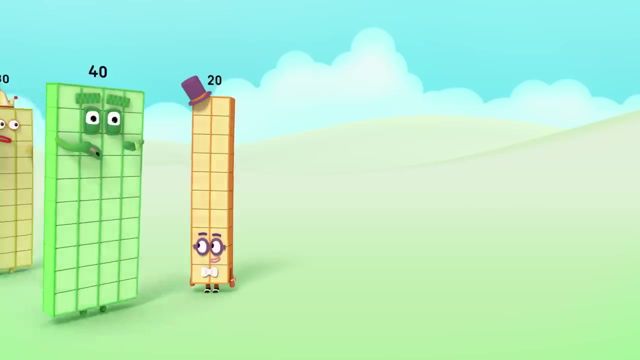 I'm forty. Ooh, I'm sticking out a bit on top. Ah, That feels better. I love rectangles. Would you like to meet my pet rectangle? Oblongy, Oblongy, Oblongy, Oblongy. 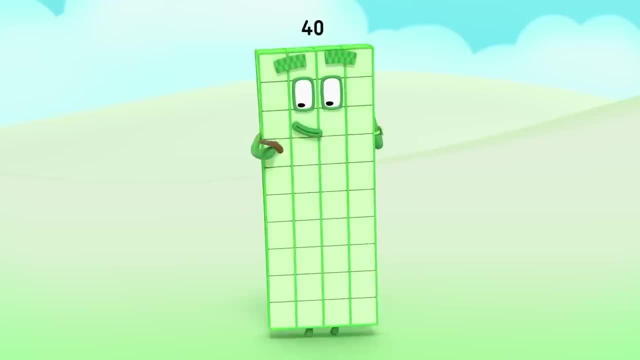 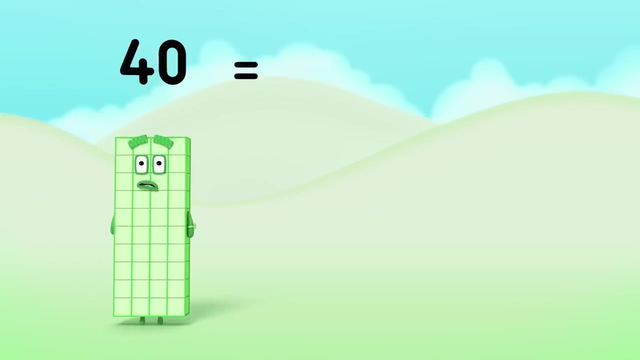 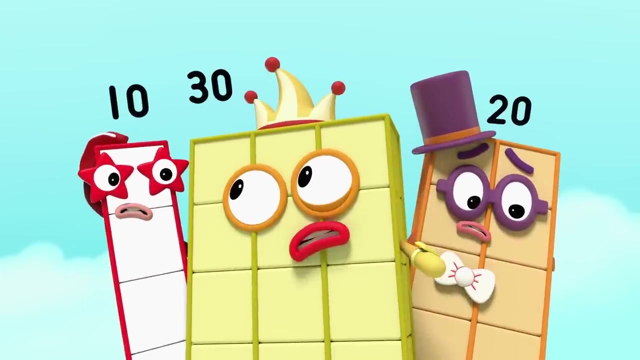 Oh, Hahaha, Huh. Where did Oblongy go? Left or right? I can't go both ways, But we can. Oh no, Not you too. Forty equals Twenty plus twenty, The terrible twenty, Jeez. 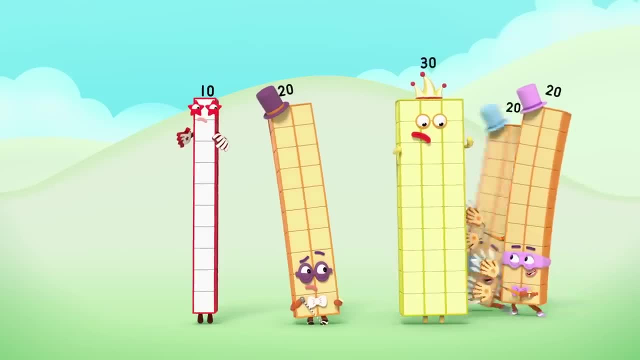 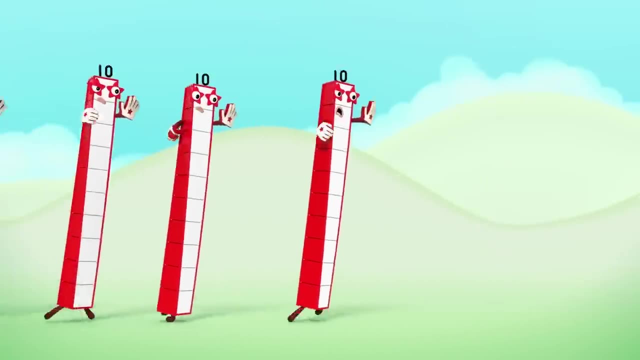 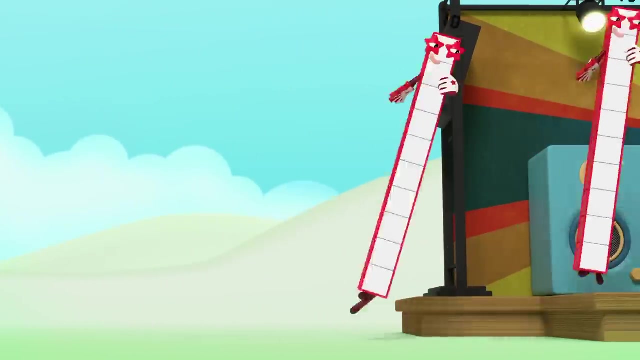 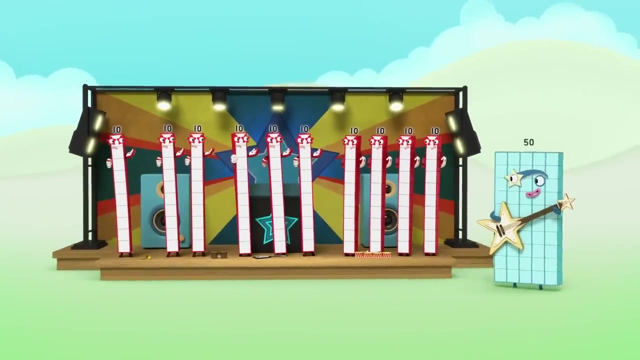 Two lots of twenty feathers. It's tickling time, Tickle, tickle, Haha, Hey, Come back here, Hey you, Uh oh, Time for us to split. Huh, Huh, Huh, I'm fifty. 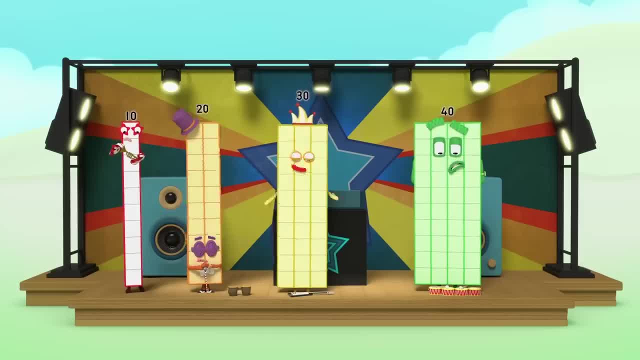 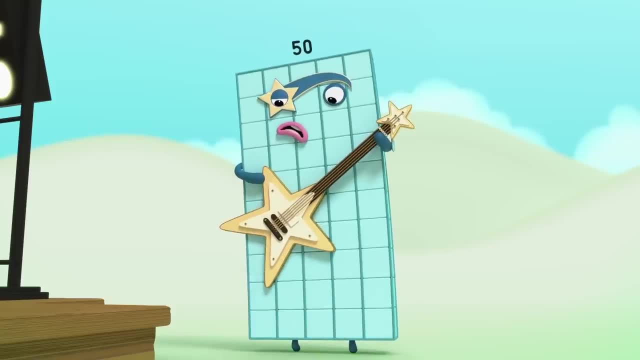 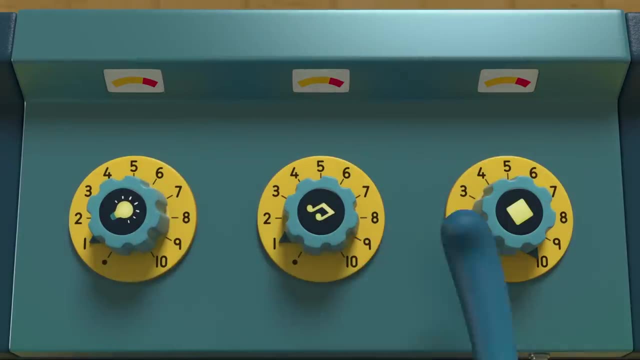 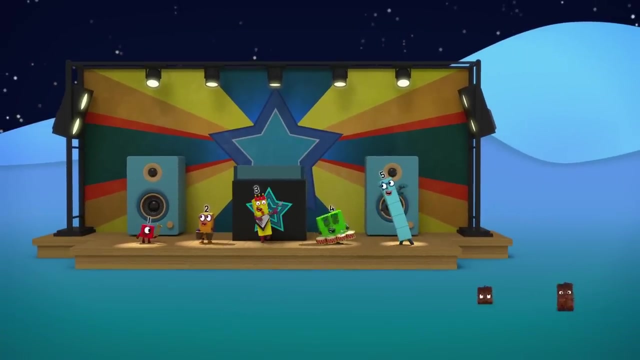 Let's split back together. Huh, Uh, oh, Whoa, Woohoo. Hey, You turned everything up to ten, That's more like it. Five, four, three, two, one Time for some number fun. You can count on us. 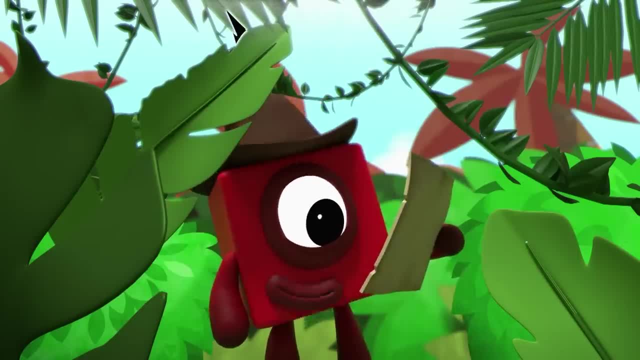 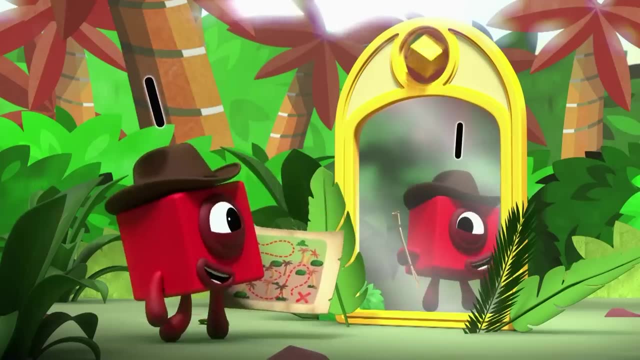 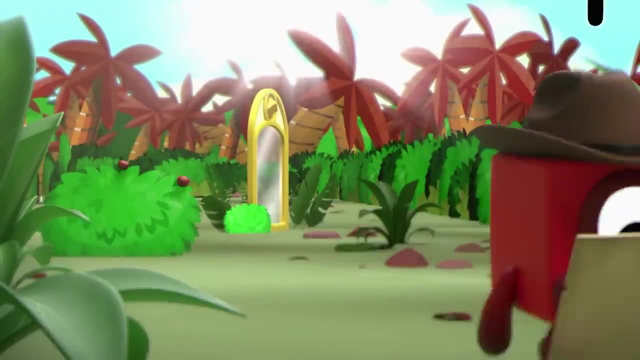 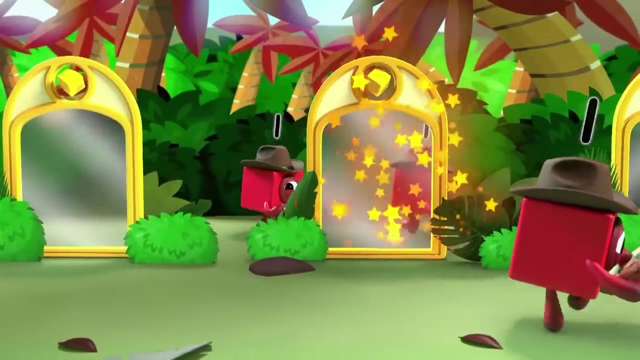 We're the number belts. Hmm, X marks the spot, But where is? Ah, Only my reflection. Hello me, Haha, Huh, Haha, Haha, Haha, Haha, That's it. X marks the spot. 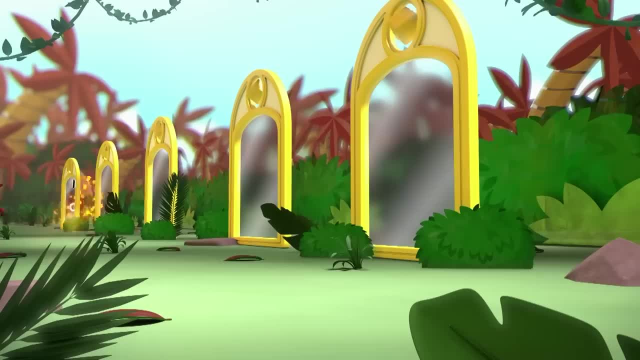 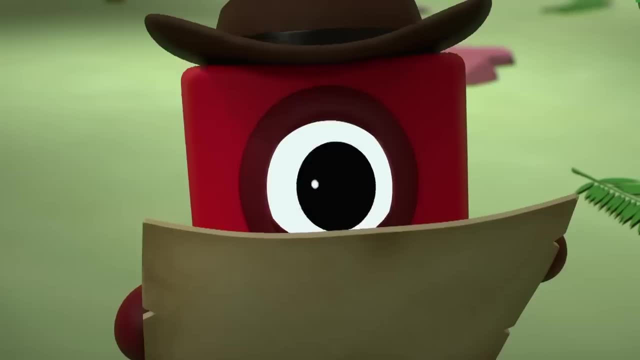 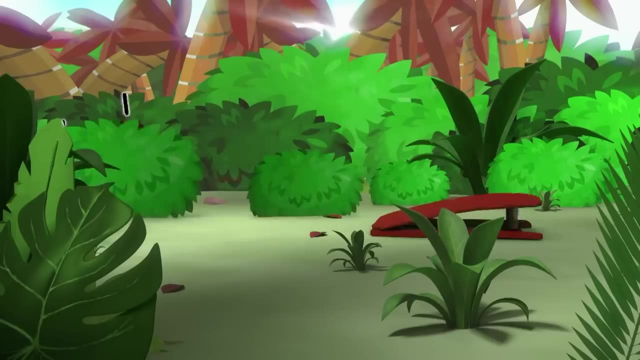 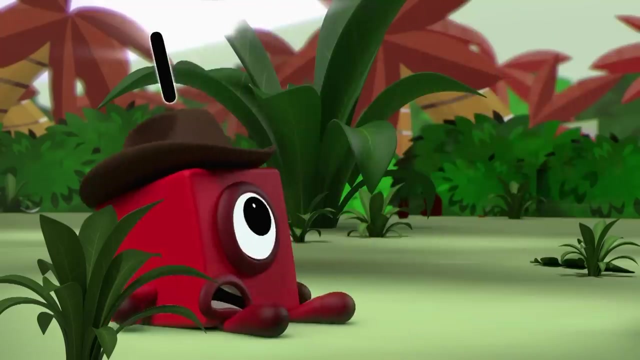 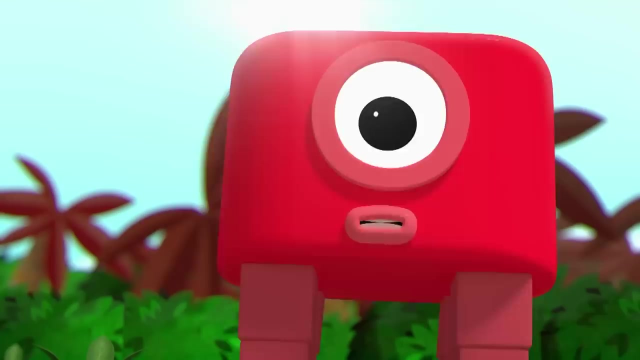 Hehe, Haha, Haha, Haha. Where Ah A leap into the unknown? Great, Oh, Oh Ah, Welcome. Ah, Are you The fabled table, The one with the sign of the times? 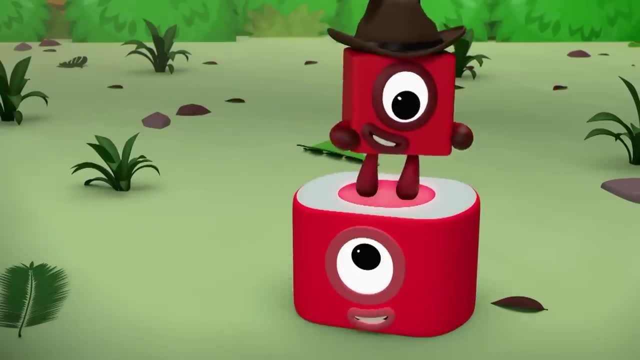 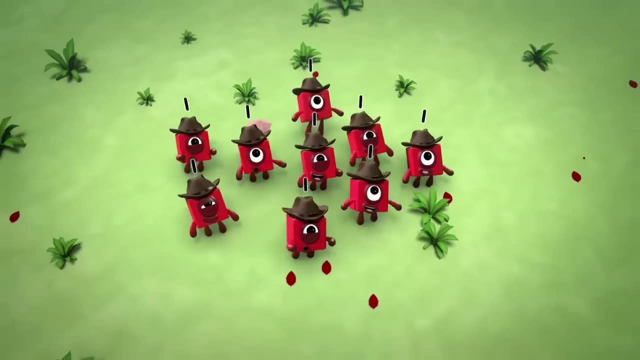 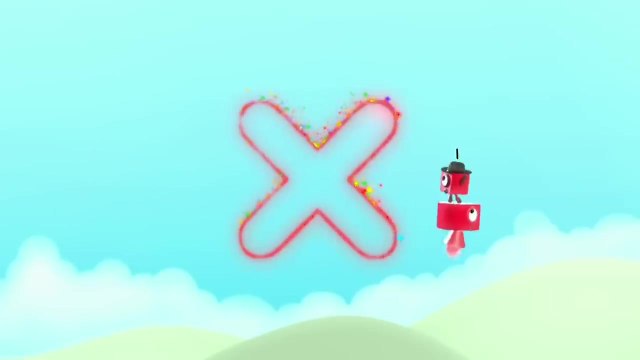 First time. Let's go. Ooh, Come with me and you will see I like wands And wands like me. You'll discover what I do. That's no X, But it may be a clue. You may look, but never find A label. But you can see I'm one of a kind. 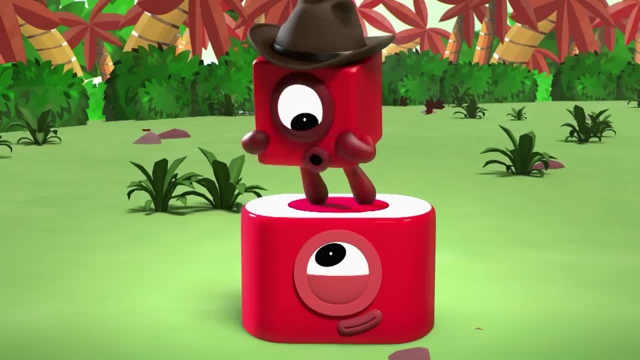 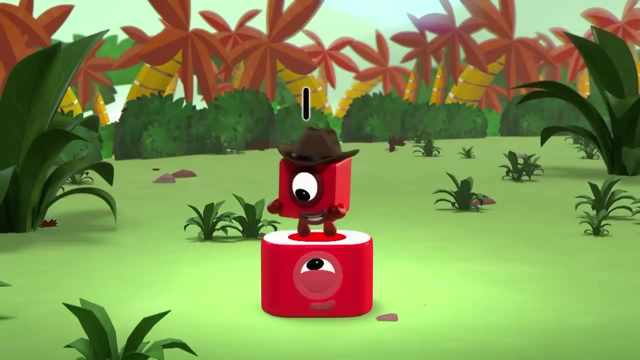 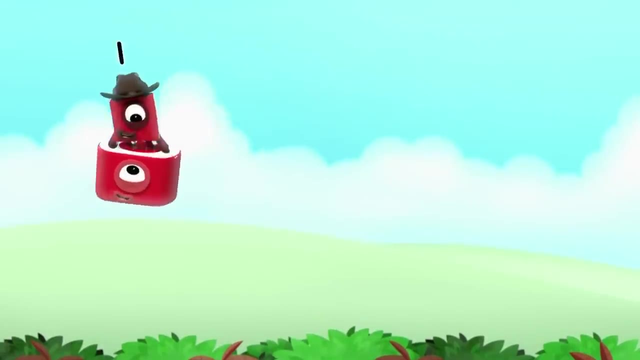 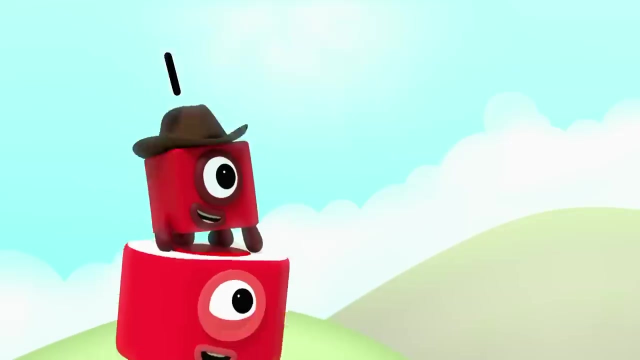 A table. Oh Wow, I've never seen a table That could fly before. Well, That's because I'm No ordinary table. I'm the fun times One times table In a wonderful world of wands. When it comes to fun, I'm the one who has tons. 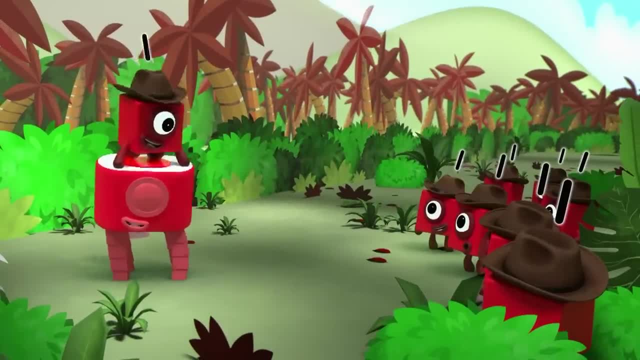 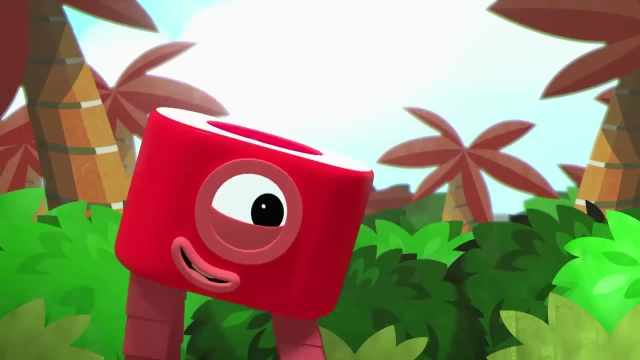 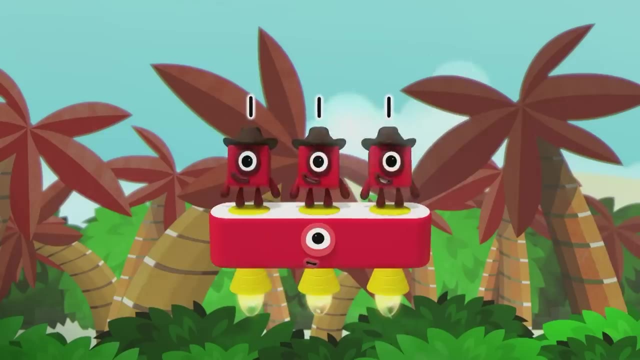 So sing along, if you're able, For fun times With the one times table. Oh Ah ah ah. One at a time, please, One. one is one. Two wands are two. Three wands are three. Four wands are four. Five wands are five. 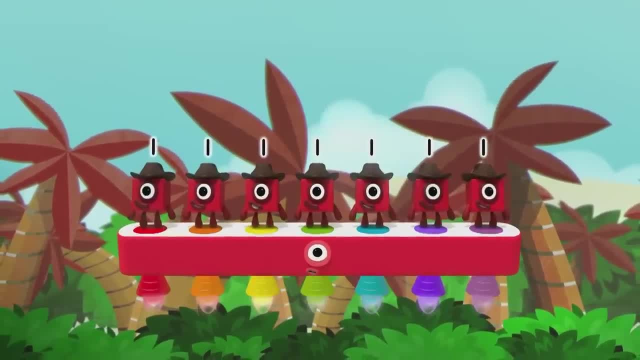 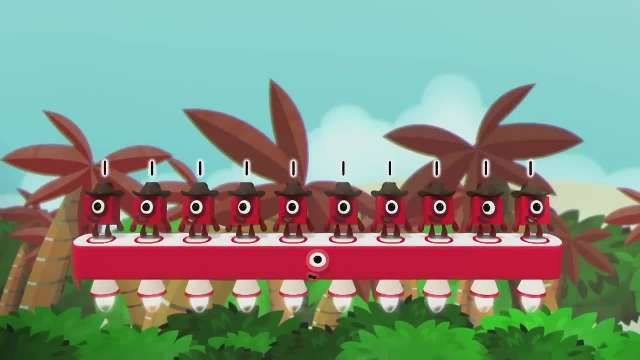 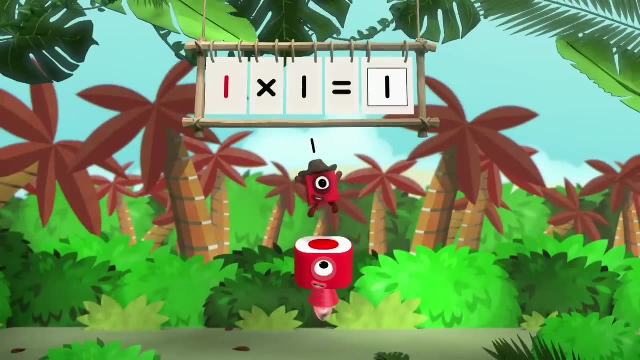 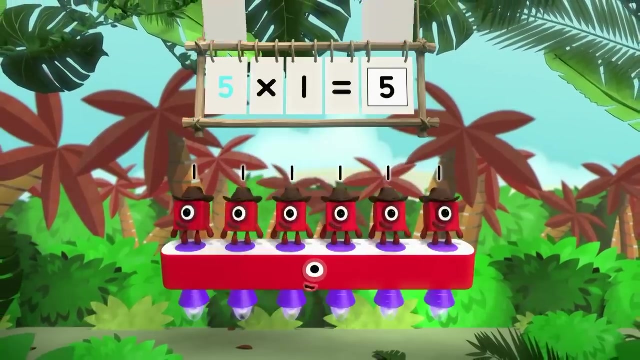 Six wands are six And seven wands Are seven. Eight wands are eight, Nine wands are nine And ten wands Are ten. Sing along: One one is one, Two wands are two, Three wands are three, Four wands are four. Five wands are five. 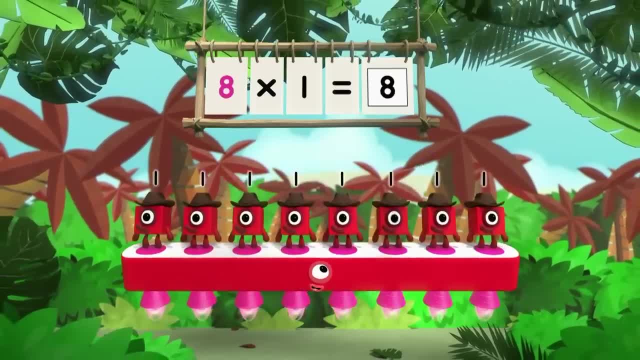 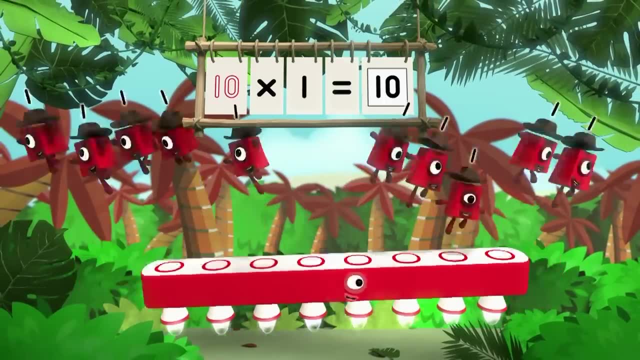 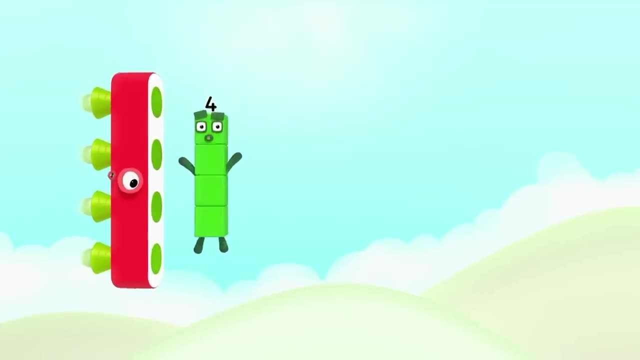 Six wands are six And seven wands Are seven. Eight wands are eight, Nine wands are nine And ten wands are ten Sideways. One one is one, Two wands are two, Three wands are three, Six wands are six And seven wands. 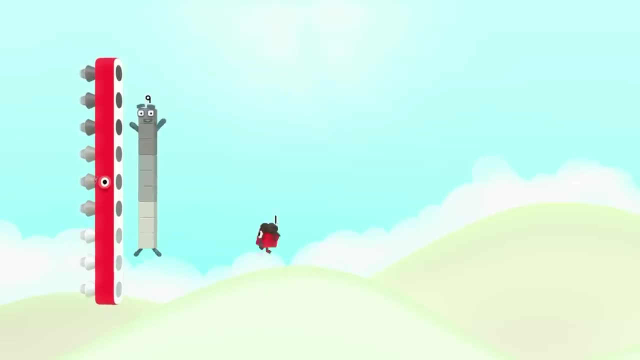 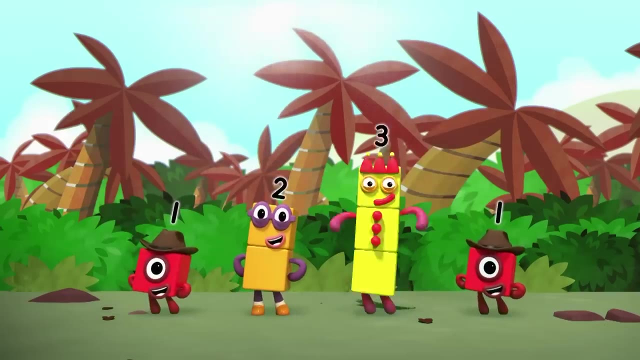 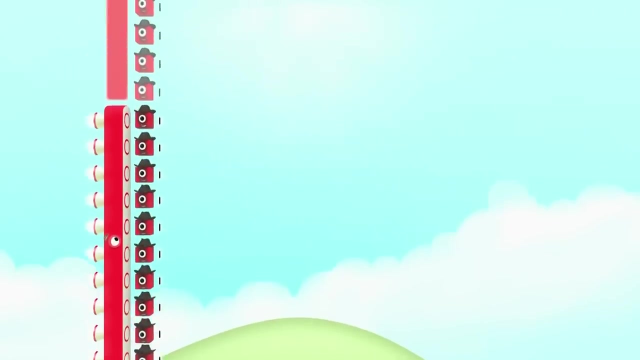 Are seven, Eight wands are eight, Nine wands are nine And ten wands Are ten. With wands, you can make any number block. Now, isn't that clever. If you just add one Or a bunch of ones, You can go on forever. I'm the fun times, one times table. 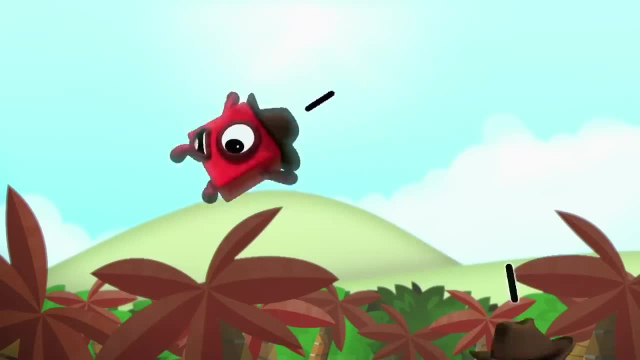 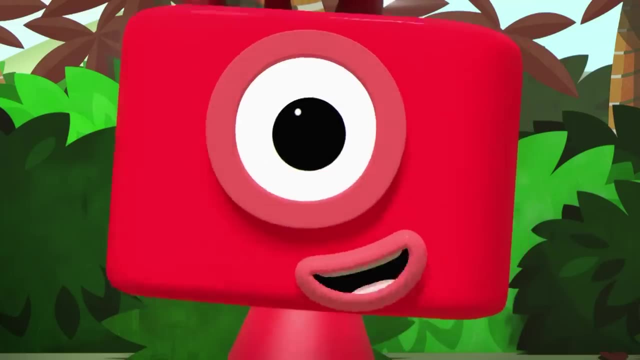 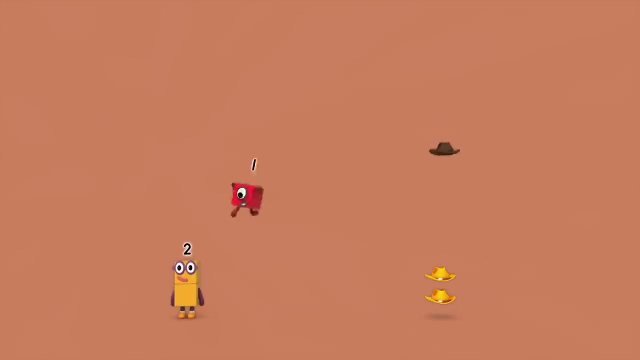 In a wonderful world of wands. When it comes to fun, I'm the one who has tons, So sing along, if you're able, For fun times with the one times table Hats. One hat is one, Two hats are two, Three hats are three, Four hats are four. 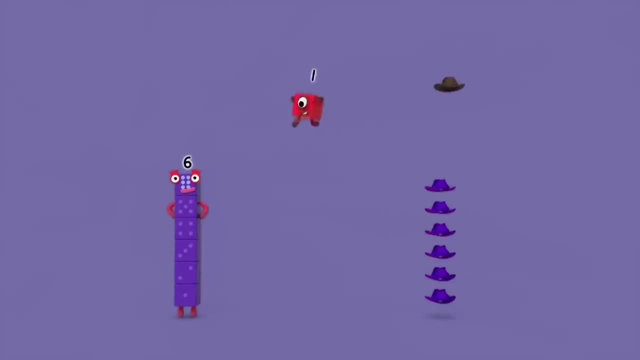 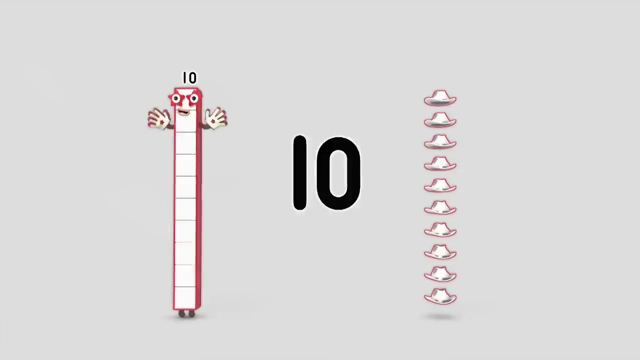 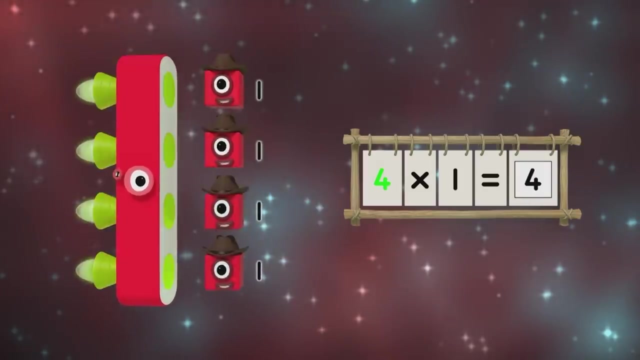 Five hats are five And seven hats Are seven. Eight hats are eight, Nine hats are nine And ten hats Are ten. One one is one, Two wands are two. Three wands are three. Four wands are four. Five wands are five. Six wands are six. 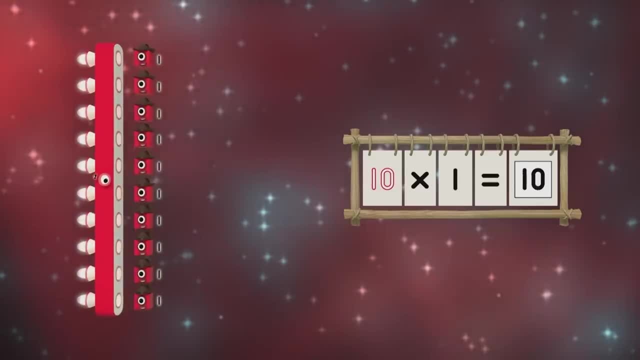 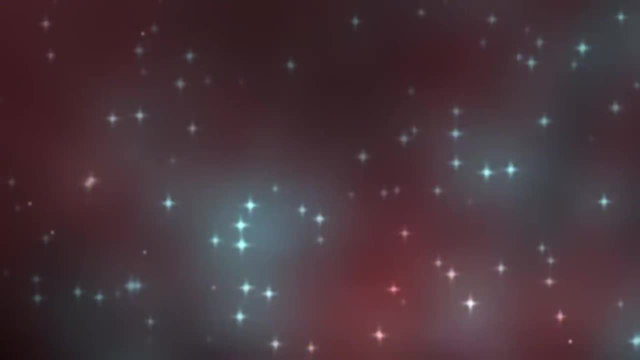 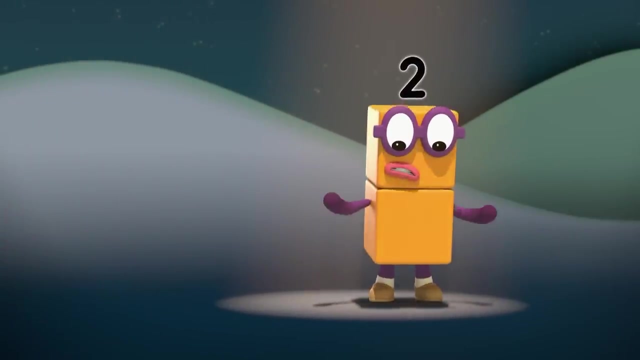 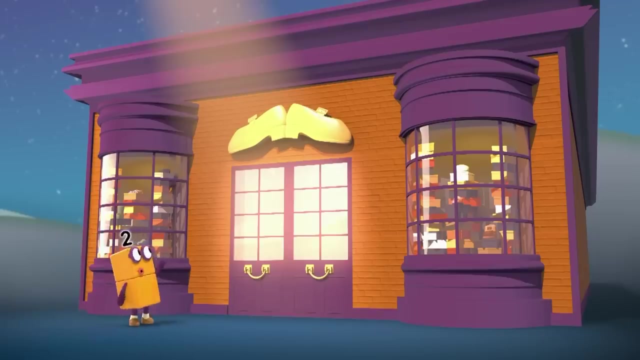 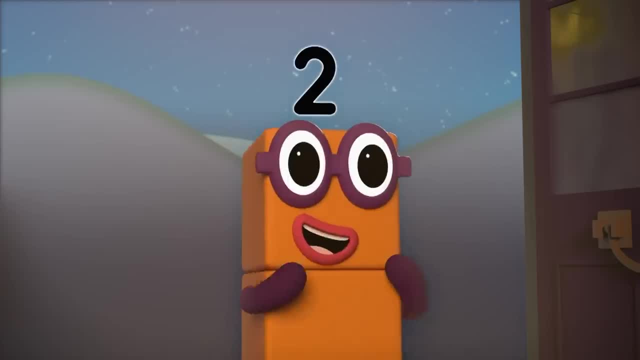 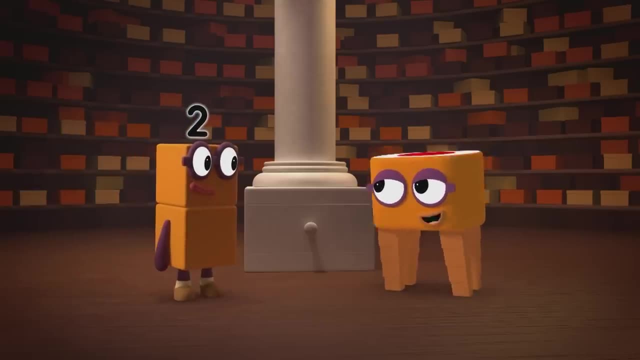 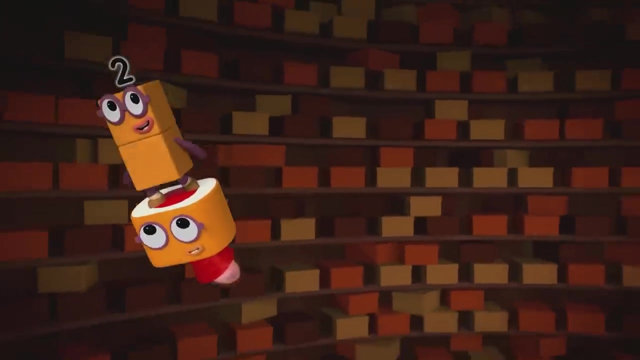 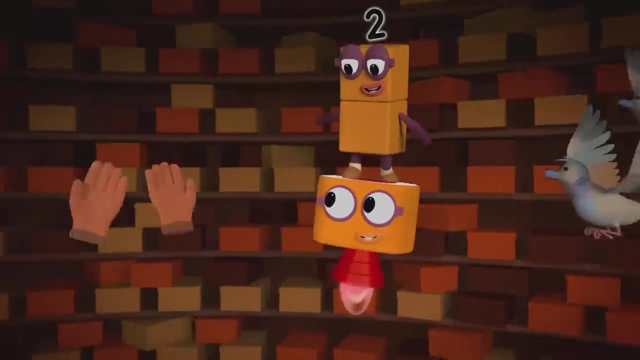 Welcome. Do you like shoes? Uh huh. Well, I like twos. I'm the two times table And we both Like to dance. I like things that come in twos. I like ears and elbows And knees. I like pairs of gloves And turtle doves. I like wings and wellies. 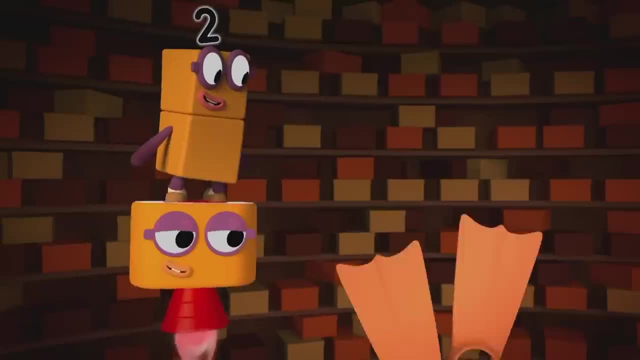 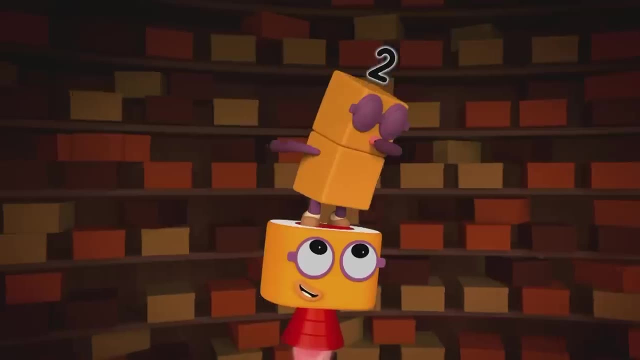 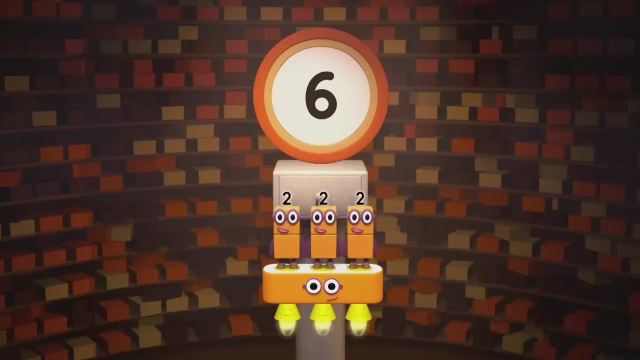 And water skis, When you're counting slippers Or flippers or shoes. This is the method you'll need to use A table for twos. One two is two. Two twos are four. Three twos are six. Are you keeping the score? Four twos are eight. 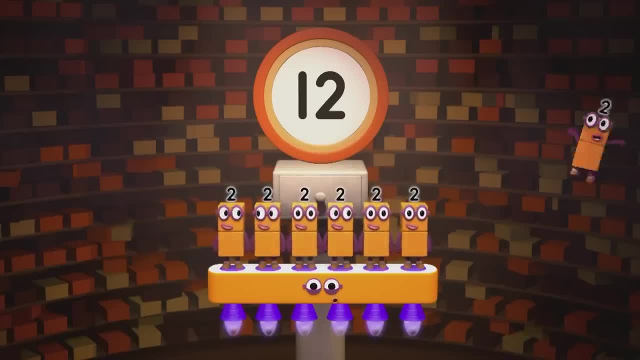 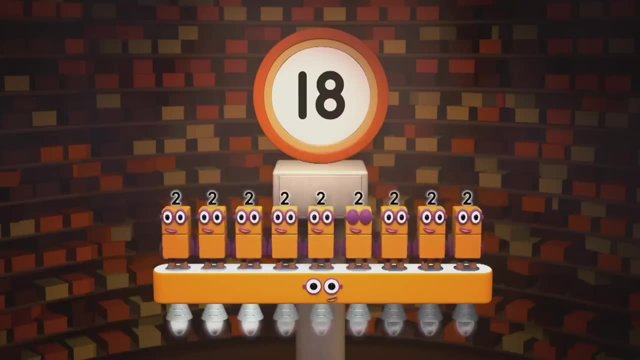 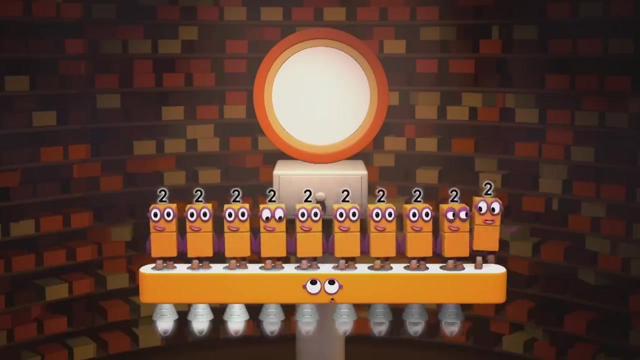 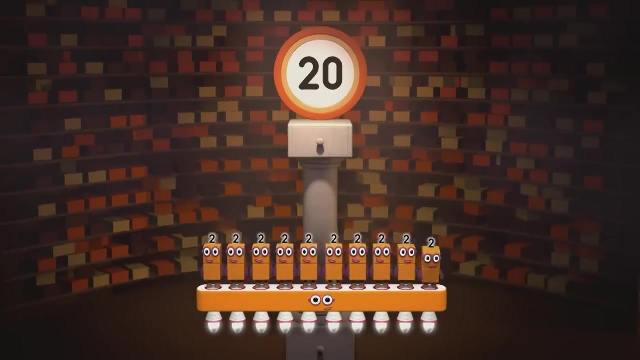 Five twos are ten. Six twos are twelve. Are you ready for more? Seven twos are fourteen. Nine twos are eighteen. That might be plenty, But why should we stop now? Reach for the top now. Ten twos, Ten twos Are twenty. It's shoe time. 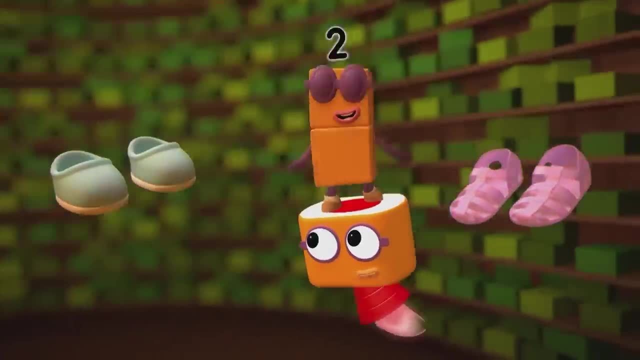 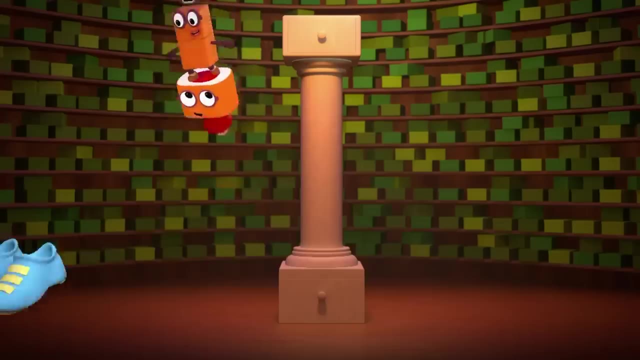 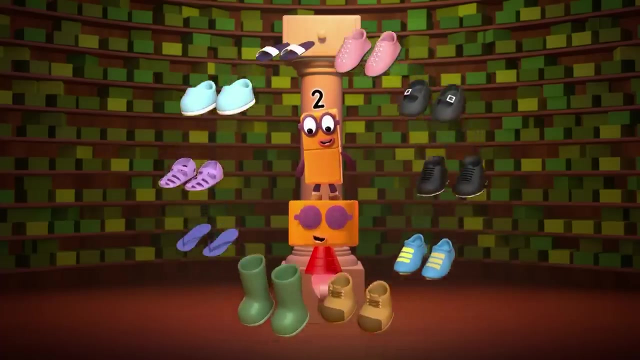 Work. boots and wellies, Flip flops and jellies, Slip-ons and sliders, Sprint shoes with spikes, Shiny black tap shoes, Flip-ons for riders Of super-fast bikes, Velcro or lace-up. Let's keep the pace up And count all the shoes In twos. 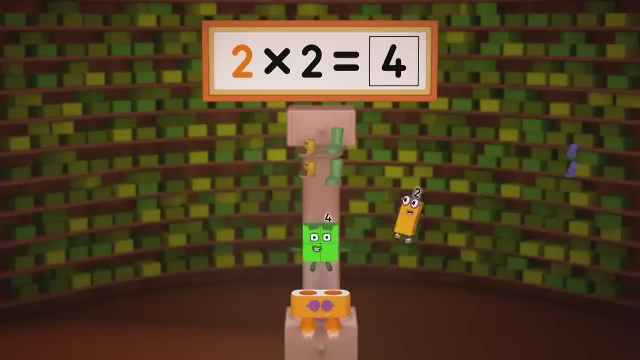 One pair is two, Two pairs are four, Three pairs are six. Now let's take to the floor. Four pairs are eight, Five pairs are ten, Six pairs are twelve. You can guess what's in store. Seven pairs are fourteen, Nine pairs are eighteen. That might be plenty, But we can still do more. 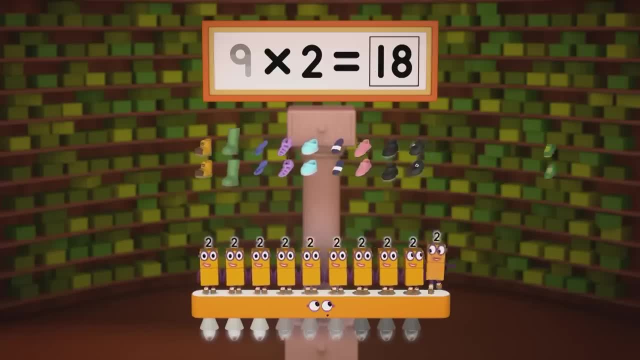 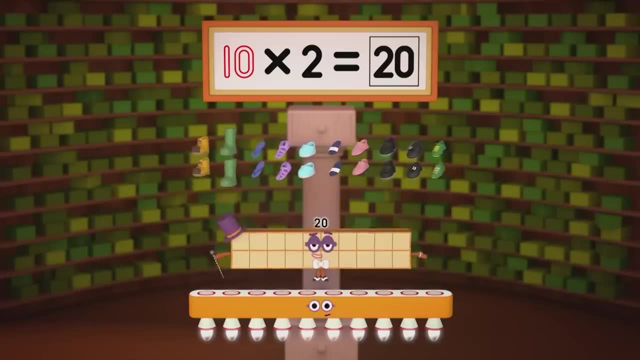 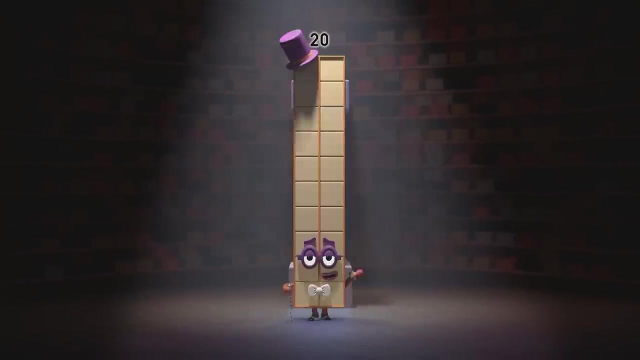 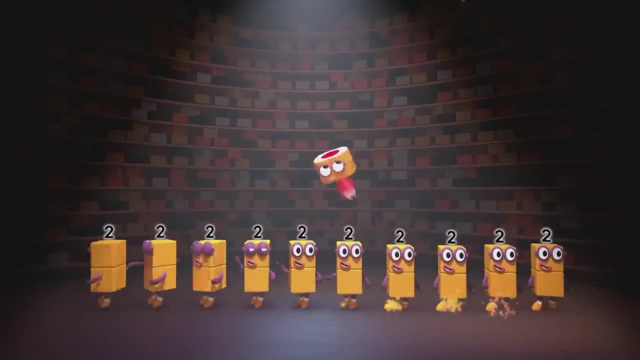 Why not have two more? Ten twos. Ten twos Are two tens. Two tens Are twenty. Two tens can tango And do the fandango: Twenty unstoppable Swappable blocks. Ten twos can line up. And where there are shoes, There are usually socks, Stroppy and spotty. 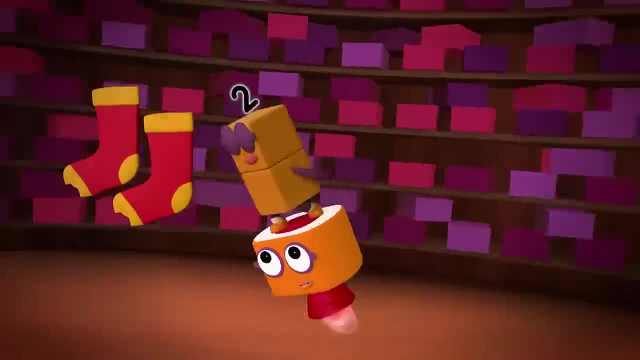 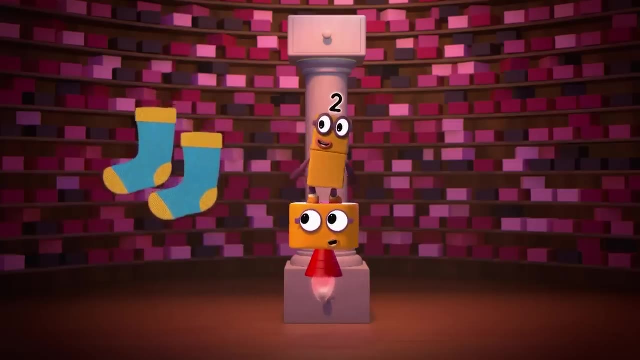 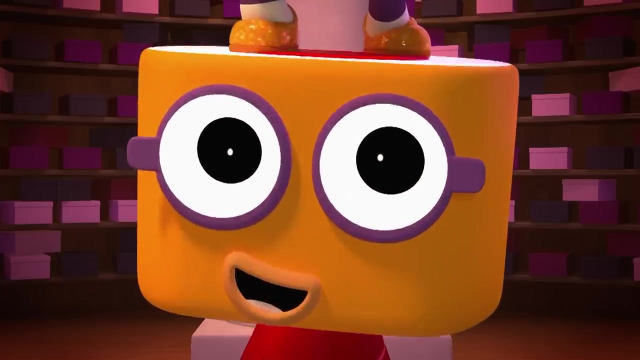 Diamond and dotty, Yellow and red socks With holes in the toes, Long socks and short socks, School socks and sports socks, Warm woolly bed socks, Which grandma once chose, Silky and snazzy, Jolly and jazzy. Let's count them all Good call. 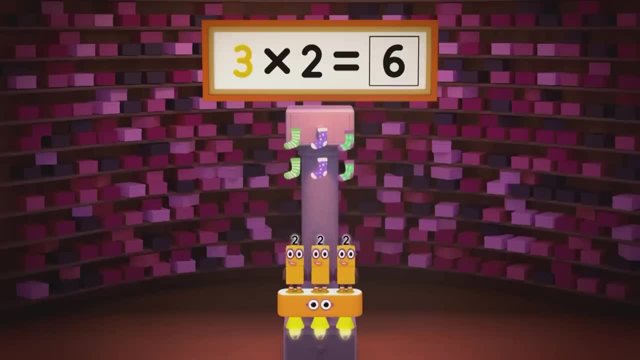 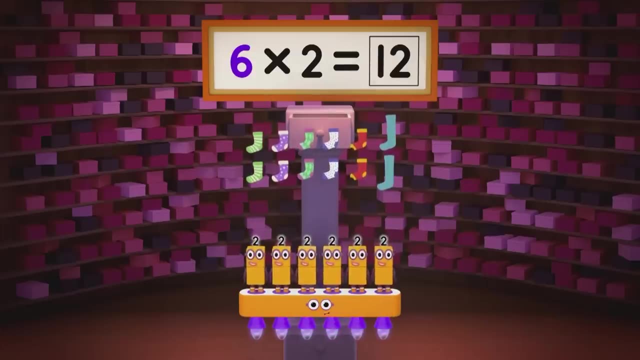 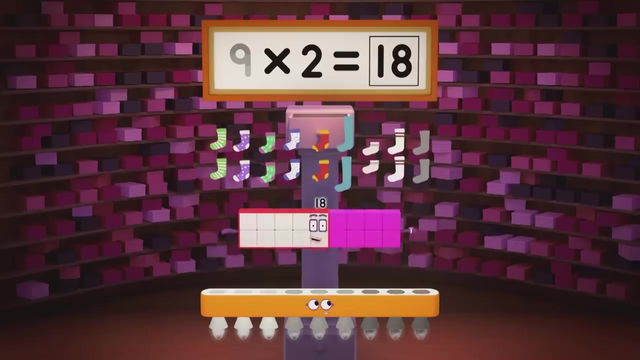 One pair is two, Two pairs are six. Now let's open the drawer. Four pairs are eight, Five pairs are ten, Six pairs are twelve. Socks you cannot ignore. Seven pairs are fourteen. Eight pairs are sixteen. Nine pairs are eighteen. That might be plenty. Let's have some new socks. 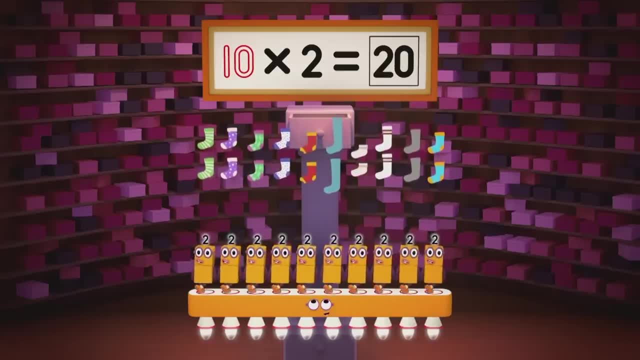 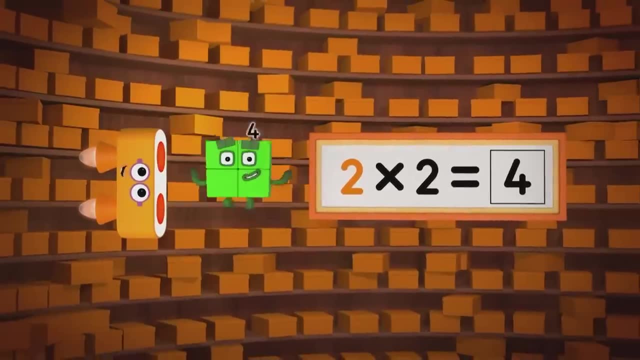 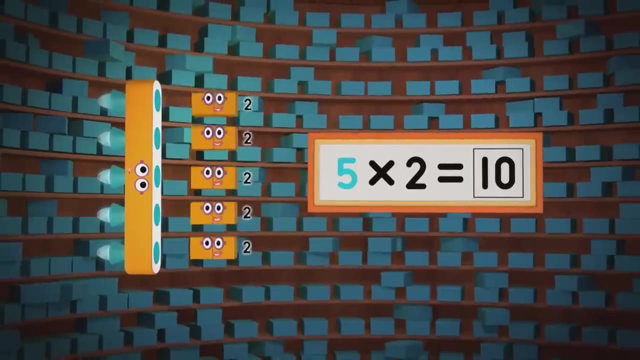 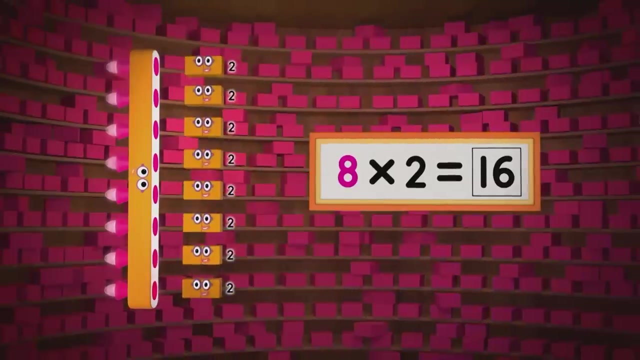 Orange and blue socks. Ten pairs Are twenty. Sideways, One pair is two. Two pairs are four. Three pairs are six. Are you keeping the score? Four pairs are eight. Five pairs are ten. Six pairs are twelve. Are you ready for more? Seven pairs are fourteen. Eight pairs are sixteen. 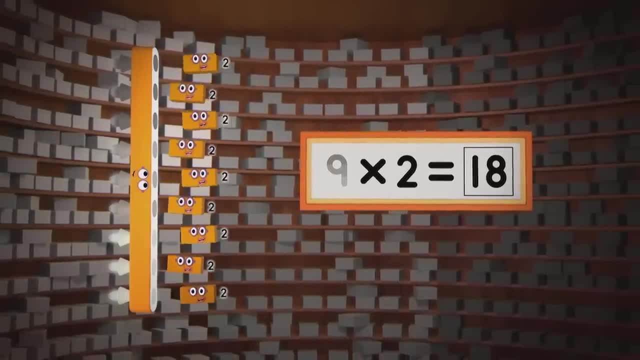 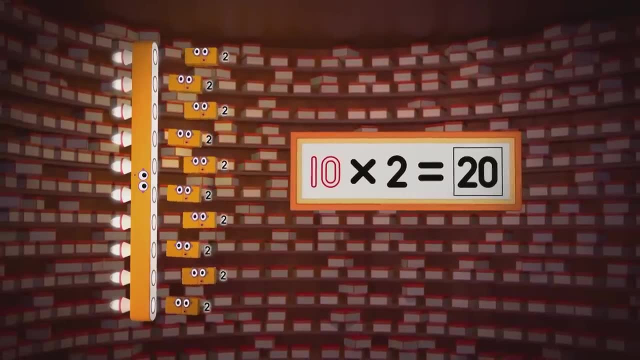 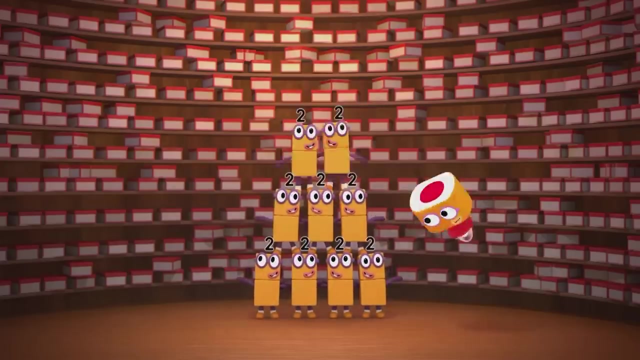 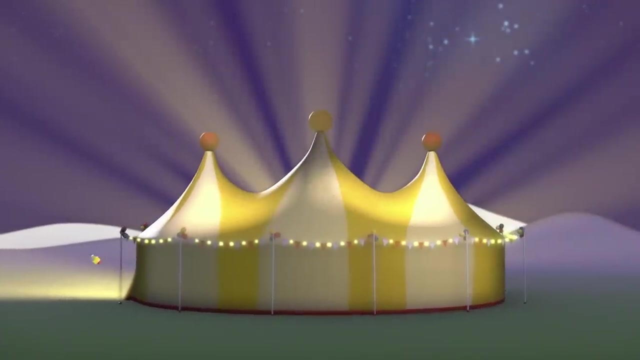 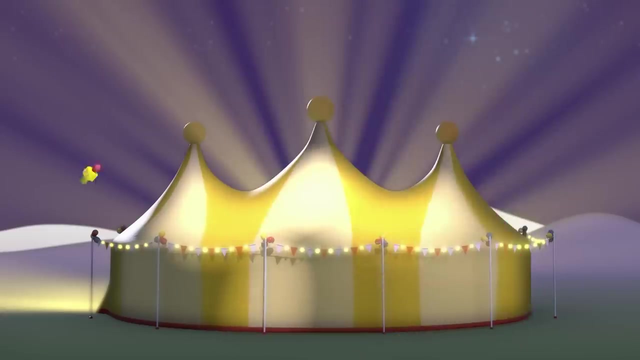 Nine pairs are eighteen. That might be plenty, But why should we stop now? Reach for the top. now 10s, Two, Ten T's are twenty. Hold Bueno 2. Roll up, roll up, roll up for The Circus Of Threes with your ringmaster. 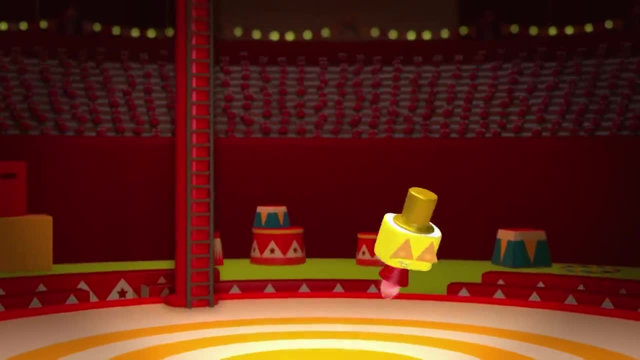 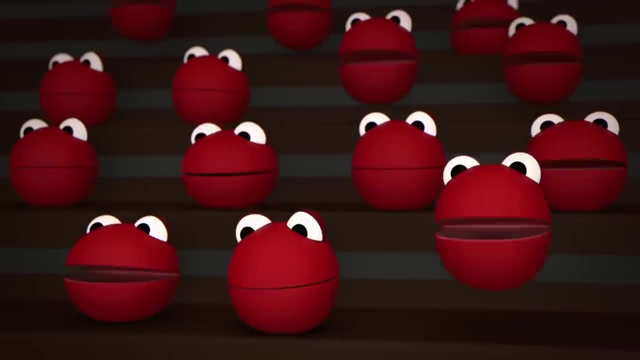 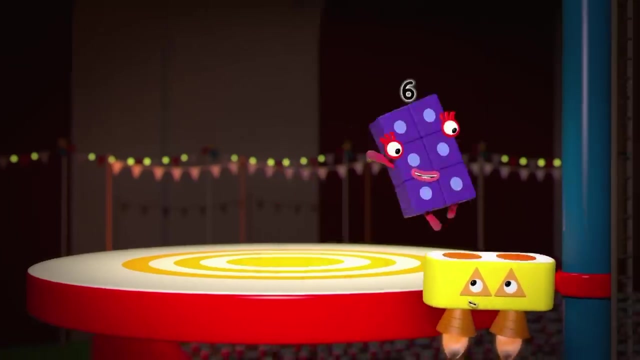 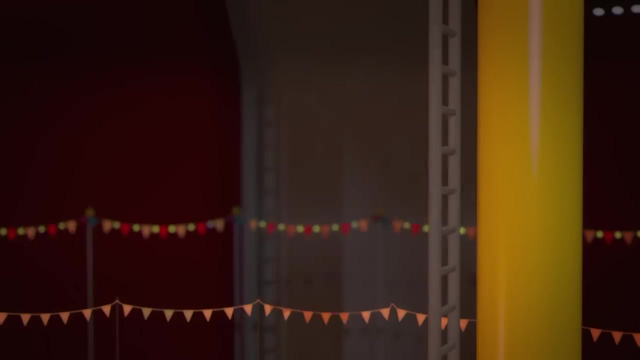 Me Three times two. One, three is three, with a juggling act to open the show. Two, threes are six. with one roll of the dice, the excitement will grow. Three, threes are nine. who might get to the top if he stifles that sneeze? 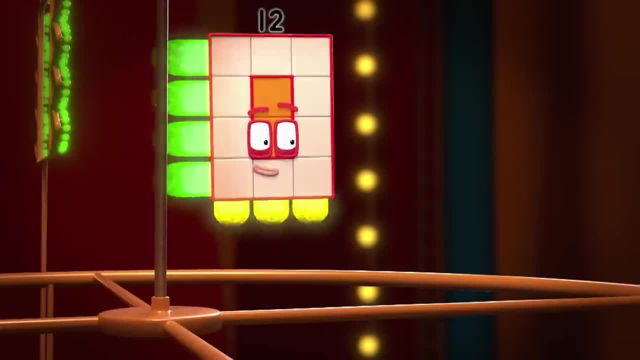 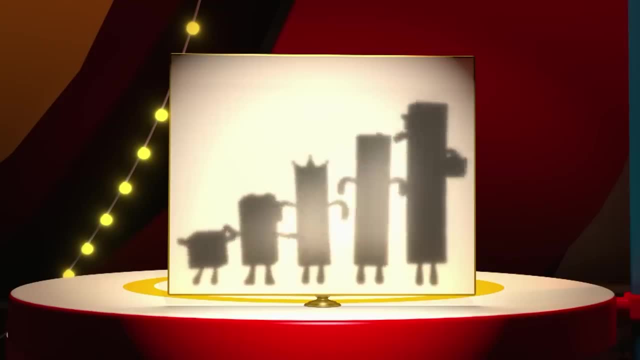 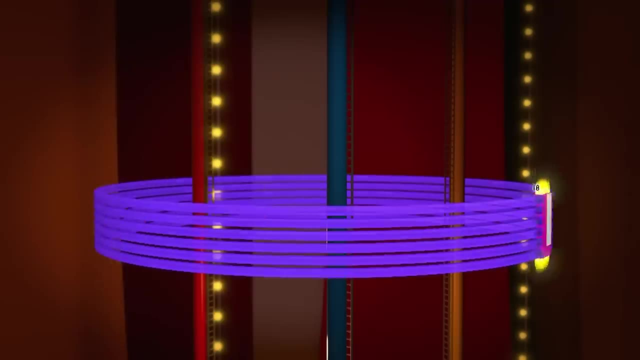 Four, threes are twelve. a rectangular marvel she floats with the greatest of ease. Five, threes are fifteen. a secretive type. her antics are mostly mysterious. Six, threes are eighteen. a master of hype shoots past and the crowd is delirious. 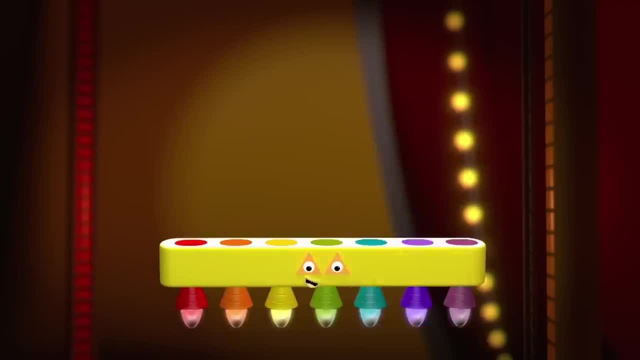 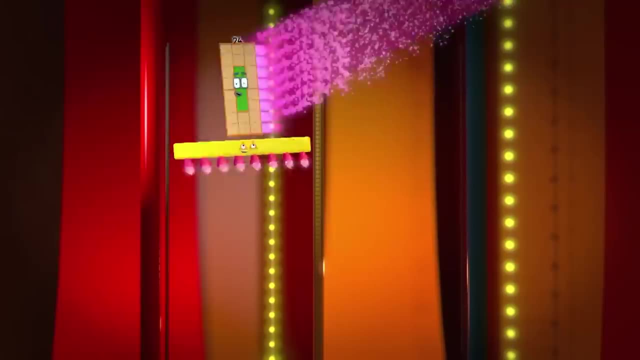 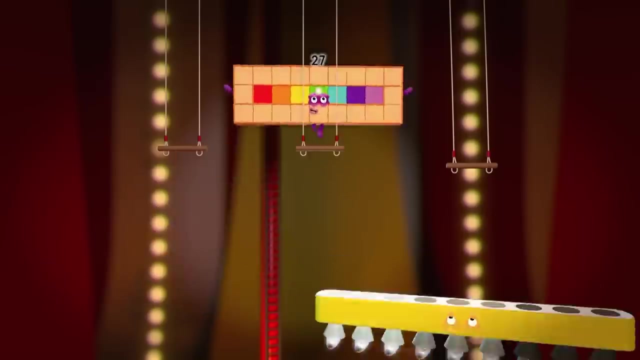 Seven, threes are twenty-one. a fearless explorer with talent to spare. Eight, threes are twenty-four, blazing a trail that glows in the air. Nine, threes are twenty-one. Twenty-seven threes. sets of three threes on the flying trapeze. 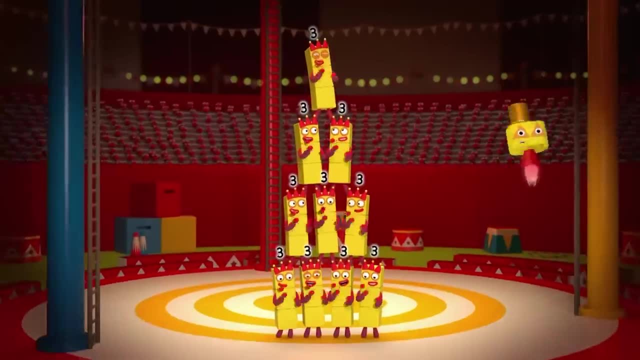 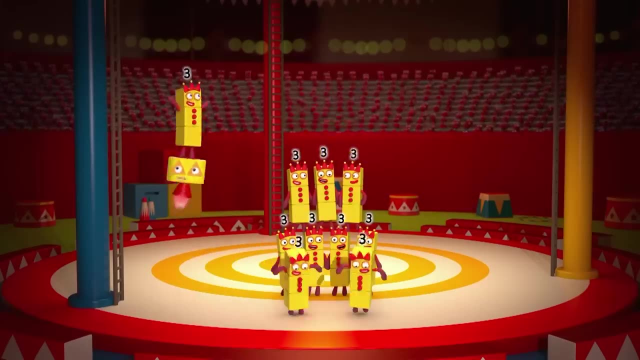 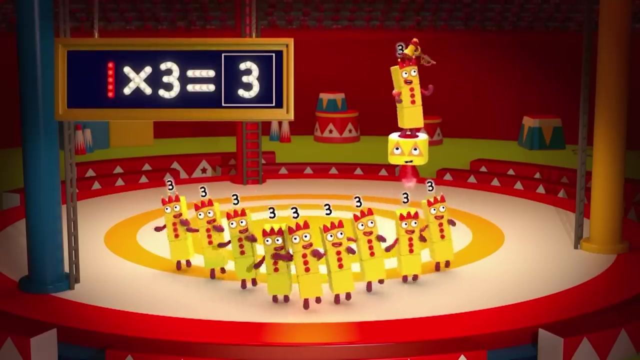 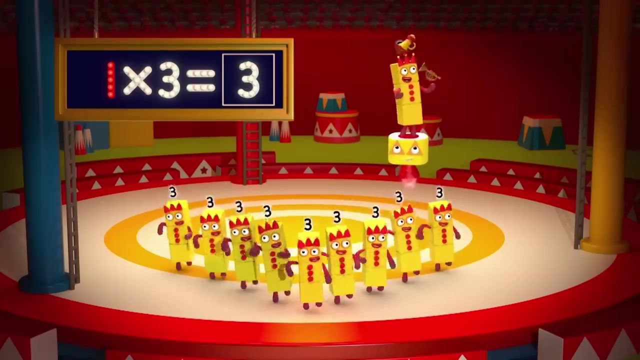 Ten. threes are thirty. ten. threes take the crown. the circus of threes is coming to town. Three's at the head of the big parade. she likes to play to the crowd. Given the choice, she prefers a vote, And her voice is really quite loud. 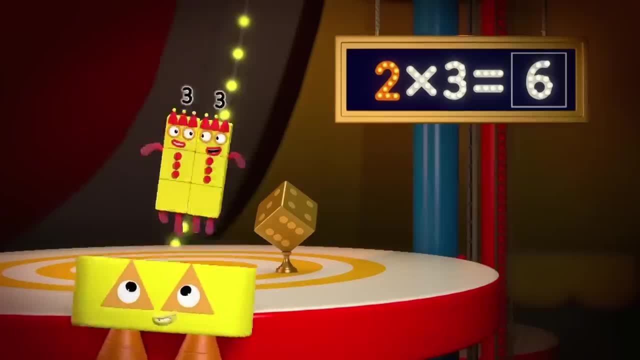 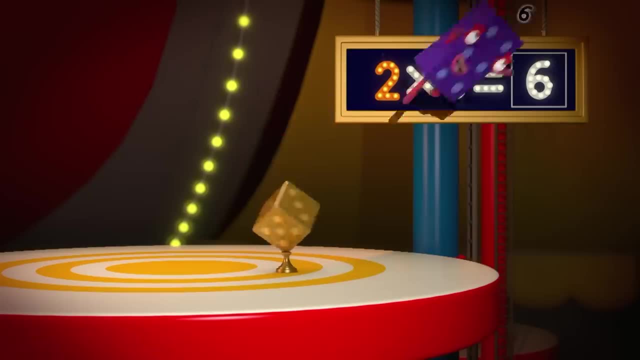 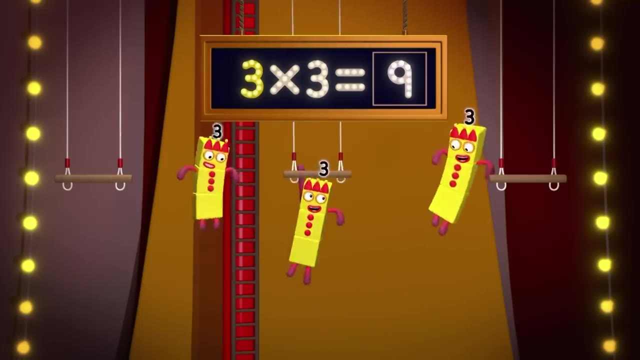 Look at me. Six is here at the top of her game with six in the mix. you'll be glad you came. Next is nine. he's on the trapeze. be careful, I think he might sneeze. Three, six, nine. 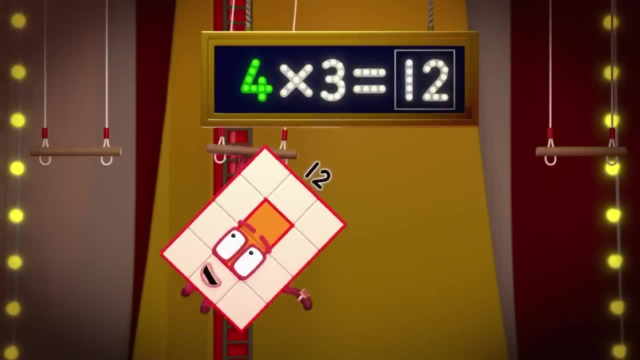 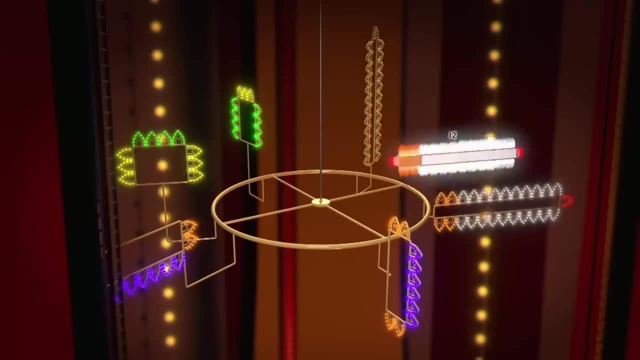 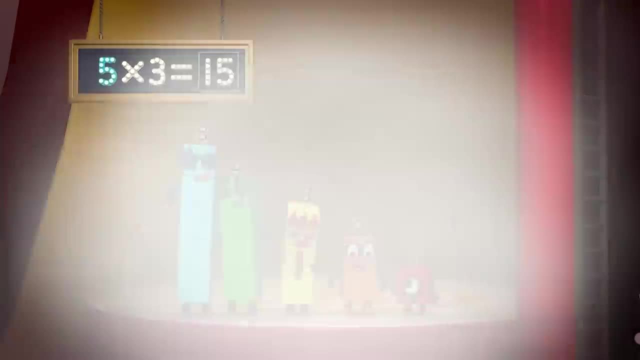 Next up is twelve. she's the fourth in line. her act will surprise and astound With her rays. she displays amazing rays as she floats with her feet off the ground. Fifteen is next with a vanishing act. she goes where no one else dares. 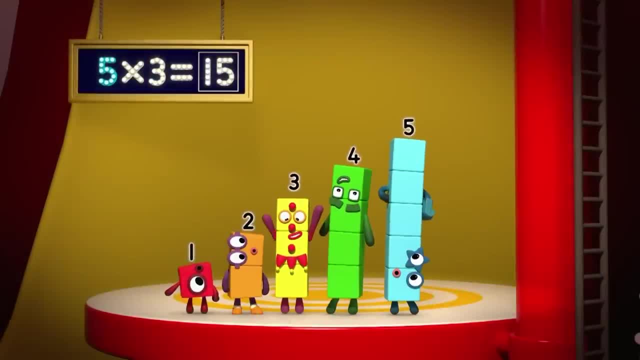 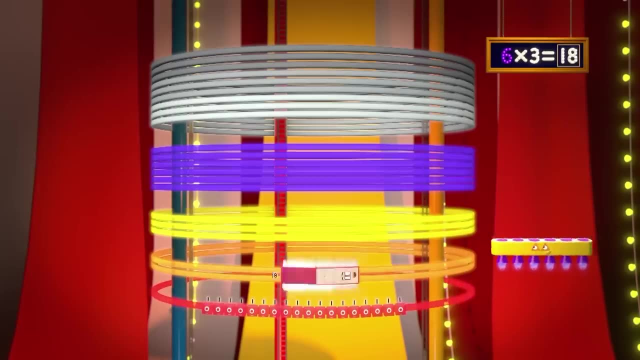 Her secretive squad may look slightly odd, but they're handy for going upstairs. Eighteen is racing around the ring, so speedy he's right off the chart. He goes past in a blur and causes a stir when he's boxed, making breaking apart. 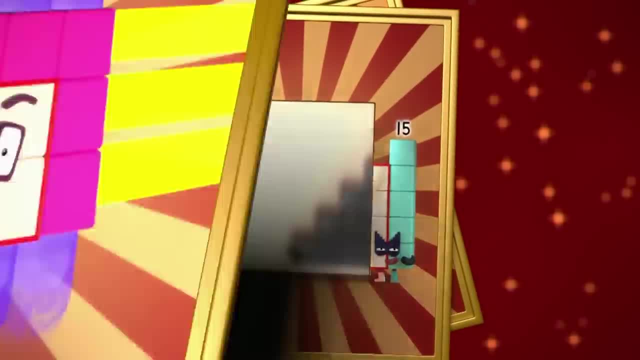 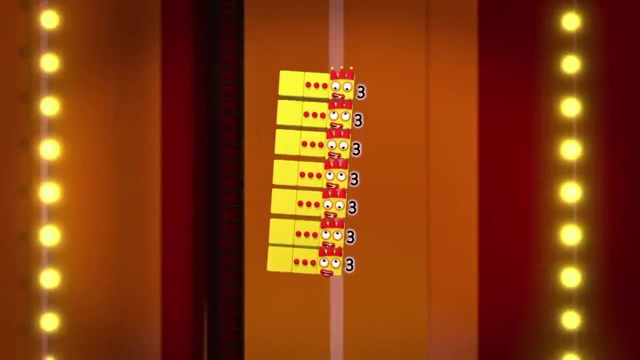 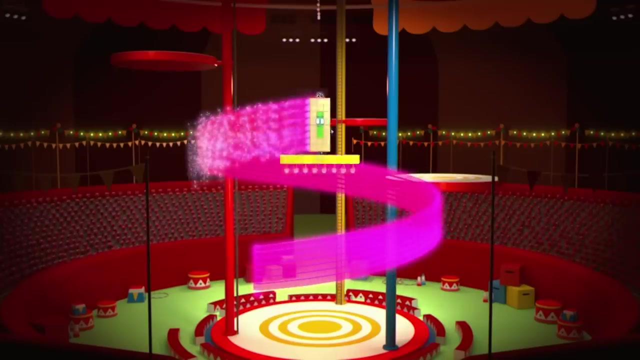 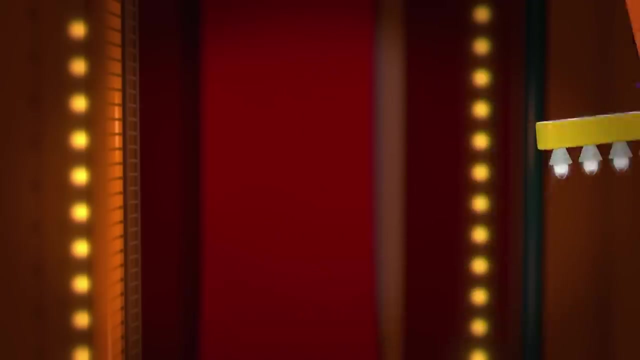 Twelve, fifteen, eighteen, Twenty-one never loses her cool as she dives into a paddling pool. Twenty-four will delight you with the light. her rays will shine all day and all night. Twenty-seven can do a neat trick: three sets of three threes in one place. 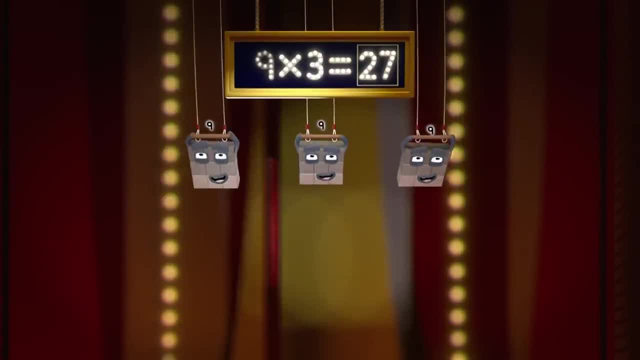 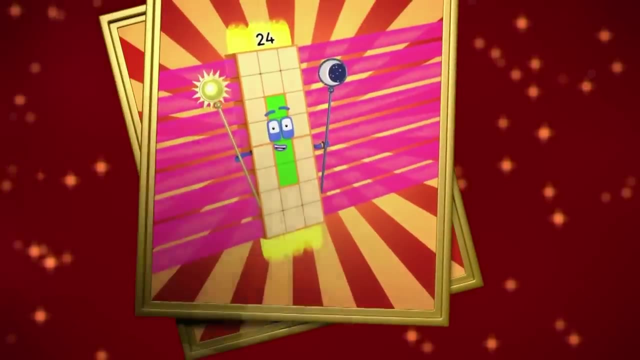 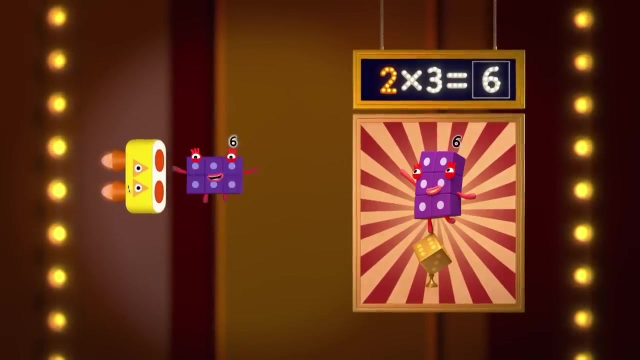 What you will see is three threes in 3D, a cube with a nine on each face. Twenty-one, twenty-four, twenty-seven. One, three is three. two, threes are six. Three, threes are nine. four, threes are twelve. 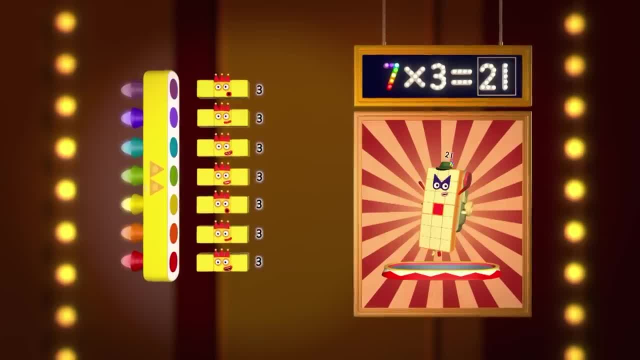 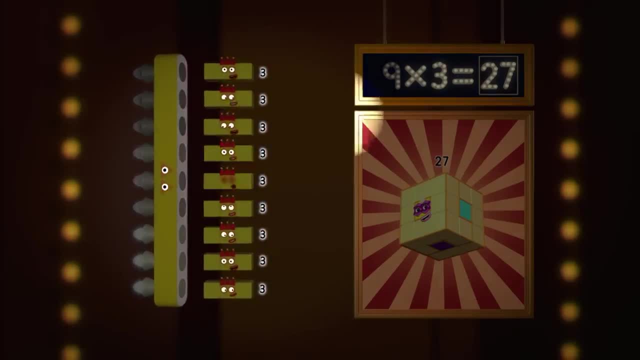 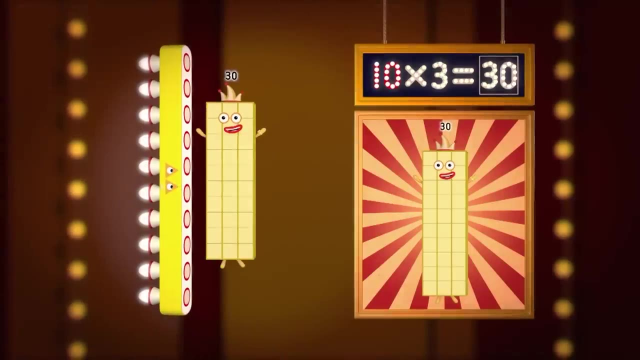 Five, threes are fifteen. six, threes are eighteen. Seven, threes are twenty-one. eight threes are twenty-four. nine, threes are twenty-seven. And now the moment you've all been waiting for: ten threes, Here's Dettie. 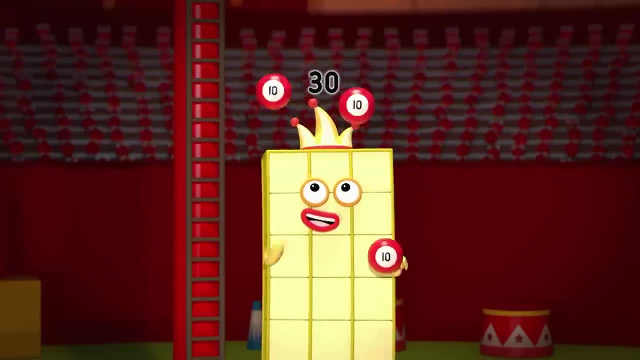 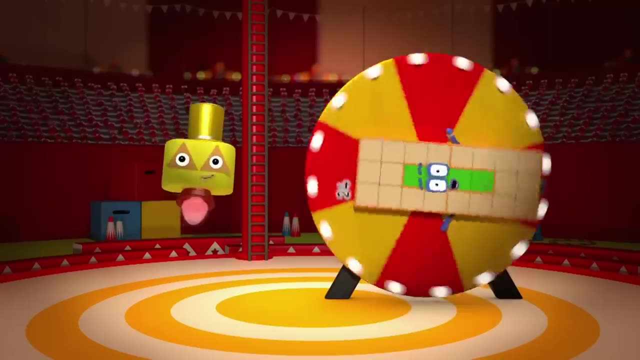 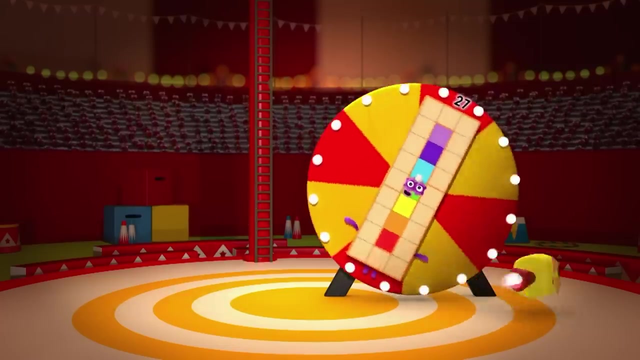 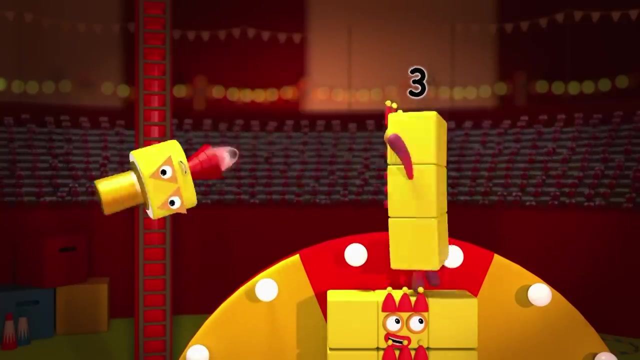 Thirteen, thirteen. the circus of threes is complete: A fabulous group, a talented troupe, the finest performers you'll ever meet. So please, raise the roof and give a big hand for the greatest show in numberland: Drum roll. please for the circus of threes. 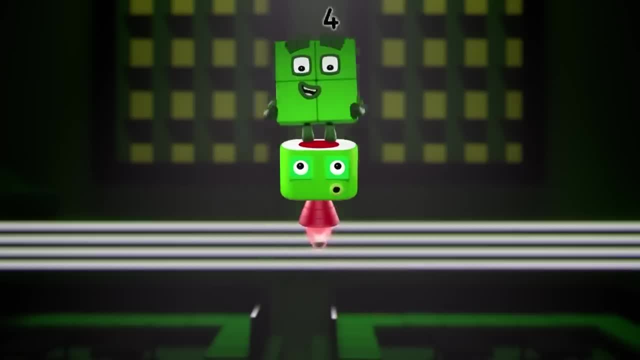 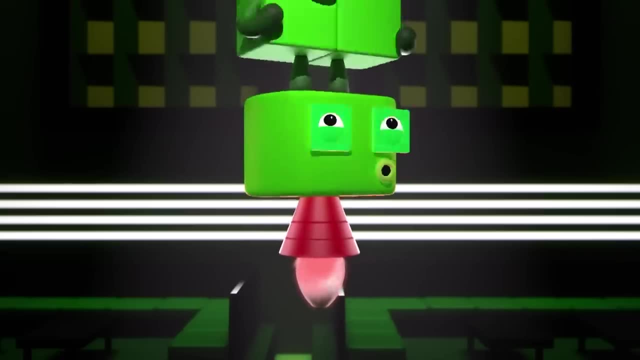 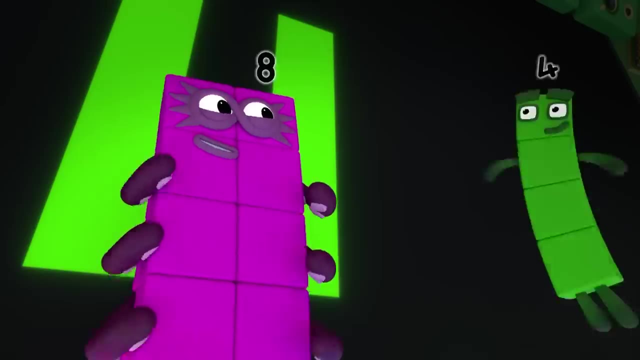 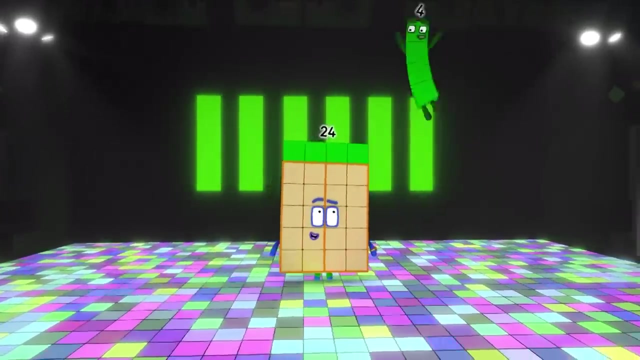 I am the four times table, calling all fours, all fours to the dance floor. Four on the floor and one more four than the four before. That's what fours are for: to get funky on the dance floor. Four on the floor and one more four, that's twenty-four, twenty-eight and thirty-two. 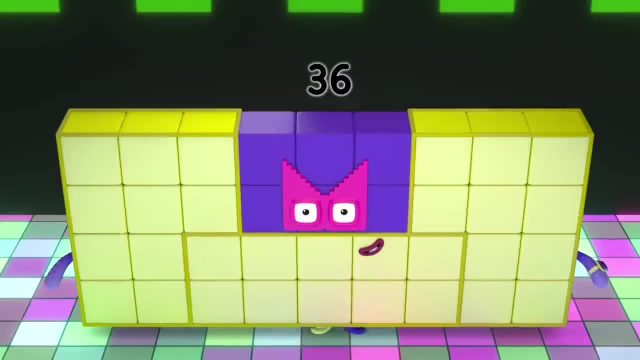 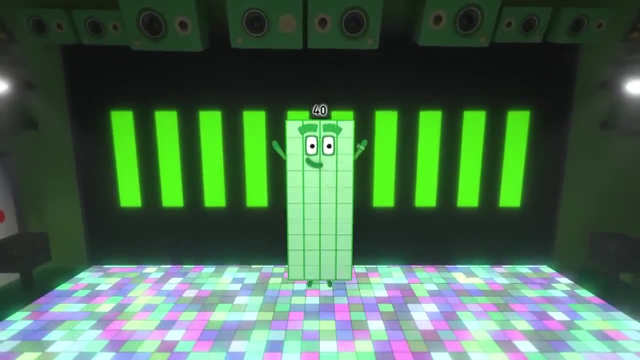 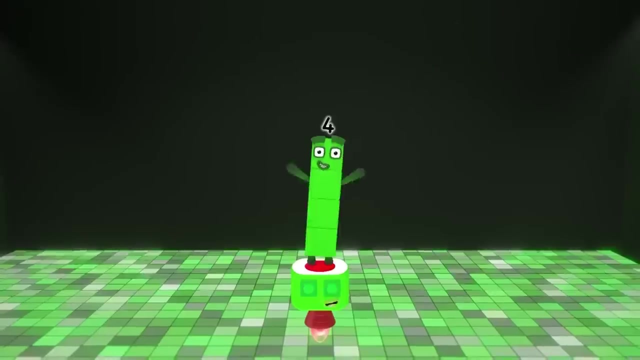 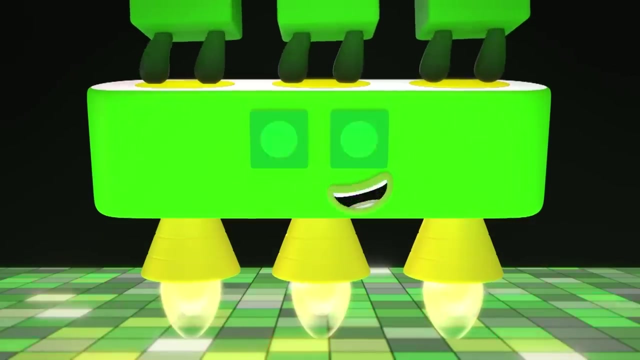 Now one more four is here to make you dance. Get down, get in the groove with thirty-six. Be there, be square when all the fours are on the floor. Here's forty. forty ten fours a forty One. four is four. two fours are eight. three fours are twelve. we know how to tell it straight. 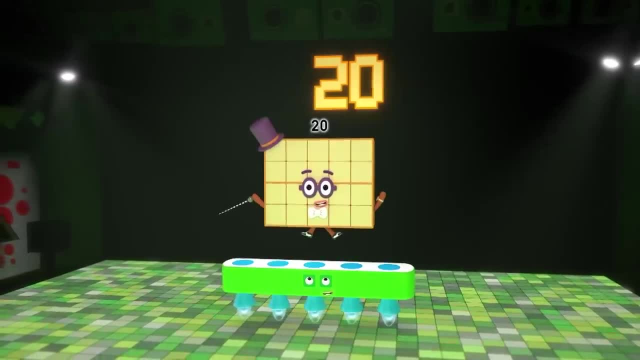 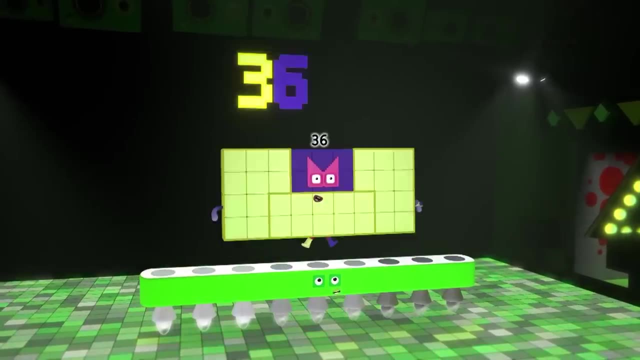 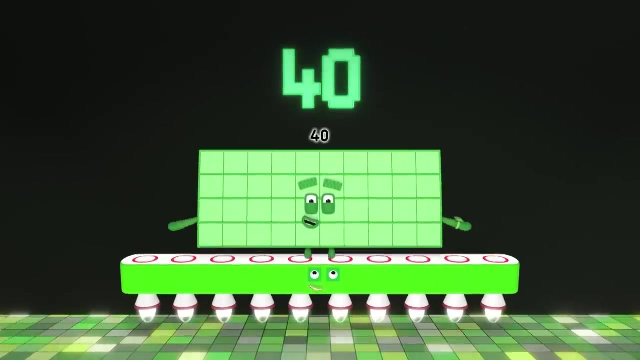 Four fours are sixteen. five fours are twenty. six fours are twenty-four. seven fours are twenty-eight. Eight fours are thirty-two. nine fours are thirty-six, and when all the fours are in the mix, ten fours are forty. Four and a four and one more four and one more four and one more four than the four before. 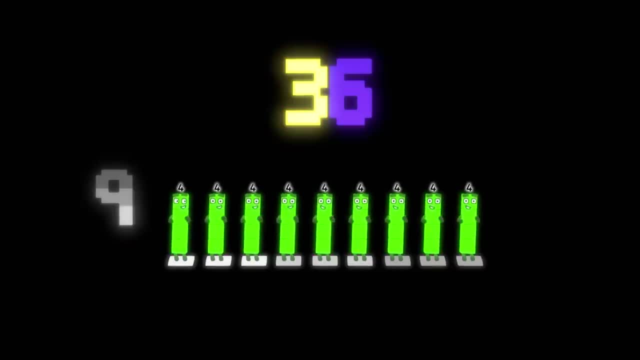 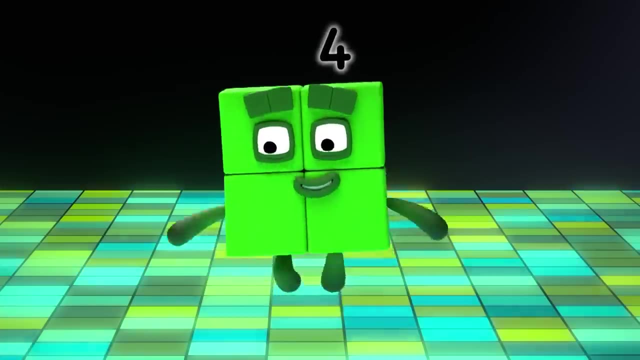 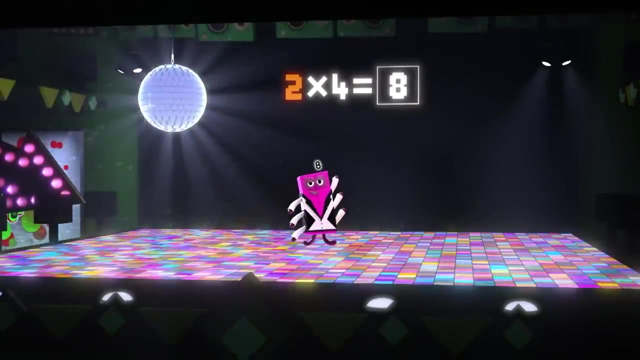 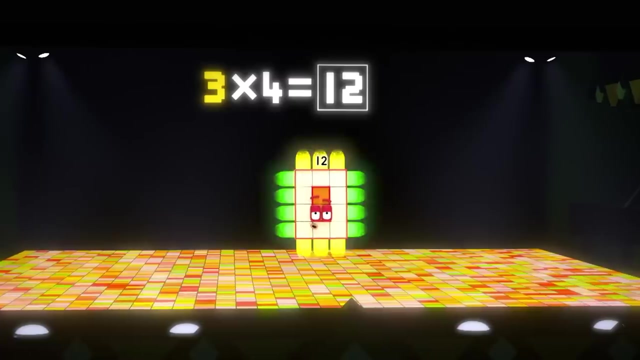 Four and a four and one more four and one more four and one more four than the four before. One four is four. Square Two fours, a eight Alto disco Three, fours, a twelve. Ride those rays, Switch, turn, switch, switch, turn. 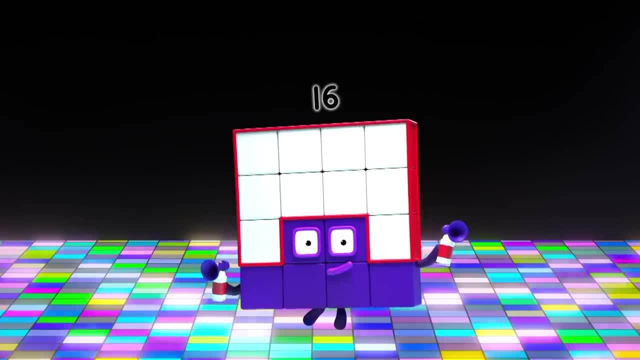 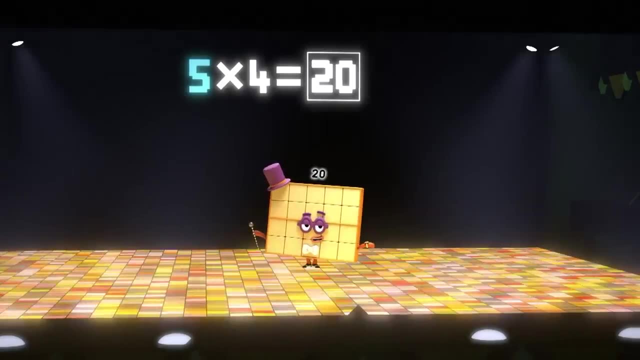 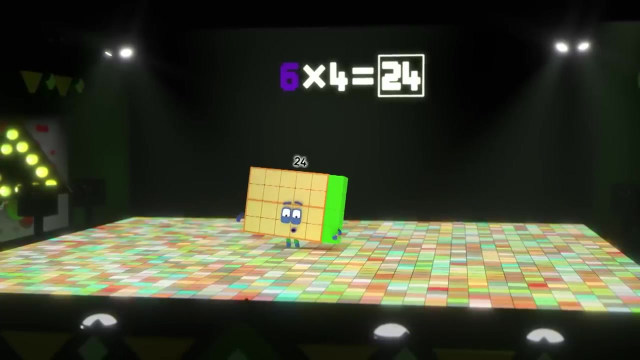 Four, fours a sixteen. Forty squares, million squares. Five, fours a twenty. Big dance number: Tap, tap, tap, tap, tap. Six, fours a twenty-four. Super duper, ride those rays, Switch turn, switch, switch tap. 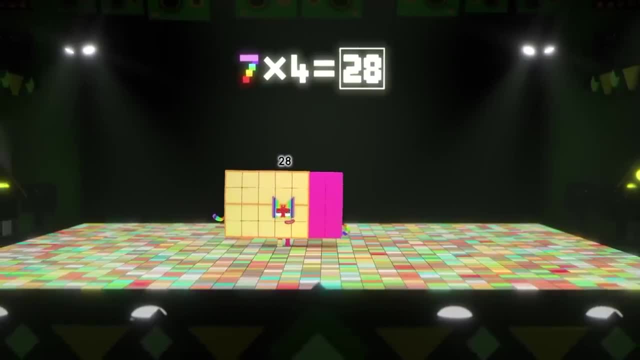 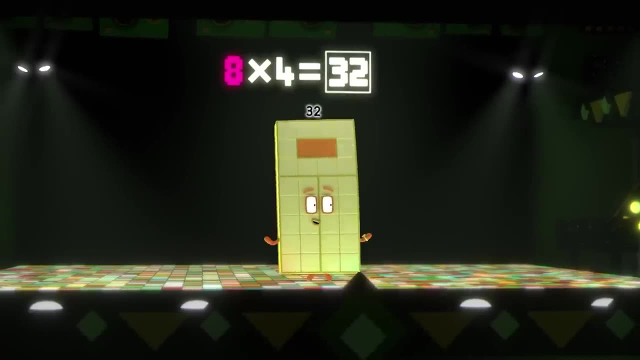 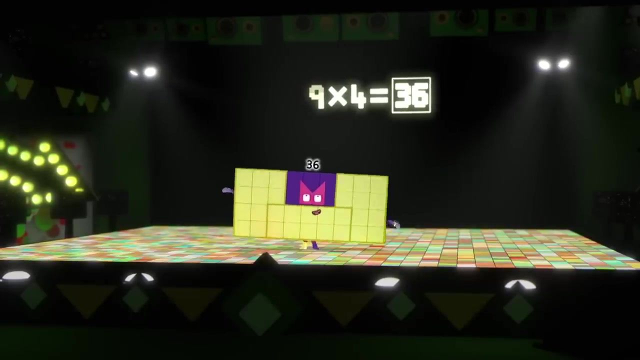 Seven fours a twenty-eight. Pick a pattern party people, Yeah. Eight fours a thirty-two. Double, double, double, double, double dance. Nine fours a thirty-six: Big, big square Made of squares, Up the stairs. 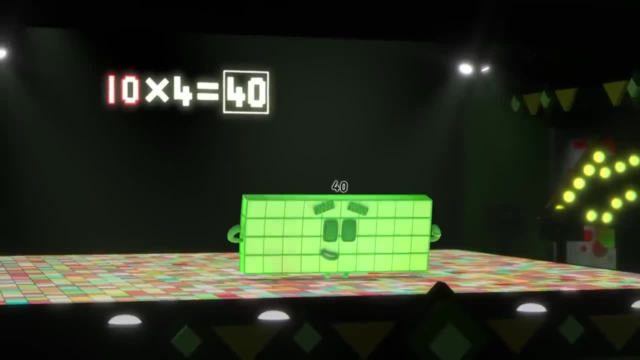 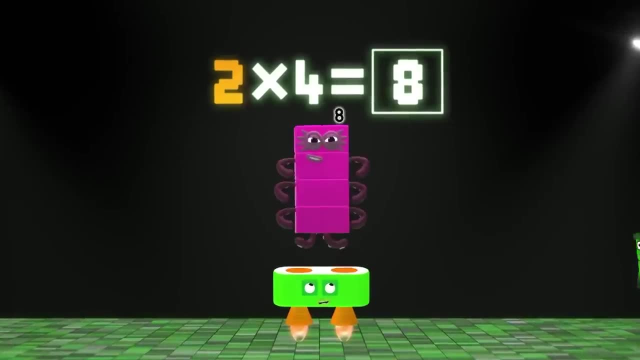 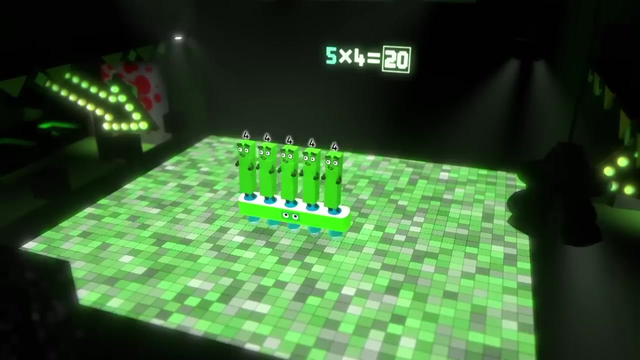 Ten, fours a forty. Great big rectangle Come on. One, four is four, Two, fours a eight, Three, fours a twelve. We know how to tell it straight. Four, fours a sixteen, Five, fours a twenty, Six, fours a twenty-four. 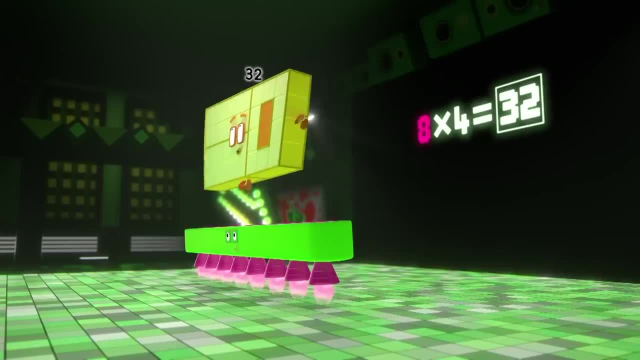 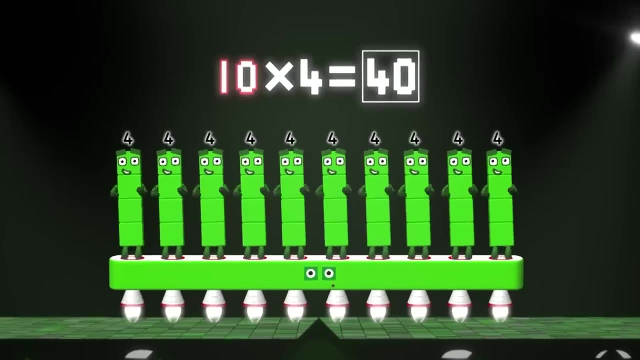 Seven fours a twenty-eight, Eight fours a thirty-two, Nine fours a thirty-six And, when all the fours are in the mix, Ten fours a forty, Four on the floor And one more four than the four before. 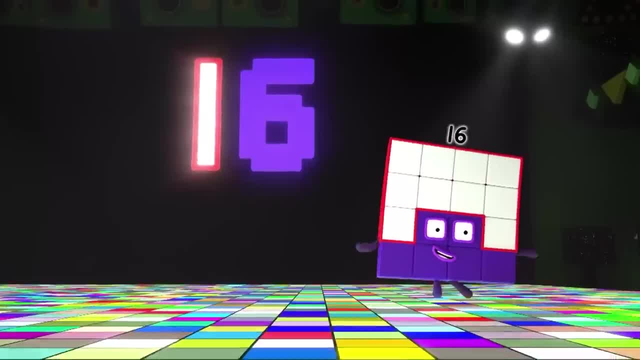 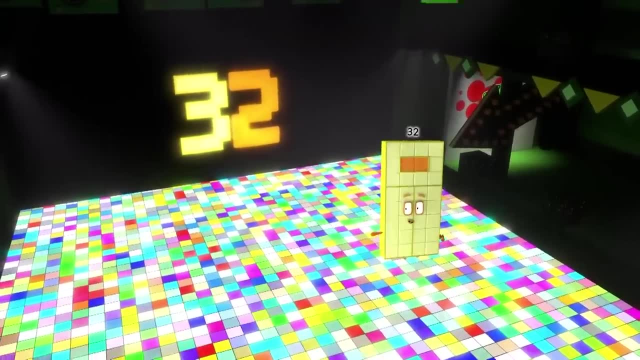 That's what fours are for: To get funky on the dance floor. Four on the floor And one more four. that's twenty-four, Twenty-eight and thirty-two. Now one more four is here to make you dance. Get down, Get in the groove with thirty-six feet. 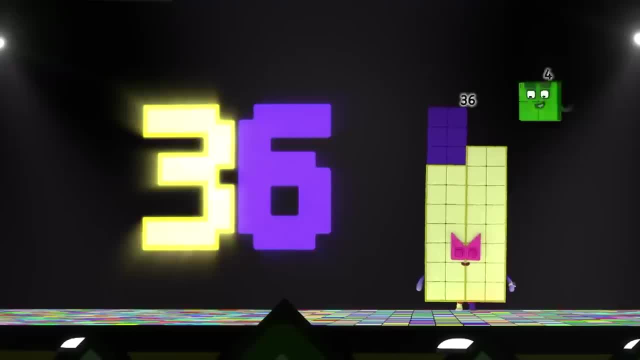 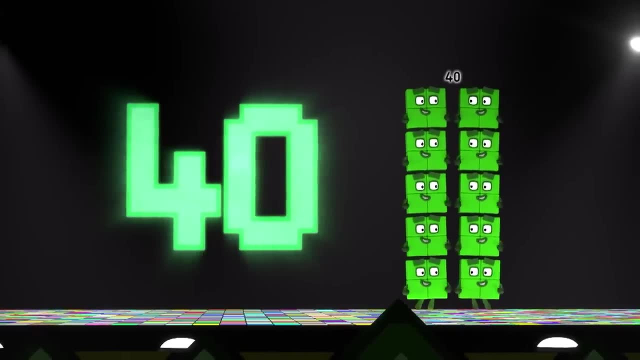 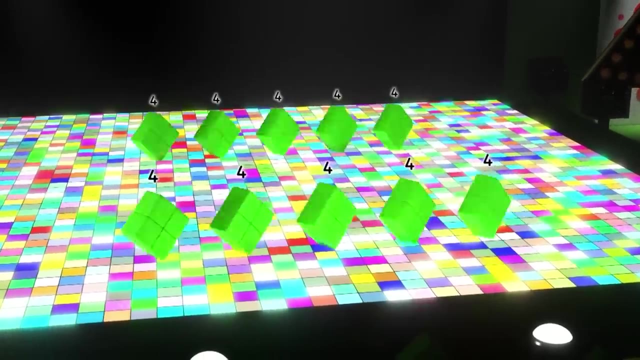 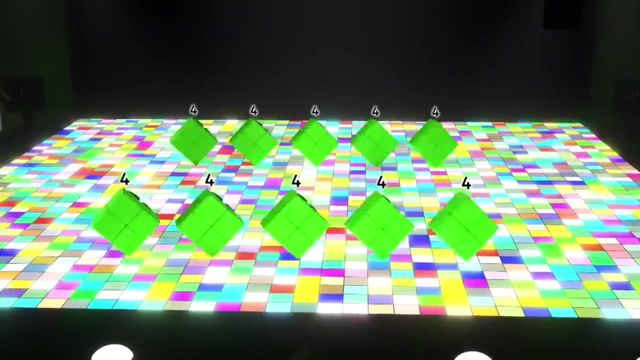 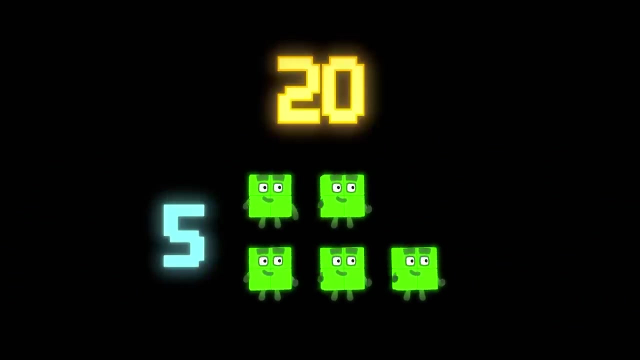 There we square, When all the fours are on the floor. Here's forty, Forty Ten fours, a forty Whoa Four and a four, And one more four And one more four And one more four than the four before. 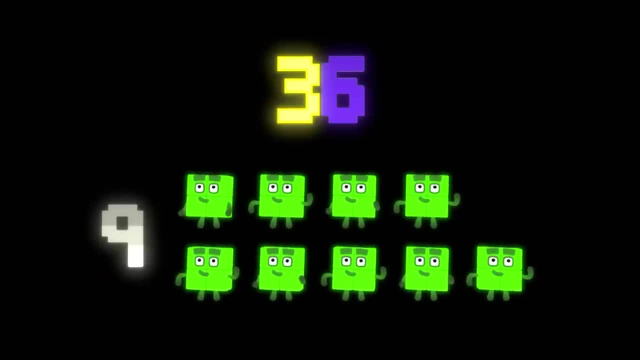 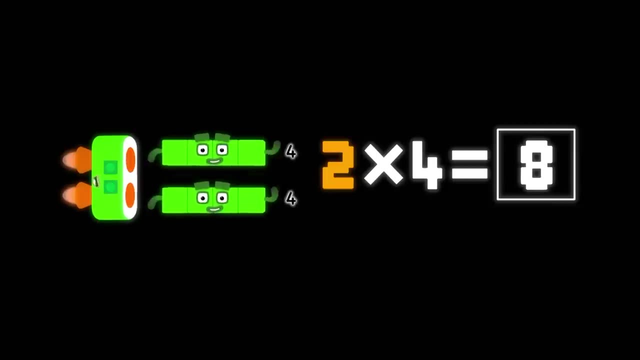 Four and a four And one more four And one more four And one more four than the four before Sideways. One four is four, Two fours a eight, Three, fours, a twelve. We know how to celebrate Four, fours, a sixteen. 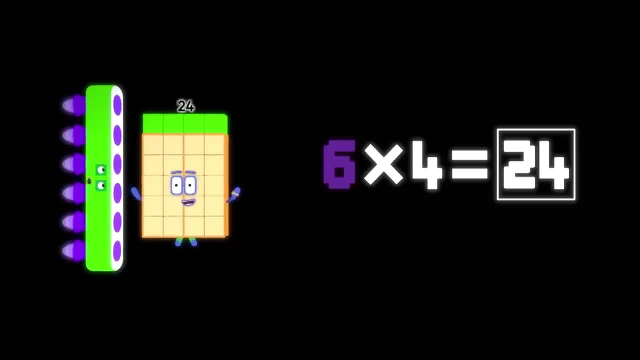 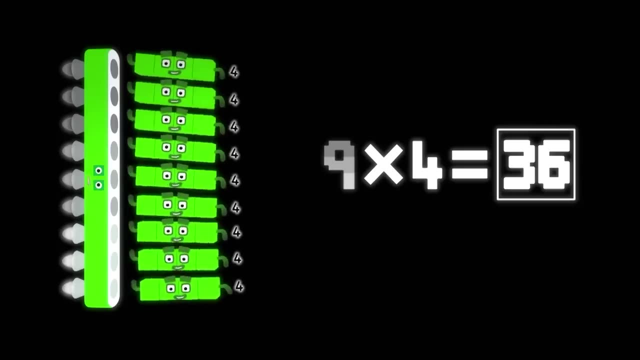 Five fours a twenty Six fours a twenty-four, Seven fours a twenty-eight, Eight fours a thirty-two, Nine fours a thirty-six And, when all the fours are in the mix, Ten fours a forty. Whoo. 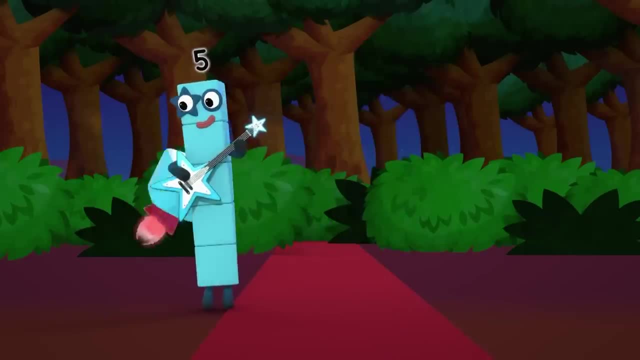 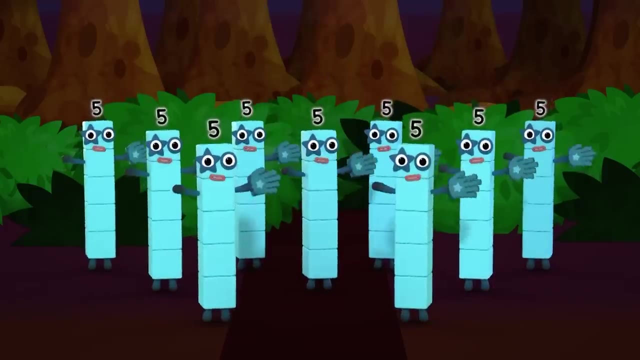 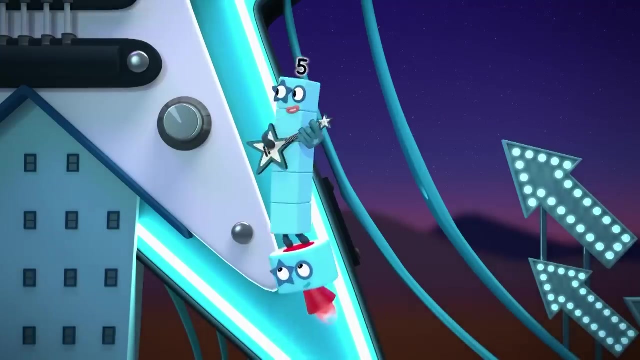 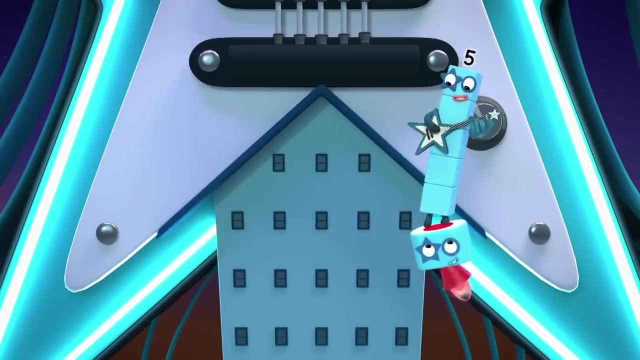 You've got talent, you've got drive and you never give up. It runs in the family, The family, The family of fives, High five, Let's rock, Crack it up, Plug in the cable. I'm the one and only five-time sable. 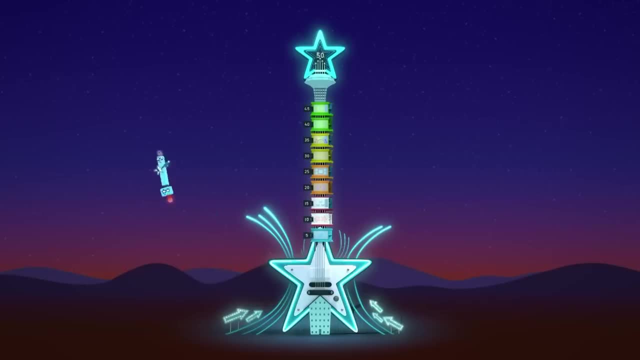 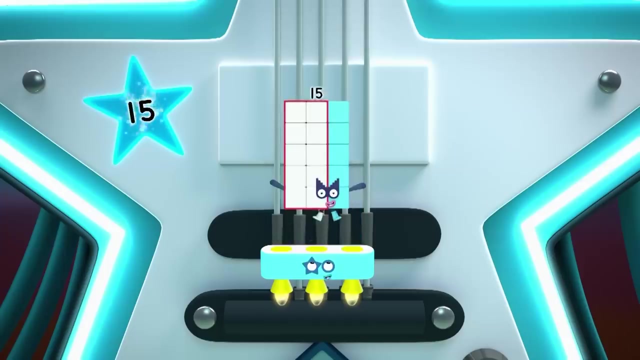 It's time to come alive And meet your heroes. Some of them end in five And some end in zero. One five is five. Two fives are ten. Three fives are fifteen. Trust me, you'll go far. Four fives are twenty. 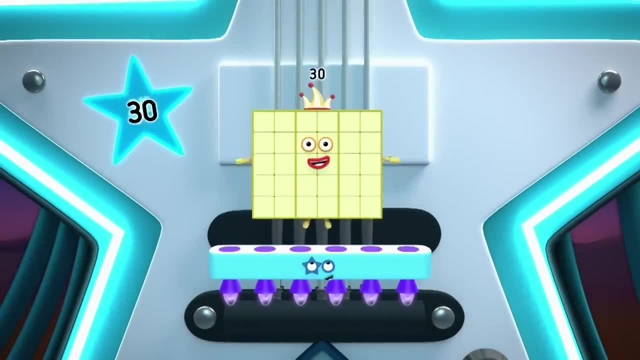 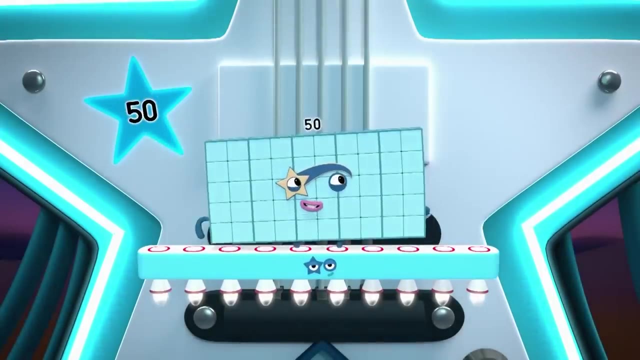 Five fives are twenty-five. Six fives are thirty. You know who you are. Seven fives are thirty-five. Eight fives are forty. Nine fives are forty-five. And here's the next big superstar: Ten fives are fifty. 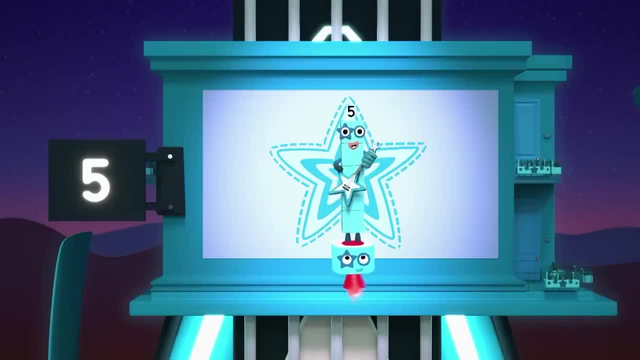 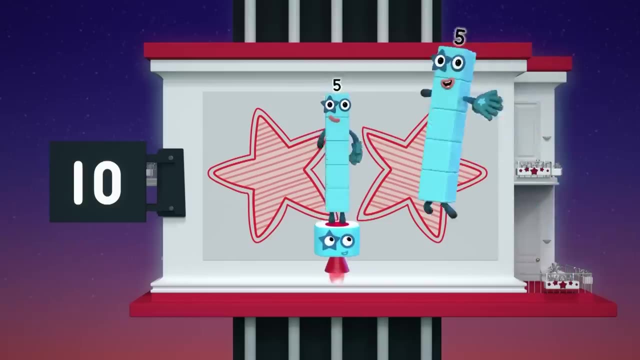 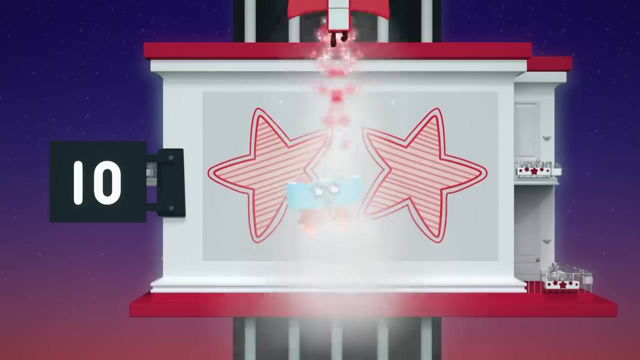 Take it to the top. One five will land her hands. She's the leader of the band. Five High five. Two fives can take a trip. They can make a rocket ship. Ten Lost all Cause I'm the five-times table. 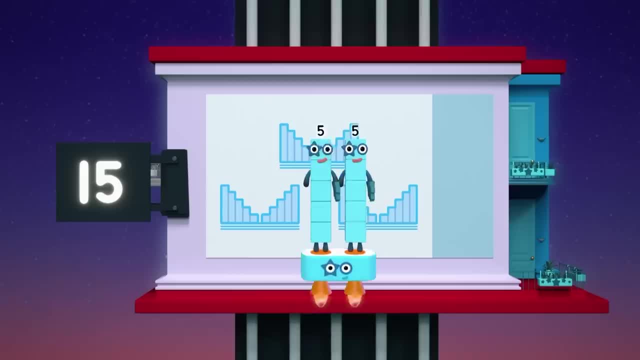 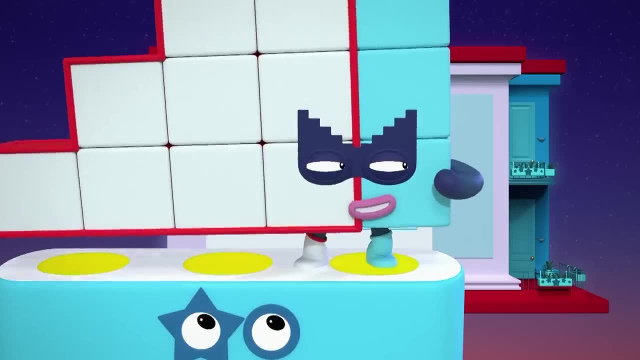 Start me up and we'll go up in fives. Three fives are slightly odd. They're a secret special squad. Fifteen Hush, hush, Slightly odd. Four fives make a great quartet, But you ain't seen nothing yet. 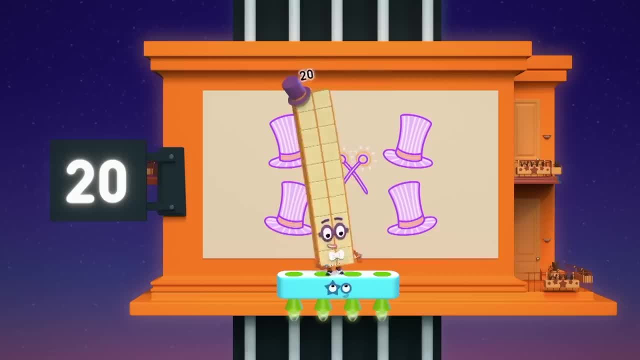 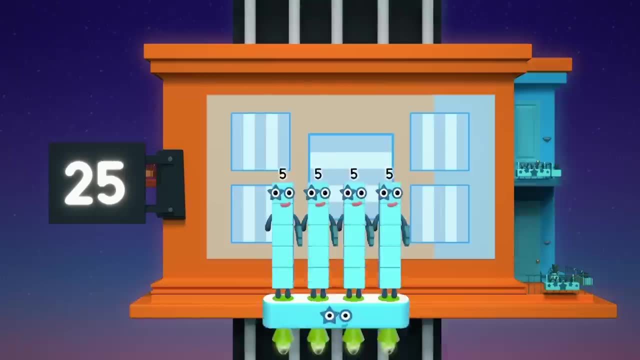 Twenty: Chop, chop, chop, chop, chop, chop. Cause I'm the five-times table, Start me up and we'll go up in fives. Five fives were half way there. Five fives make a great big square. Twenty-five: 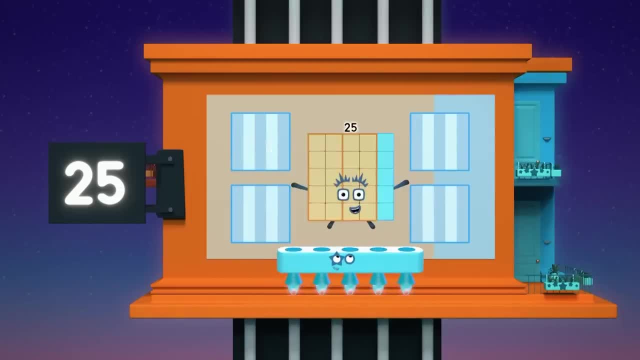 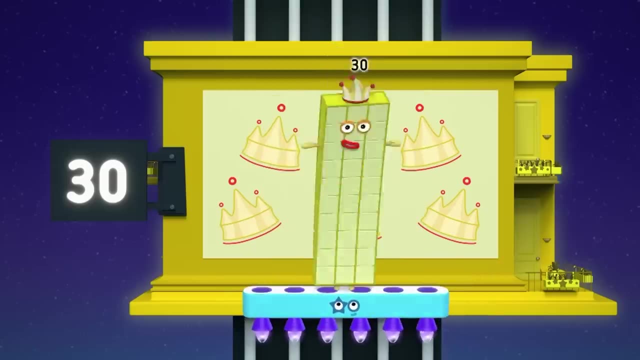 Square. Six fives are neatly stacked. Six fives are a circus act. Thirty, The greatest show in Numberland. Seven fives never come unstuck. Seven fives have sevens luck. Thirty-five, She's the five-times table. 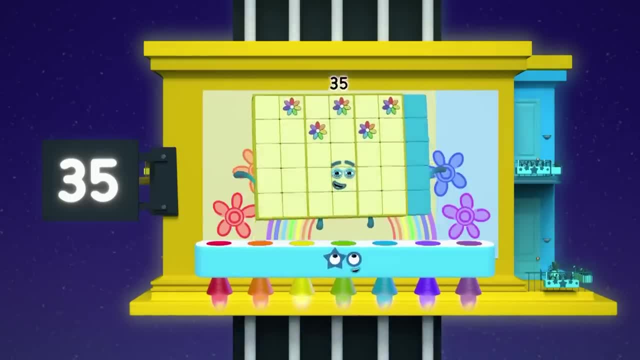 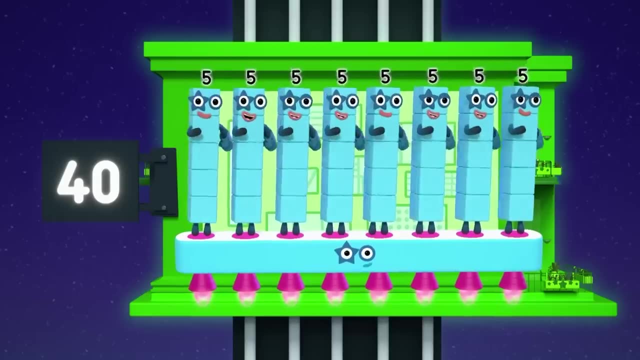 Eight fives will get them bigger. They make a great show in Numberland. Seven fives never come unstuck. Seven fives have sevens luck. Thirty-five, They make an impressive figure. Forty, She's the five-times table. 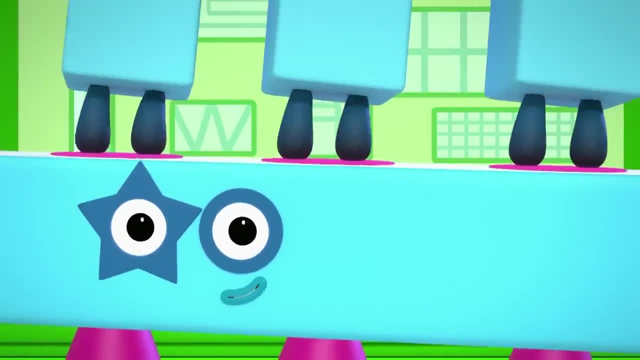 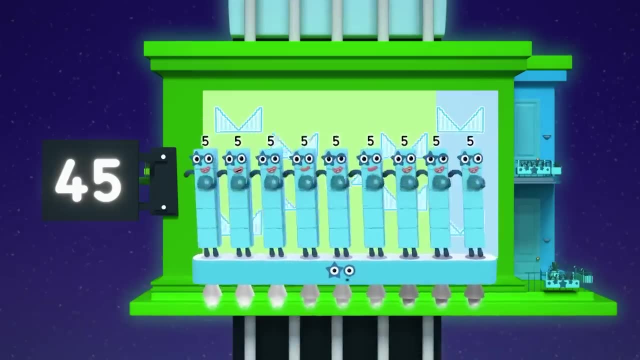 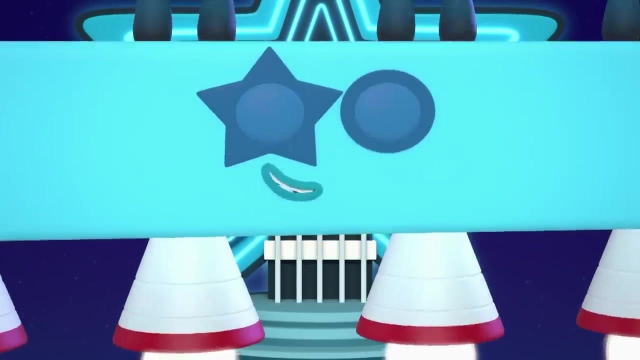 Cause I'm the five-times table. Start me up and we'll go up in fives. Nine fives to step up the pace And take you to a higher place. Forty-five, Ten fives with a gold guitar. Ten fives make a superstar. 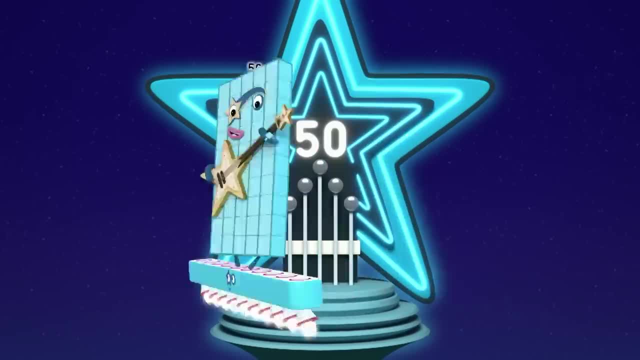 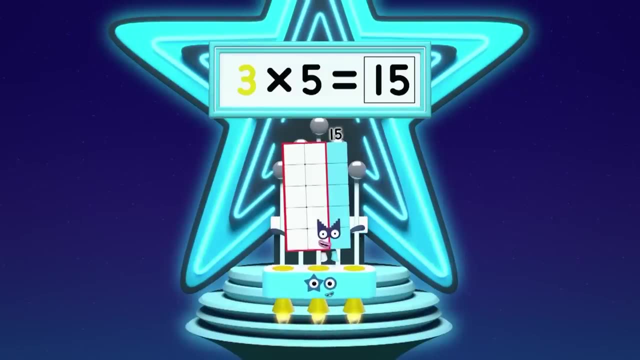 Fifty High. fifty One five is ten. One five is five. Two fives are ten. Three fives are fifteen. Trust me, you'll go far. Four fives are twenty. Five fives are twenty-five. Six fives are thirty. 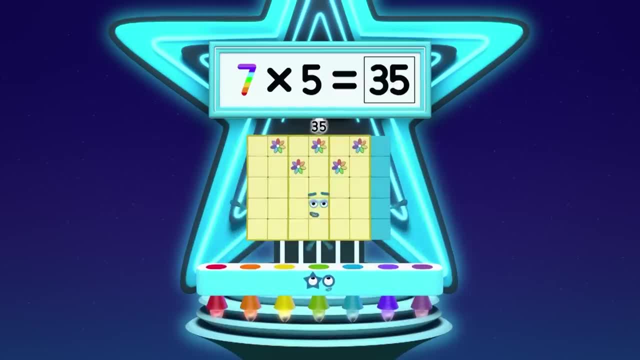 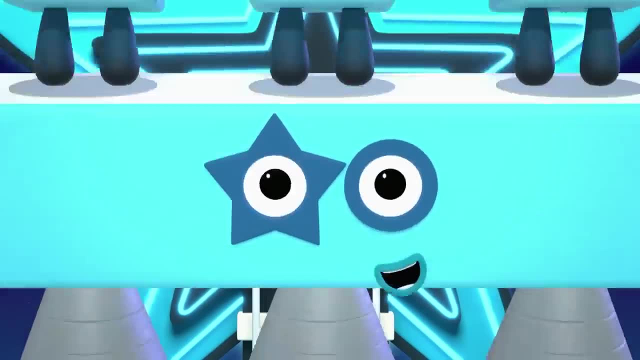 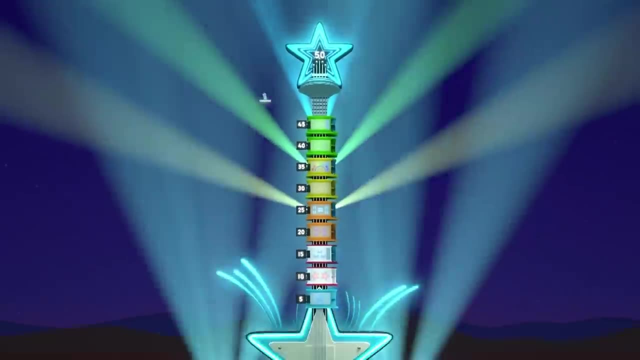 You know who we are. Seven fives are thirty-five. Eight fives are forty. Nine fives are forty-five. Here's the next big superstar. Ten fives are fifty. Guitar solo Sideway. One five is five. Two fives are ten. 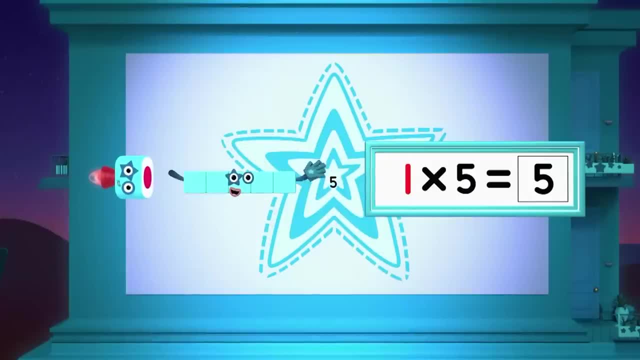 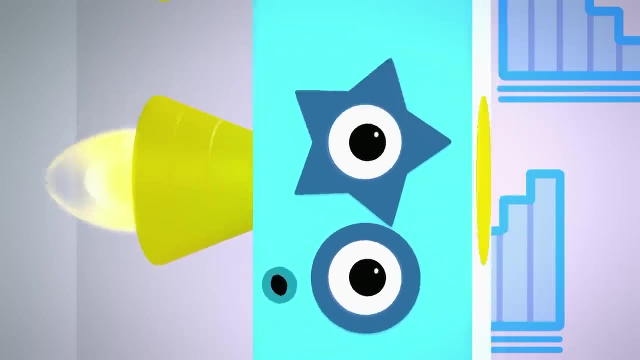 Three fives are fifteen. Trust me, you'll go far. Four fives are twenty Five fives are twenty-five. Six fives are thirty. You know who we are. Seven fives are thirty-five. Eight fives are forty. 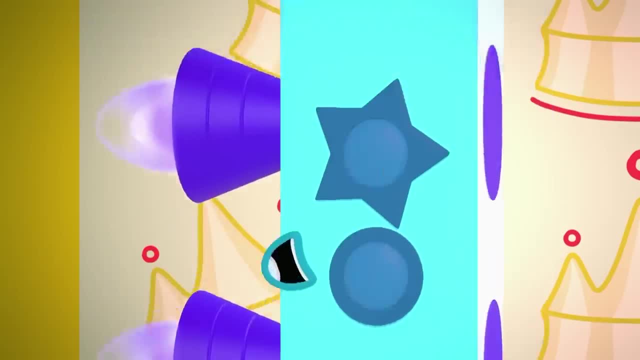 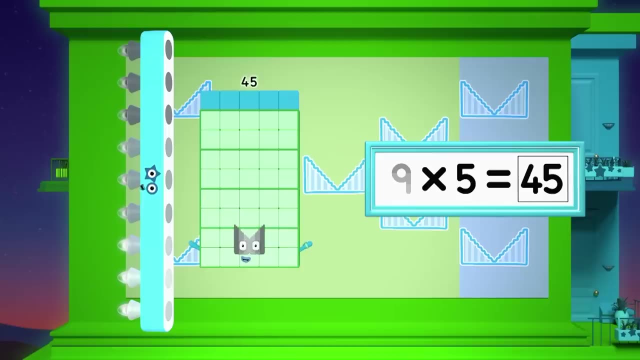 Five fives are twenty-five. Six fives are thirty. You know who we are. Nine fives are forty-five. Eight fives are forty. Nine fives are forty-five. One more time. let's take it to the top. 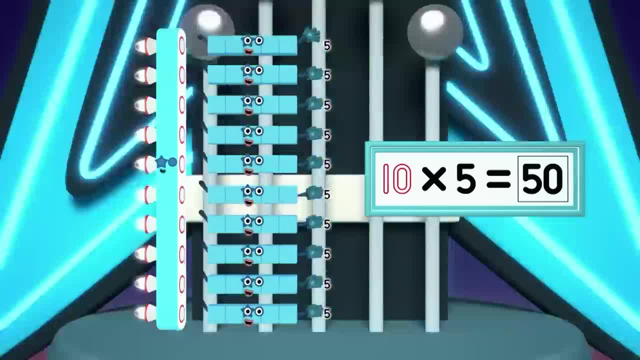 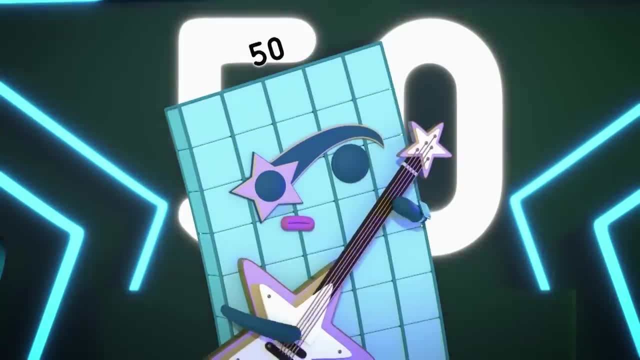 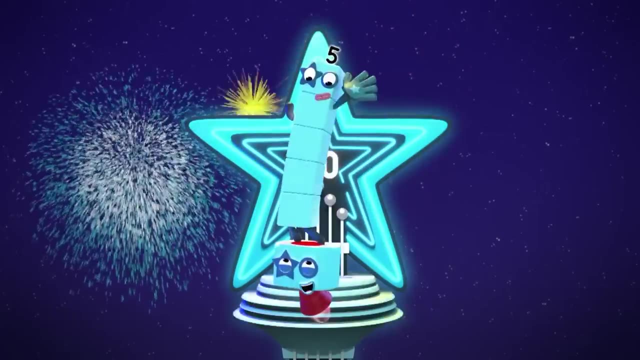 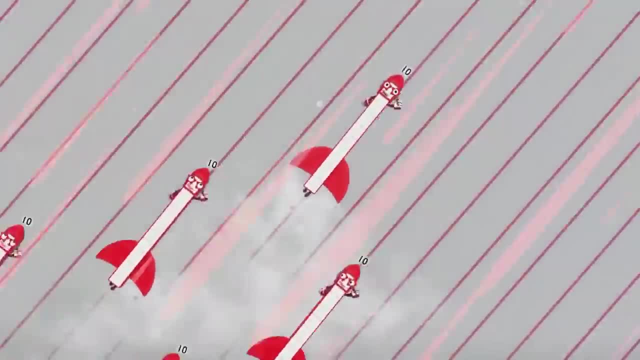 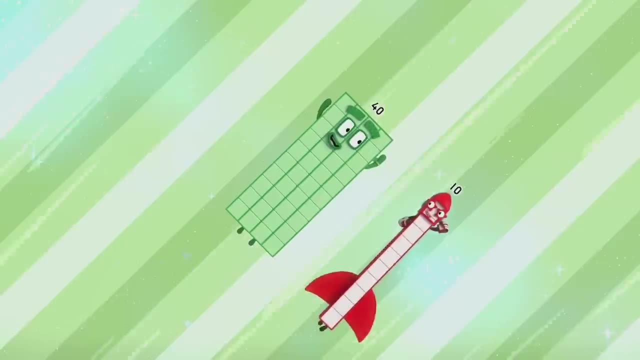 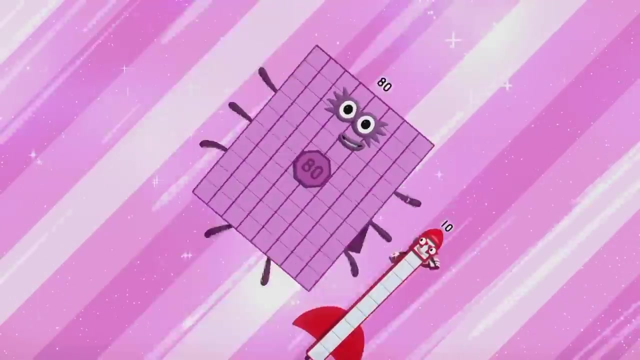 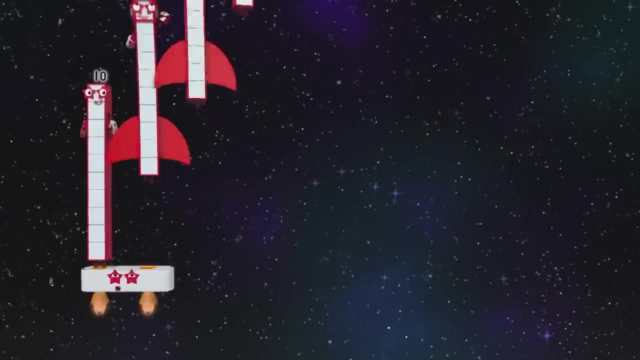 Rocket rescuers, come as soon as you are able. Ten, Twenty, Thirty, Forty, Fifty, Sixty, Seventy, Eighty, Ninety, One hundred Heroes with zeros. One ten is ten. Two tens are twenty. 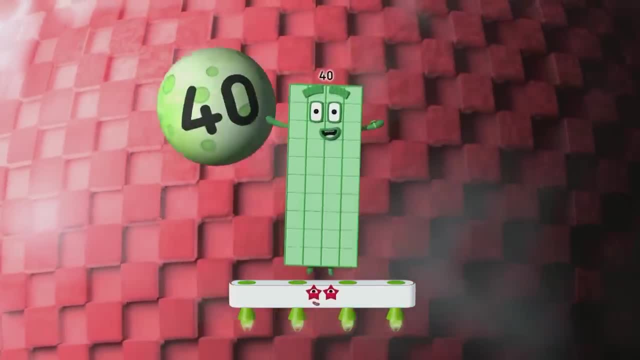 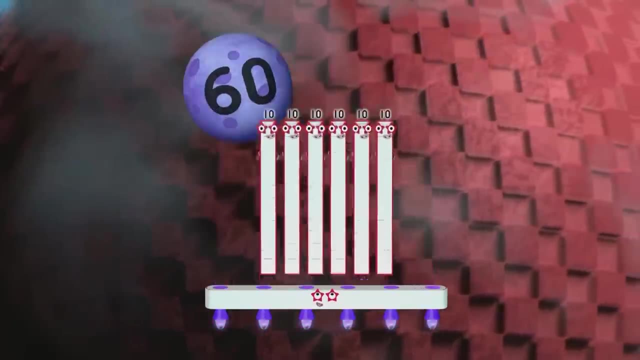 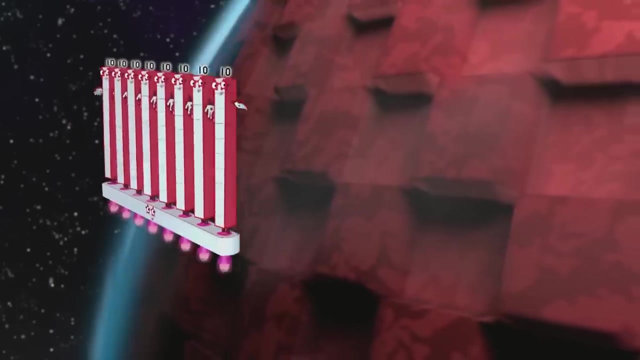 Three tens are thirty. Four tens are forty. Heroes with zeros. Heroes with zeros. Five tens are fifty. Six tens are sixty. Seven tens are seventy. Eight tens are eighty. Heroes with zeros. Heroes with zeros. Nine tens are ninety. 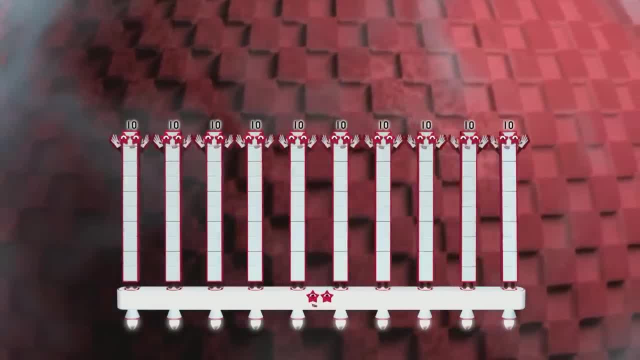 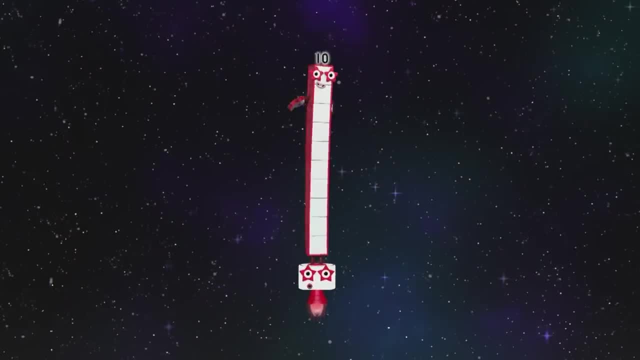 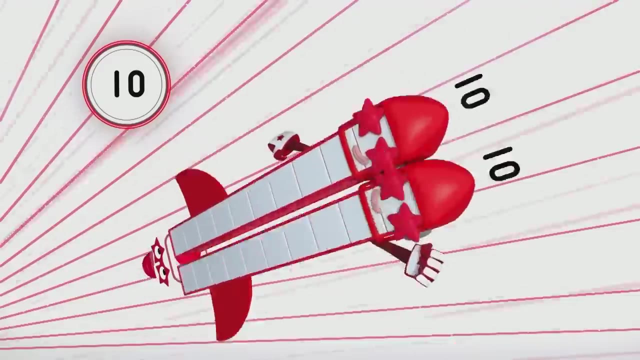 And ten, tens are one hundred. Heroes with zeros. Heroes with zeros. Heroes with zeros. Ten is the original. Ten is the original. She'll get us underway. Rocket to the rescue. Twenty has a double boost. Twenty has a double boost. 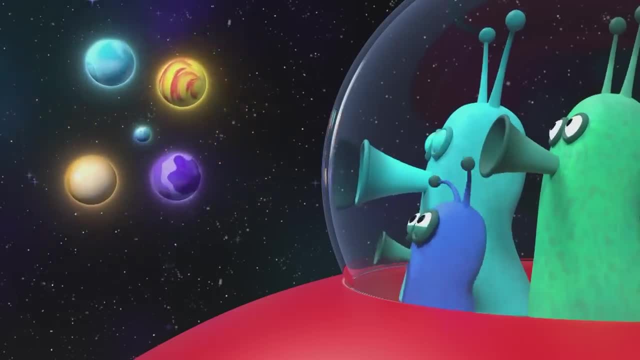 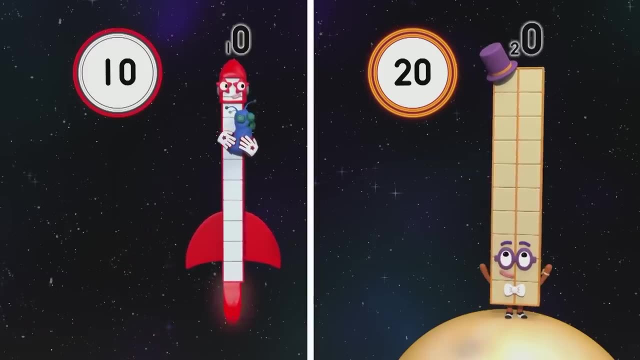 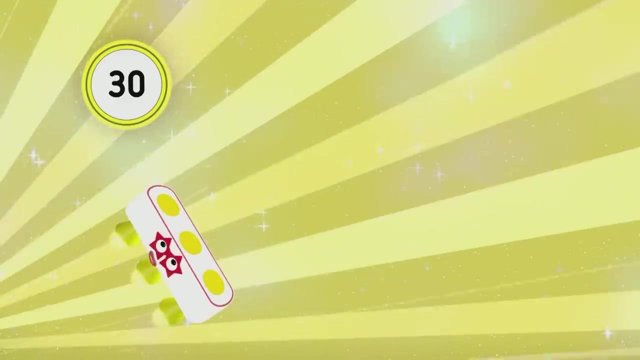 He can dance all day Interterrestrial tango. They know what their zeros are. They know what their zeros are: One, ten, Two tens And nothing more. Heroes with zeros. Heroes with zeros. Fifty juggles, asteroids. You ain't seen nothing yet. 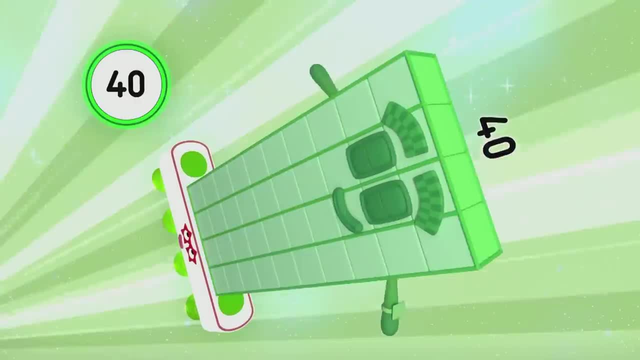 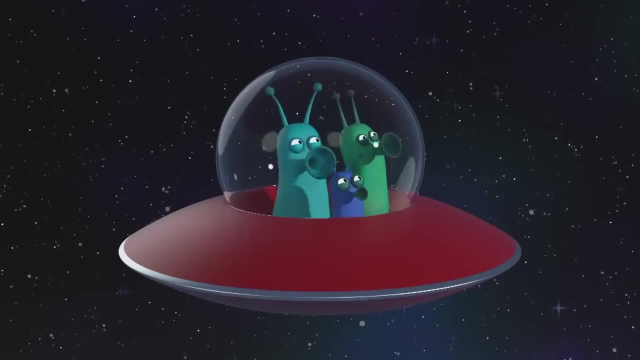 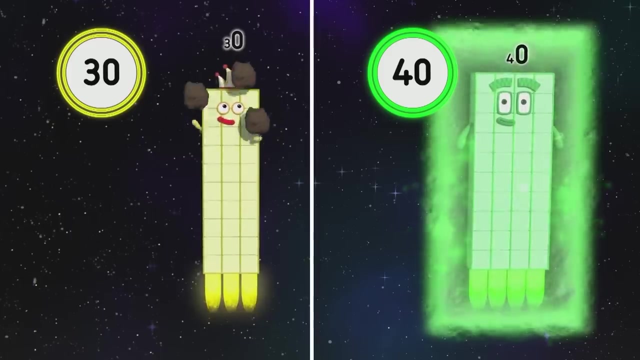 The greatest show in space. Forty is a rectangle With an oblong pit, Intergalactic oblongs. Three, They know what their zeros for? Three tens, Four tens And nothing more. Heroes with zeros. Fifty is a superstar. 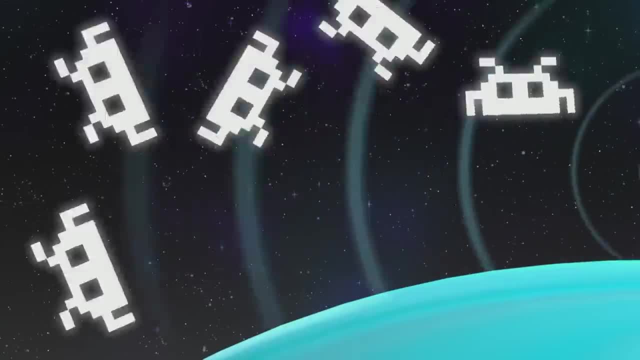 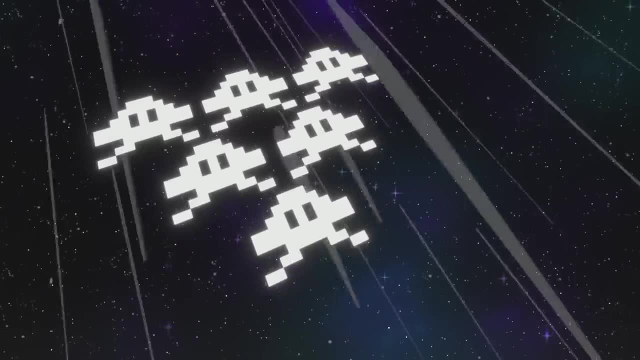 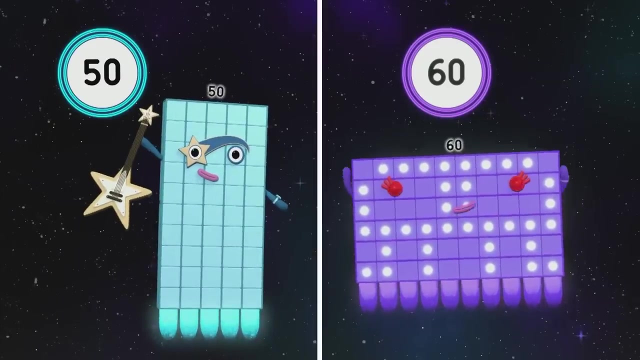 Who works the satellites Solar overdrive? Yay Sixty is a super gamer. She can light the lights Galactic game over. Yay Five tens, Six tens Heroes with zeros. Seventy has luck times. ten Launching from the dock. 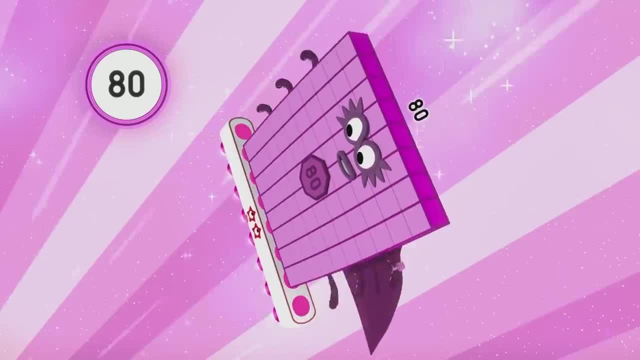 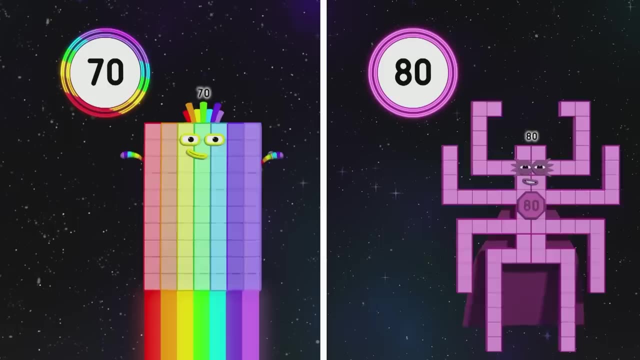 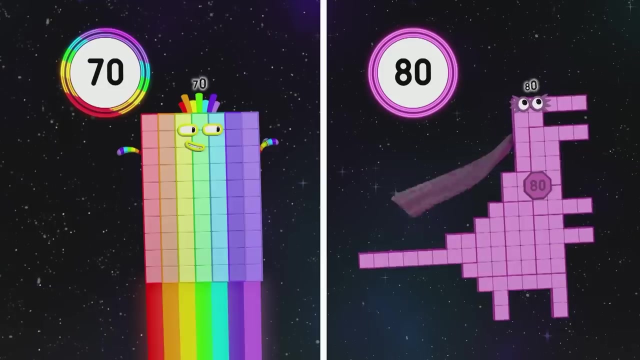 Space rainbow. Oh, Eighty needs no luck at all, He's super octoblock. Octoblocks, find octoblocks. They know what their zeros for? Seven, tens, Eight, tens And nothing more. Heroes with zeros. Ninety knows a trick or two. 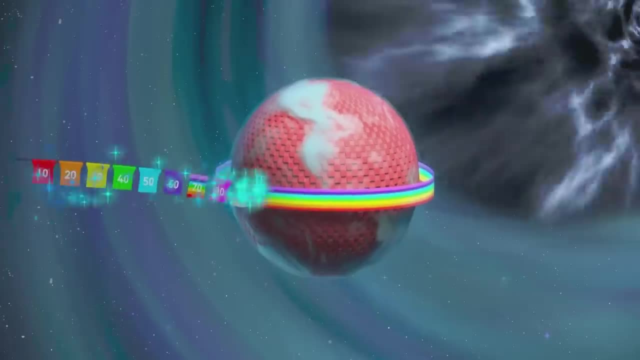 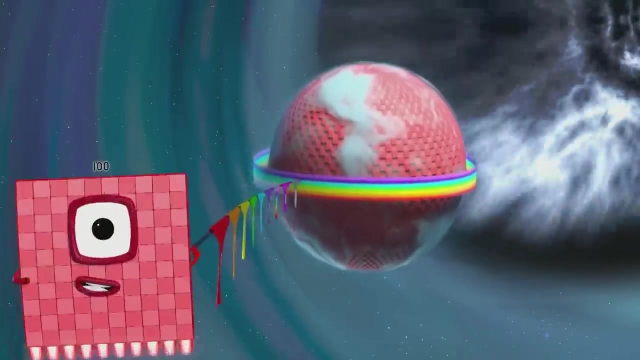 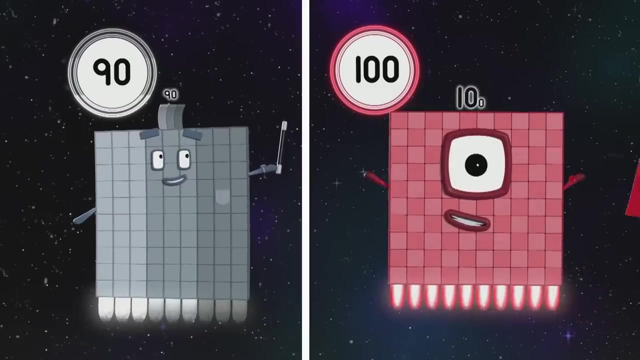 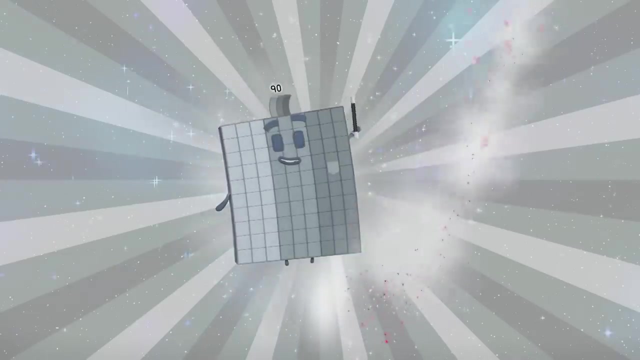 He will heed the call: Abracadabra. And now let's meet. one hundred, The greatest of them all. Hero with two zeros. Nine tens, Ten tens. Heroes with zeros One hundred Ninety Eighty Seventy. 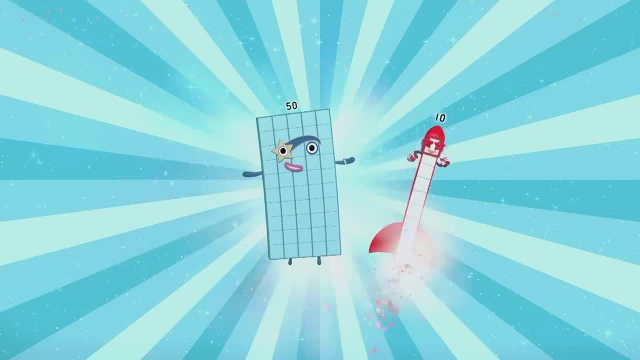 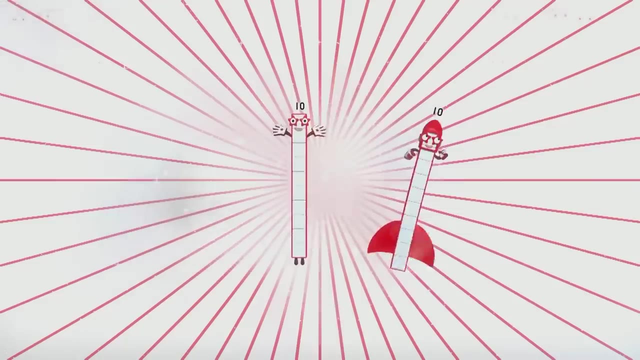 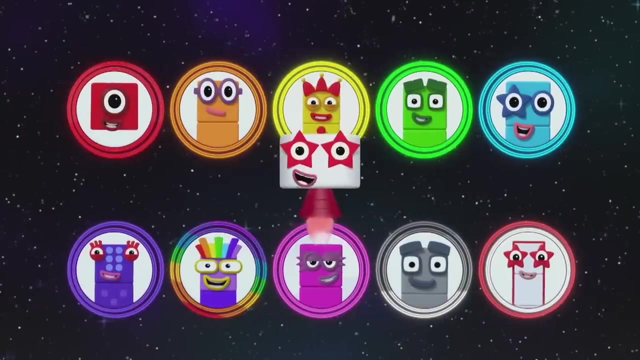 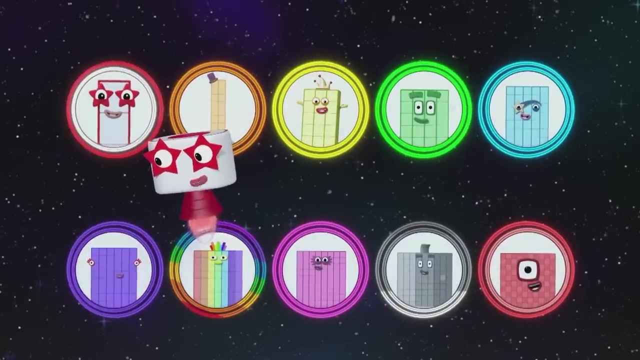 Sixty, Fifty, Forty, Thirty, Twenty, Ten. If you can count to ten, Then you know the ten times table. You just need an extra zero To make your favorite hero. One ten is ten, Two tens are twenty. 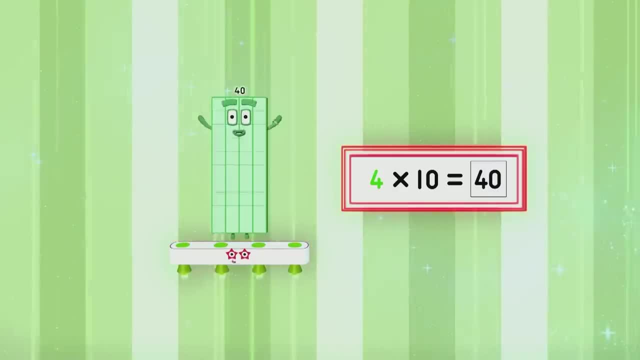 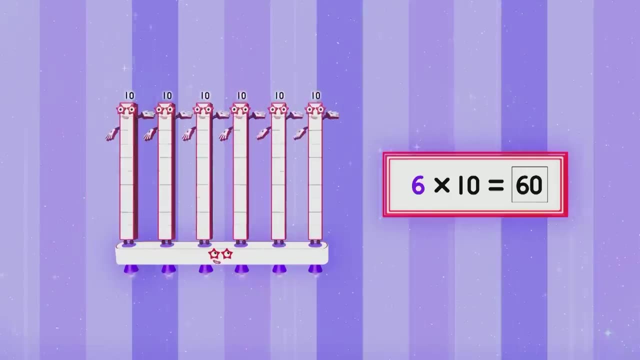 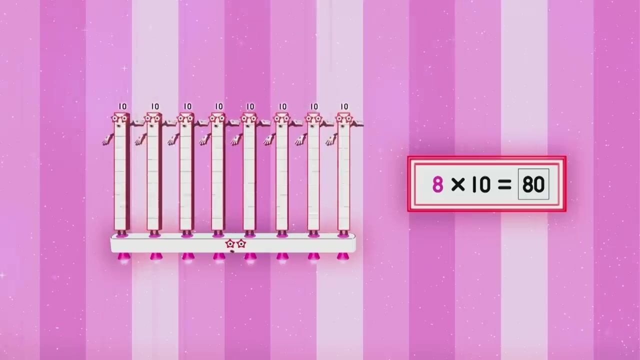 Three tens are thirty. Four tens are forty. Heroes with zeros. Heroes with zeros. Five tens are fifty. Six tens are sixty. Seven tens are seventeen. Eight tens are eighteen. Heroes with zeros. Heroes with zeros. Nine tens are ninety. 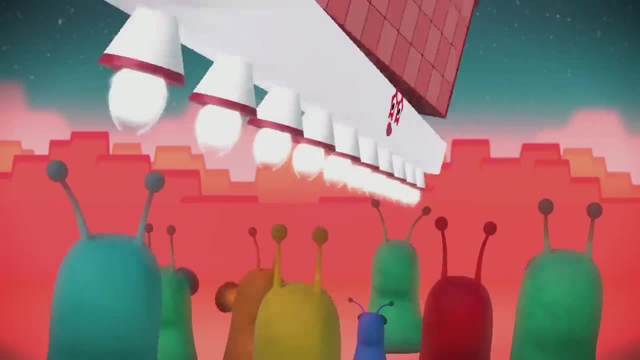 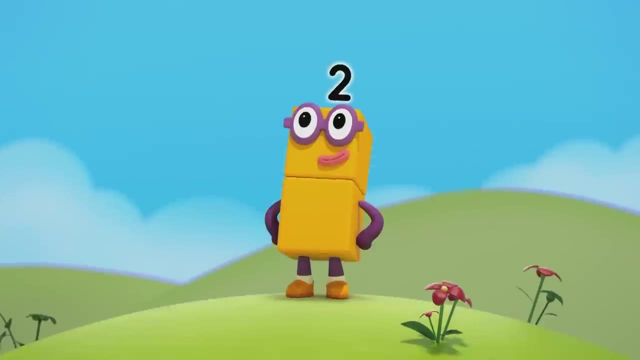 And ten tens are one hundred. Heroes with zeros. Heroes with zeros. Heroes with zeros. Hey, Hurry up Two. If we don't catch the train, we might miss the talent show. But it's such a lovely day, Just give me a second. 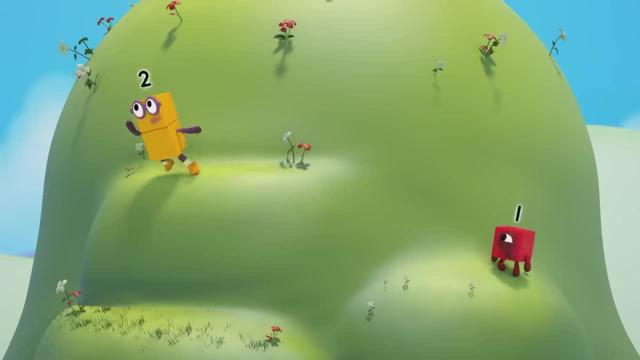 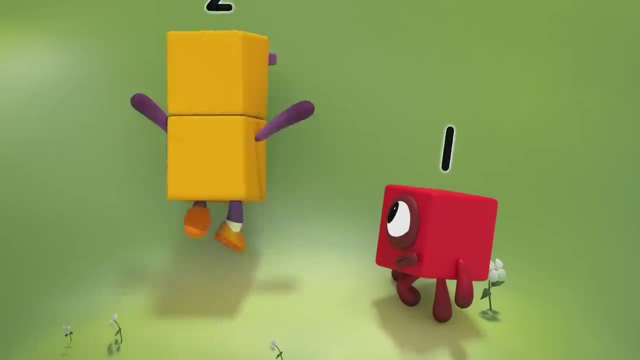 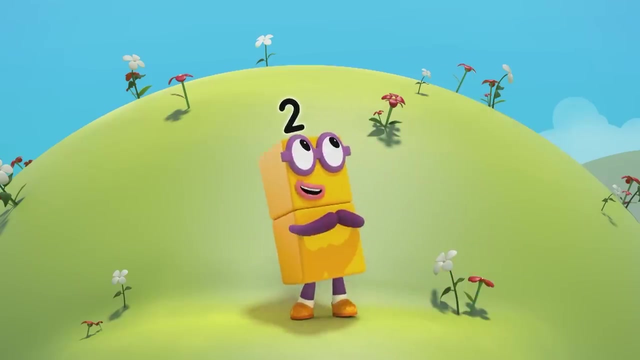 A second. How long is a second? A moment to start, A beat of the heart, A step on the way, A second Stop for a second. The sun is up, high, Straight up in the sky. Today is my day. 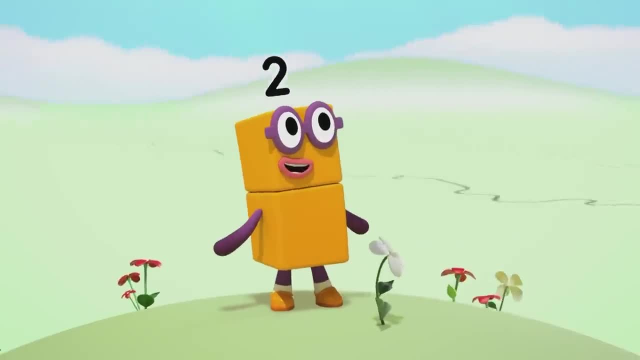 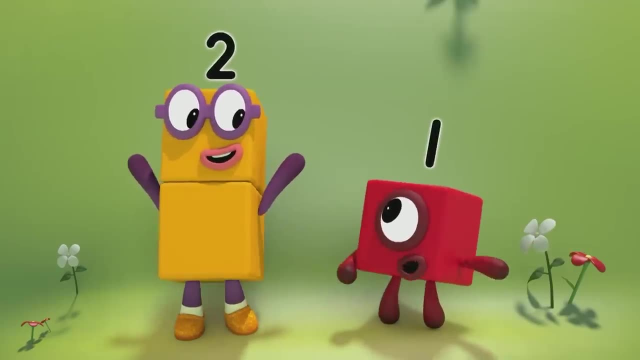 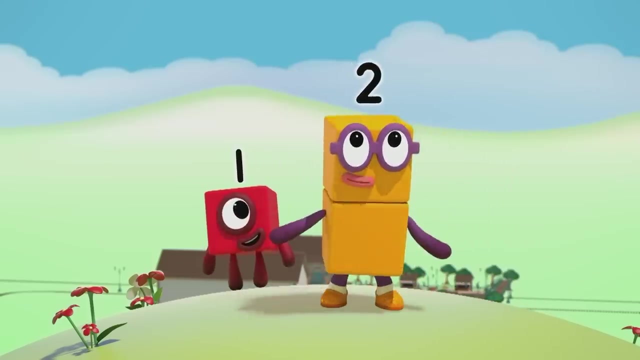 We'll ride the train to the edge of the sea, Where we'll dance together, My best friend and me. But for now We have to go A moment. I'll only take a moment. Today is too fine, So I'll take my time for a moment. 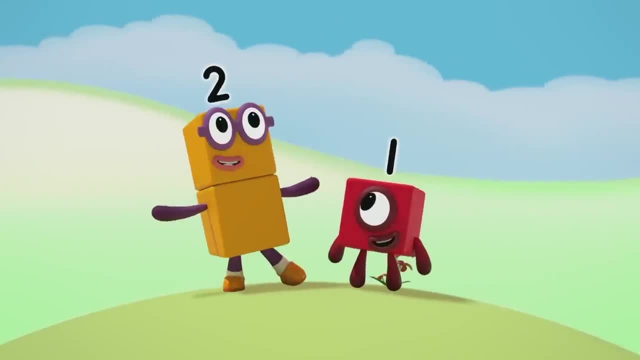 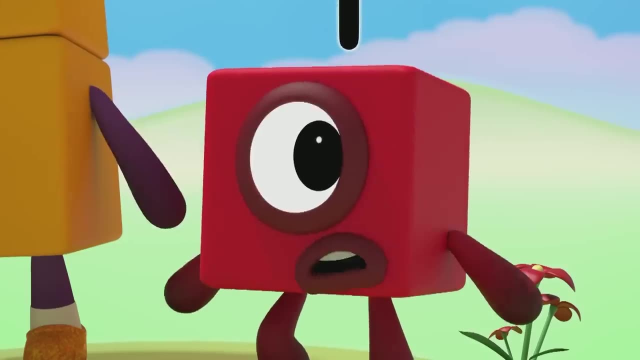 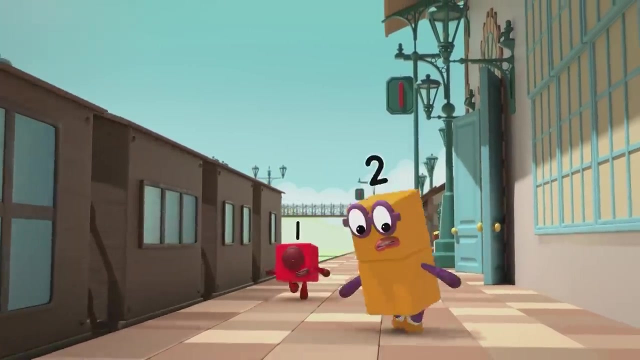 For time is a train on a one way track And this is a moment I won't get back. No, It's nearly one o'clock. We have to catch our train. Oh no, If I can stop the clock, Maybe I can stop the train. 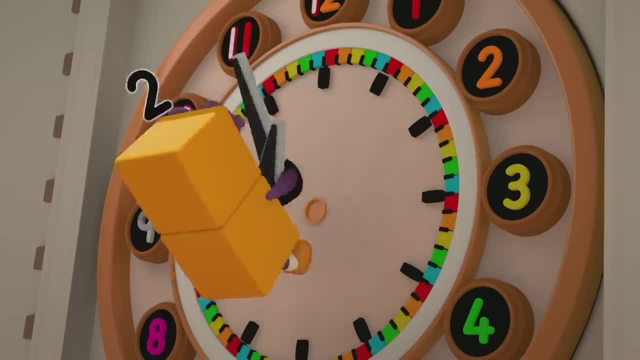 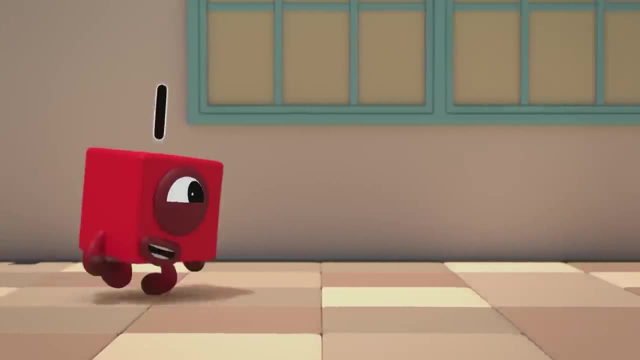 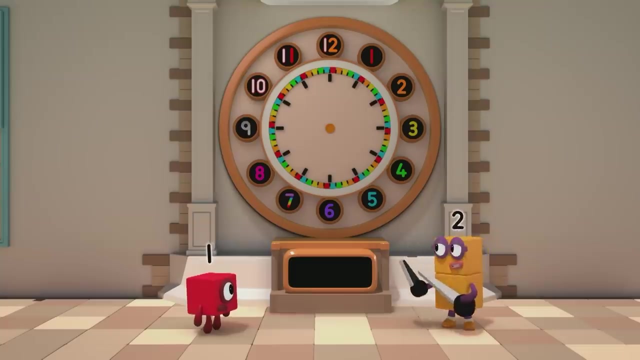 That's not how it works. We missed the train. Is there another one we can catch? Maybe, But with the clock broken, We can't tell when any train leaves. Well, I broke it, So I should fix it. There's these two pointy things. 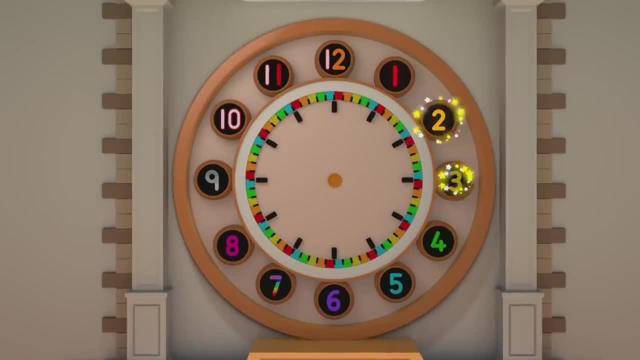 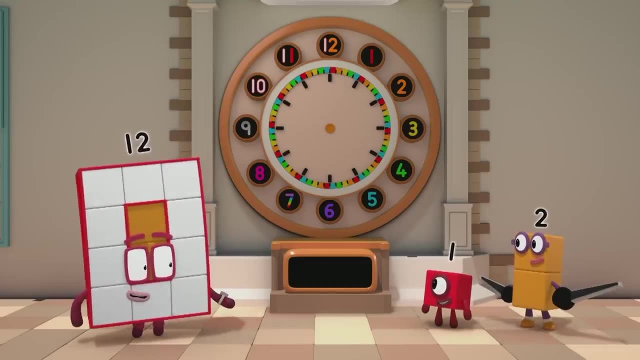 And lots of numbers, Starting at one And going all the way around to twelve, Did someone call? Looks like you could use a hand learning how to tell the time. After all, you can't be on time if you don't know what time it is. 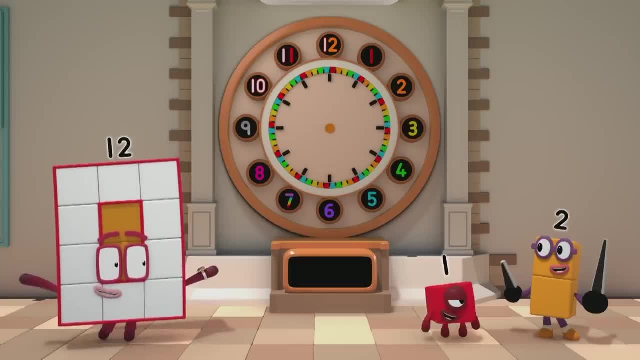 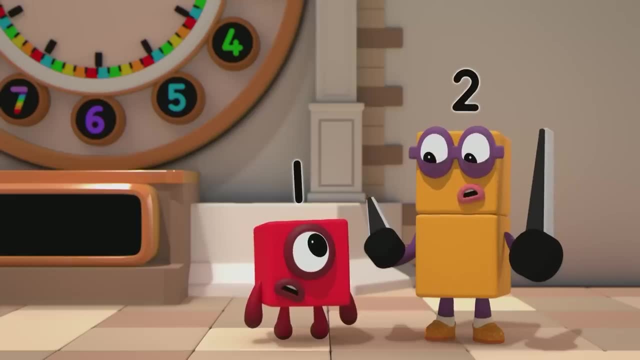 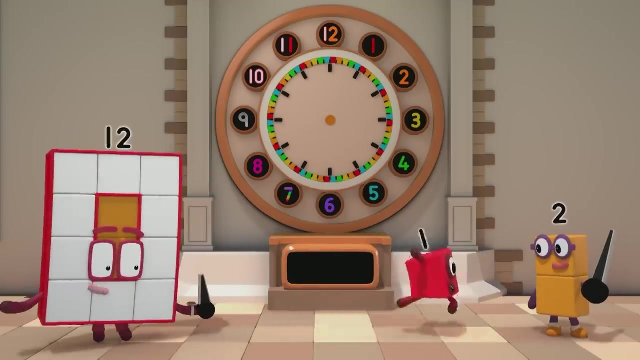 Thanks twelve. Where do I start? Well, I said you could use a hand. In fact you can use two: The two hands of the clock. There's two hands. There's a big hand And a little one And, as we know, 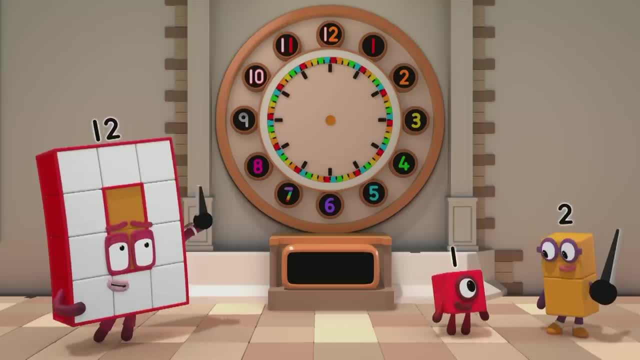 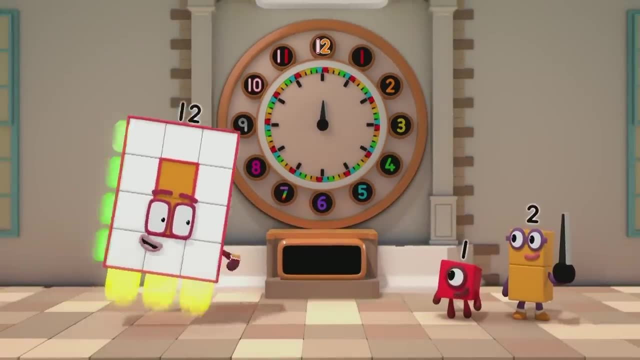 little ones can be very important. The little hand is called the hour hand. It shows you what hour it is. Like this: It starts at full height And moves round to the right, Like the sun in the sky at midday. Like the sun, it won't stop. 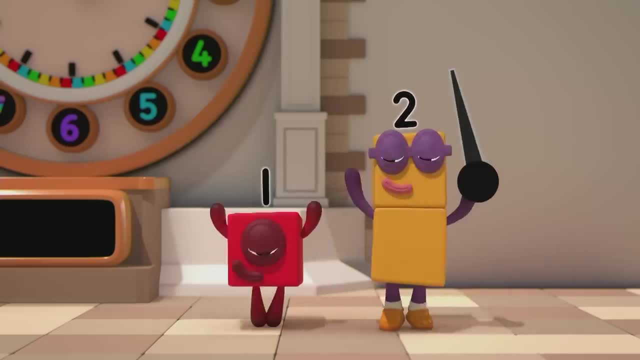 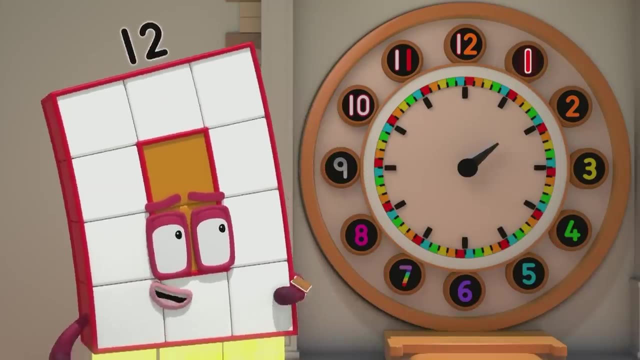 As it moves round the clock, And we count every hour on the way, And we count every hour on the way, And now it's one and a bit. One and a bit. It's one and a bit, till it's two. Two and a bit, Two and a bit. 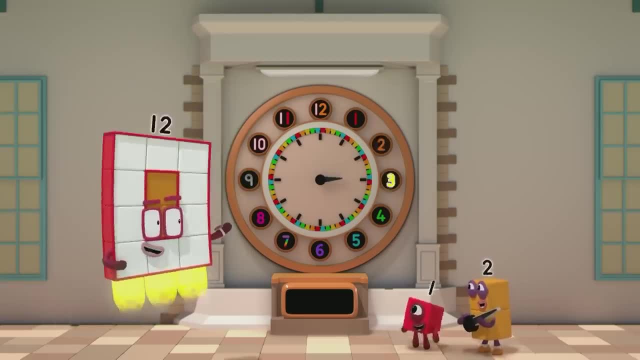 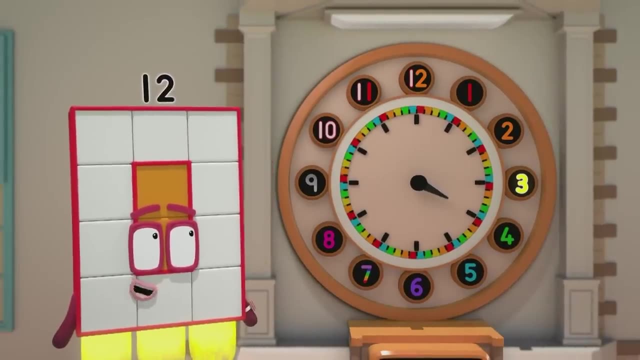 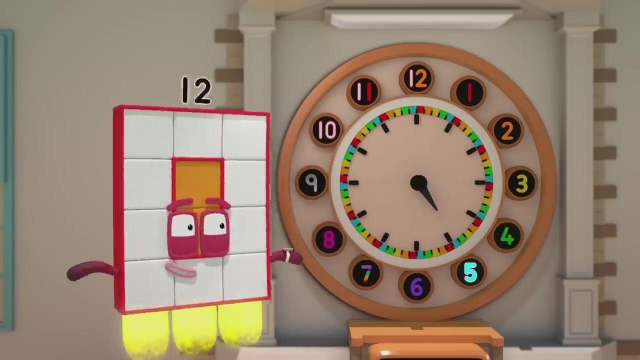 It really is that easy to do. Three and a bit. Three and a bit The hour hand is steady, not fast, And now it's four and a bit. Four and a bit The hour is the last big number that you passed. Five and a bit. Five and a bit. 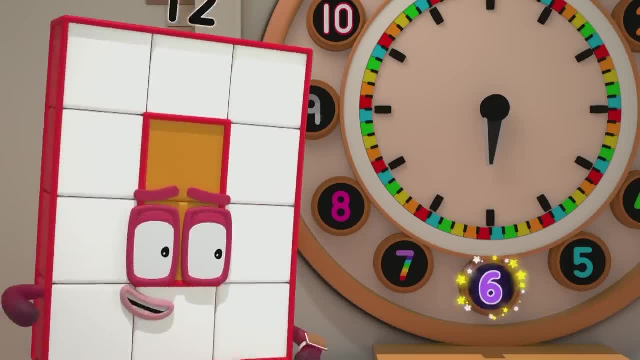 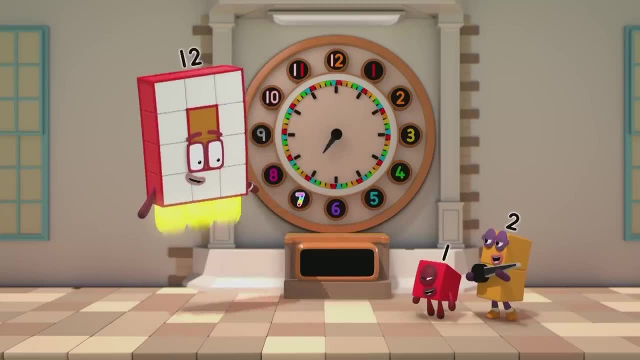 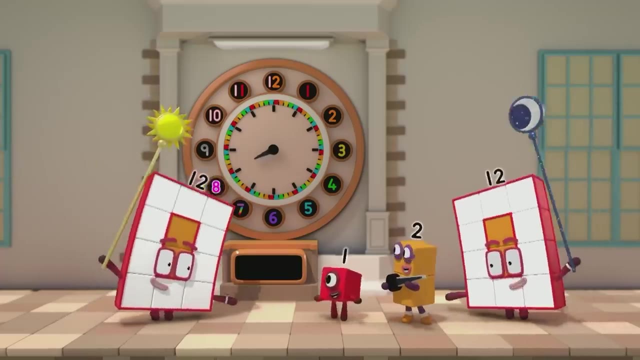 It's a short hand for telling the time. Six and a bit. Six and a bit, Halfway round and starting to climb. Seven and a bit. Seven and a bit As the day moves on towards night. As the day moves on towards night, Eight and a bit. Eight and a bit. 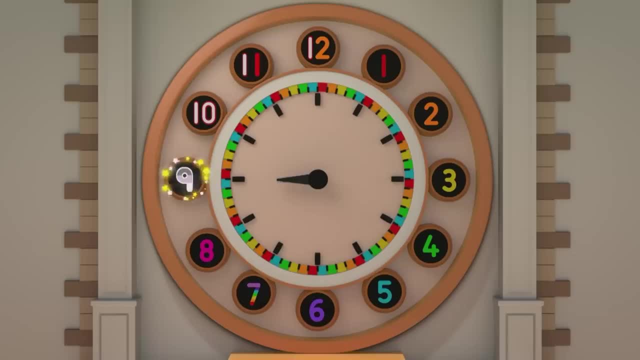 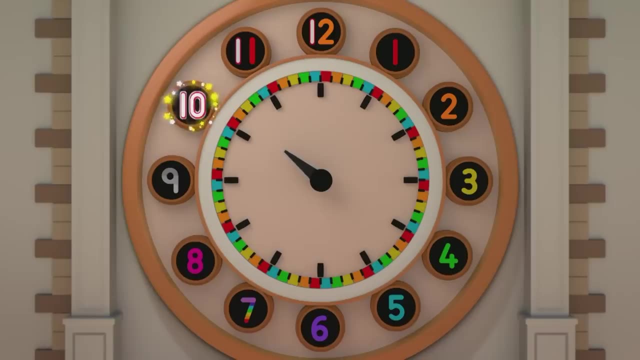 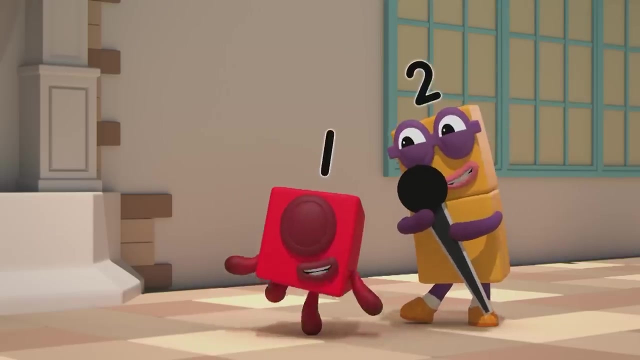 You can tell the time on sight. Now it's nine and a bit, Nine and a bit All together. call up The hour: Ten and a bit, Ten and a bit. Tell the time. now you have a power. Eleven and a bit, Eleven and a bit, All the way around. we have fun. 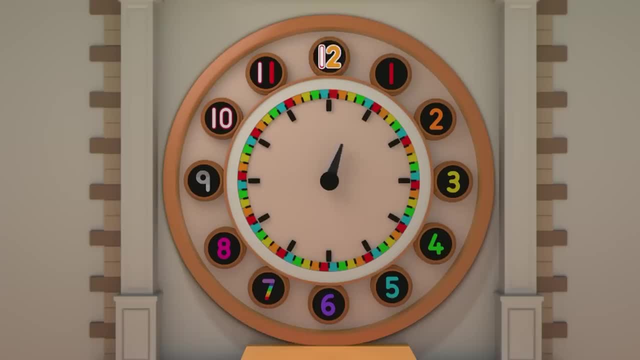 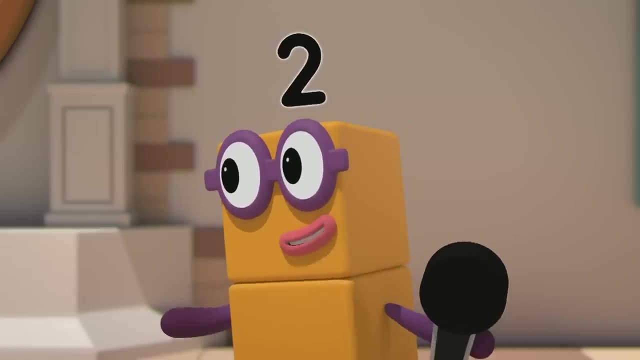 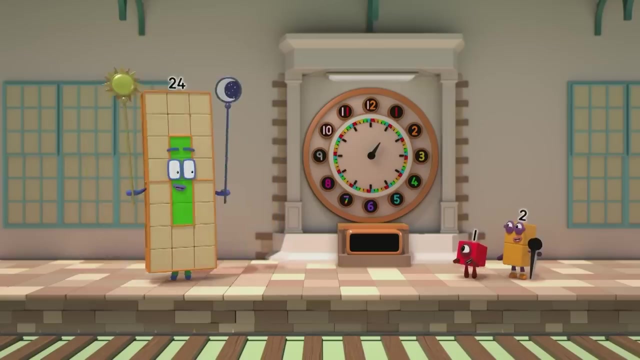 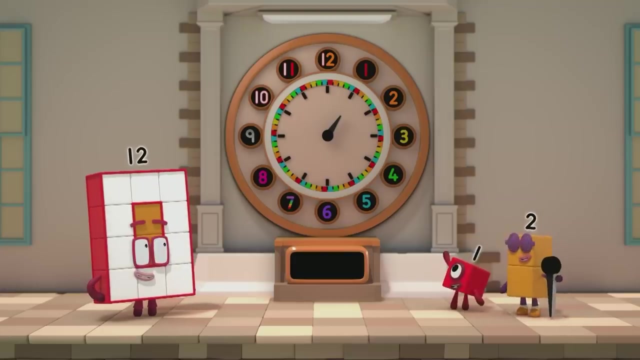 Twelve and a bit. Twelve and a bit And a bit more, And we're back to one. Thanks, Twelve And Twelve. You're welcome. We could keep this up all day, Twenty four hours a day. So the hour hand is saying that the time now is one And a bit. 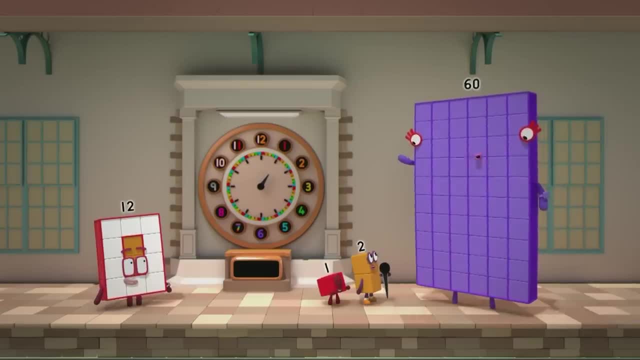 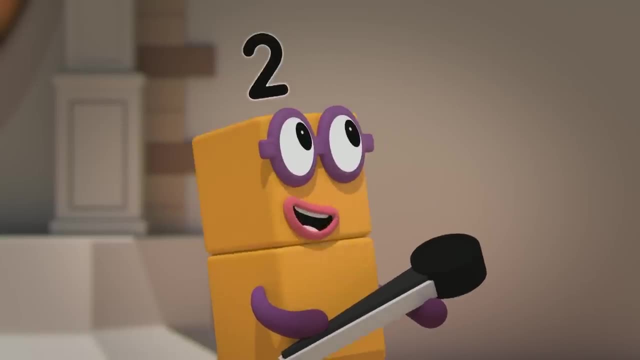 And that bit is the number of minutes, Which is what the big hand counts. Which is what the big hand counts, Hello, Sixty. So the big hand is the minute hand. So the big hand is the minute hand. Yes, and the big thing to remember is that Sixty is. 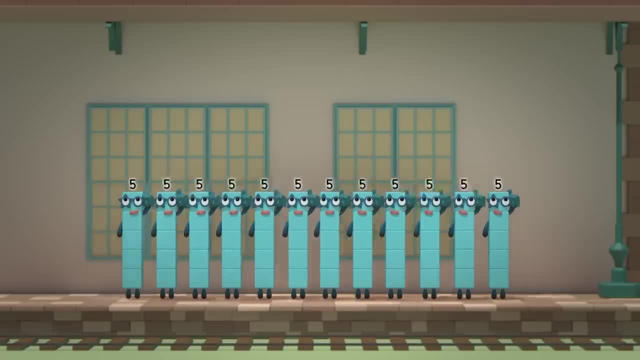 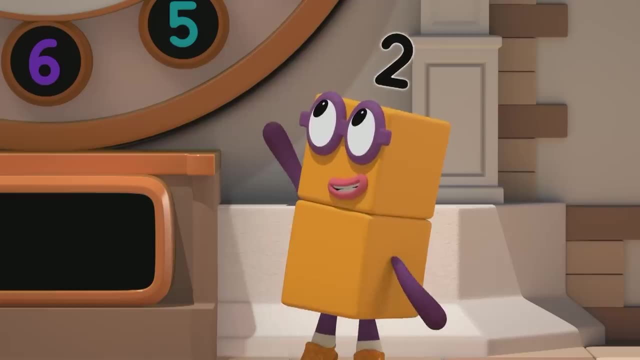 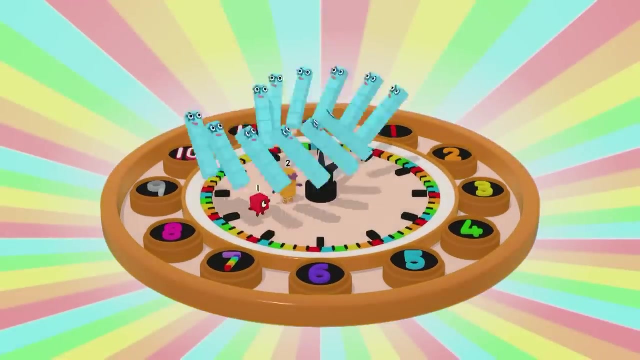 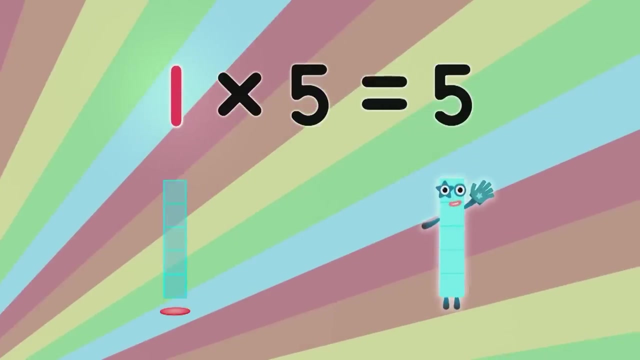 Twelve lots a day of five. roll out the big band to explain the big hand. look close at the clock. you'll see between every number are five little marks. so come along and count them with me. one minute, two minutes, three, four, five. one lot of five is five. then here come five more and the big 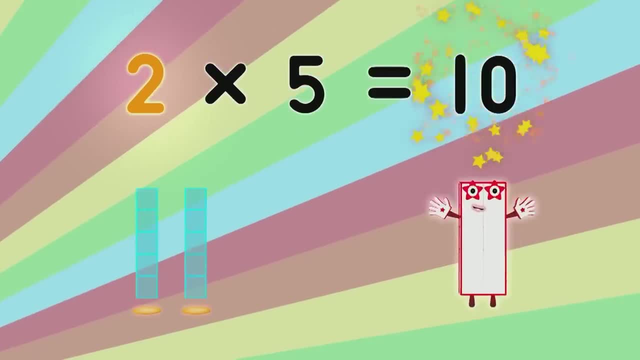 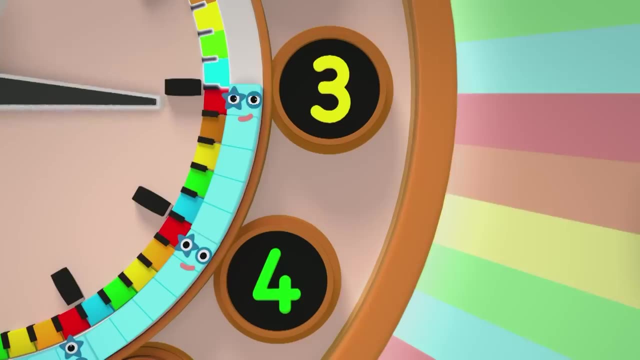 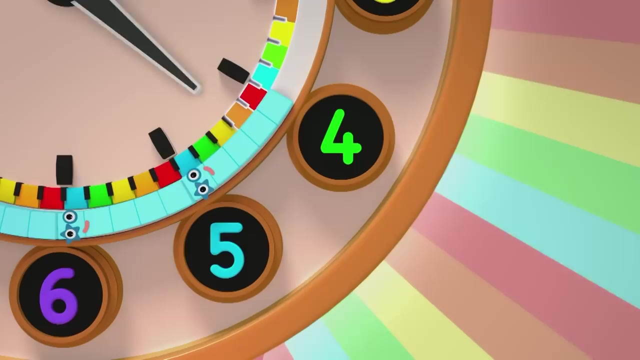 hand arrives at two lots of five, ten, ten minutes. as we reach number three, it's easy to see three, lots of five or fifteen. the secret is counting in fives, that's the key. four, lots of five or twenty. what's the minute hand dots? is the minutes advance? five, lots of five, twenty five- you can work out the. 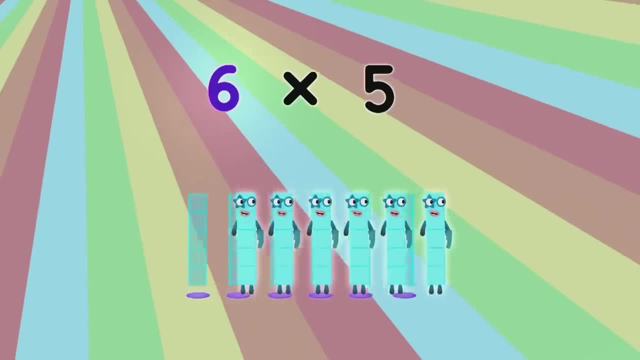 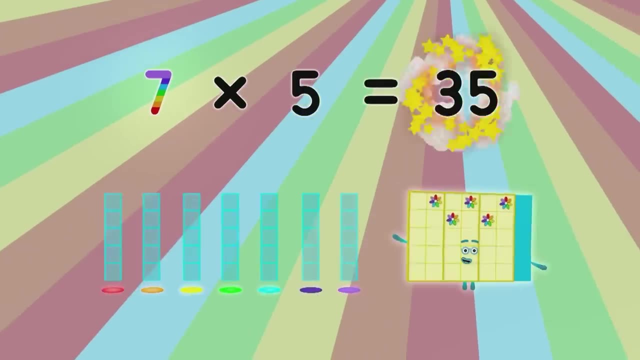 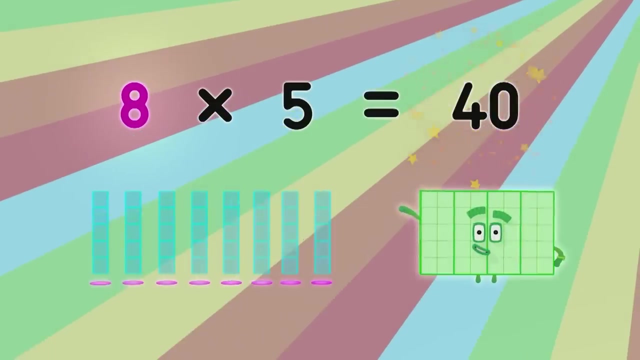 minutes. you need, at a glance, six lots of five or thirty- now the hour's half past, So we move up at last. Seven lots of fiber, Thirty-five, Counting in five so you can work it out fast- Eight lots of fiber, Forty. Keep on and keep going. there's no time for slowing. 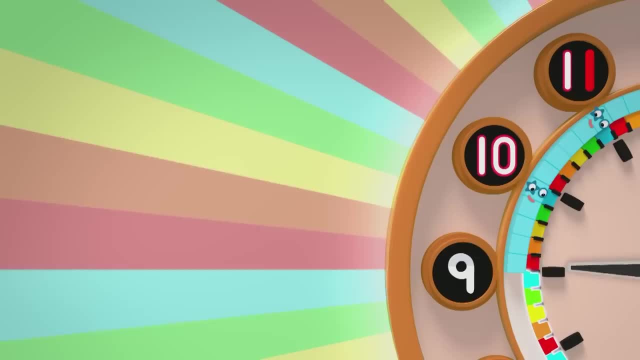 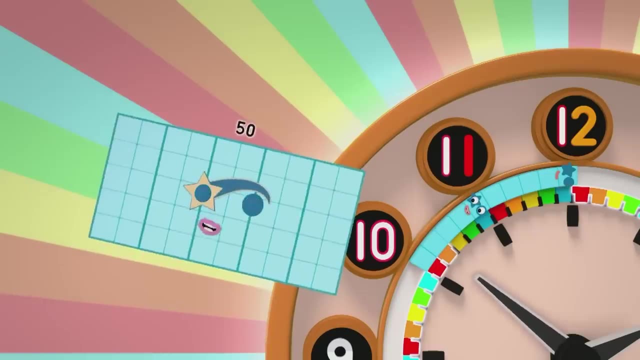 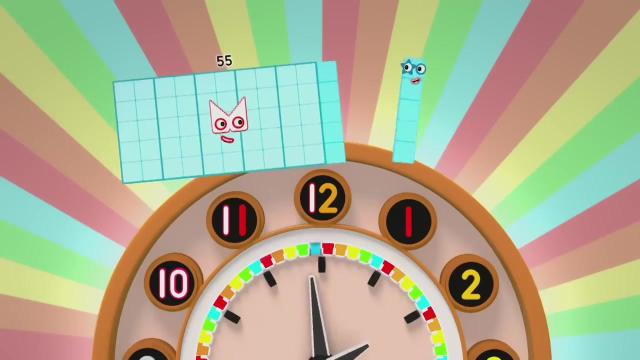 Nine: lots of five. Forty-five, Five at a time's- how these numbers are growing. Ten: lots of fiber. Fifty, Come on now and rock all the way round this clock. Eleven: lots of five. Fifty-five At sixty. we stop cause we're back to the top. Then we start again, all over from zero. 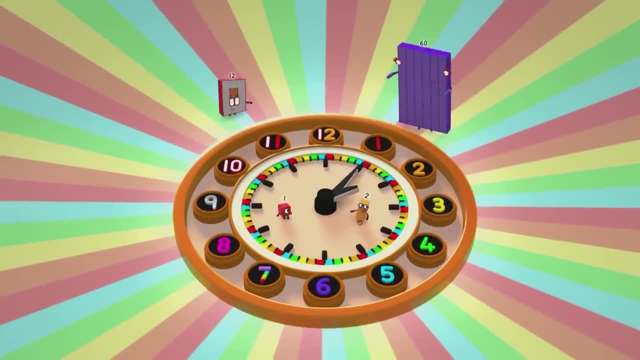 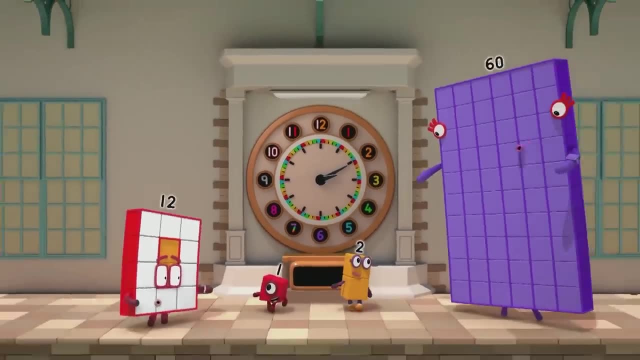 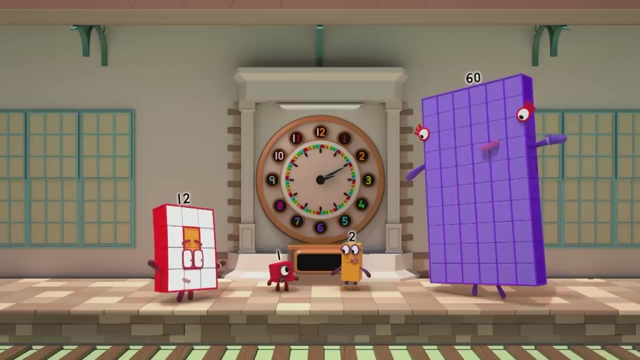 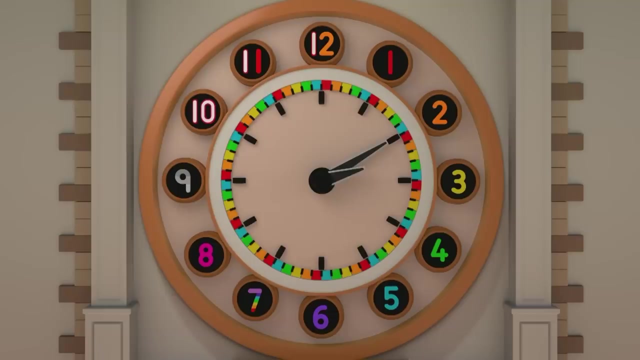 While minutes raced around our face, The hour hand moved on one place And if you put both hands together, Reading one and then the other, You can tell the time. So the little hand, the hour hand, Tells you what hour it is, And the big hand, the minute hand. 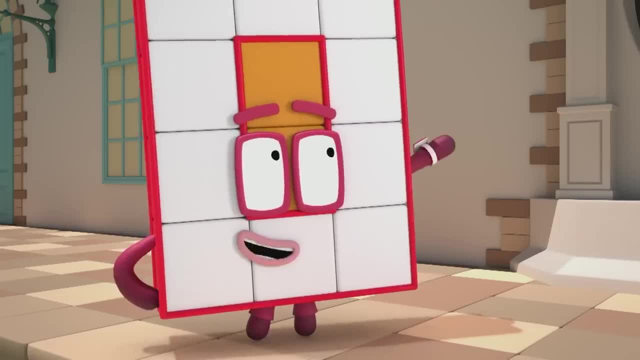 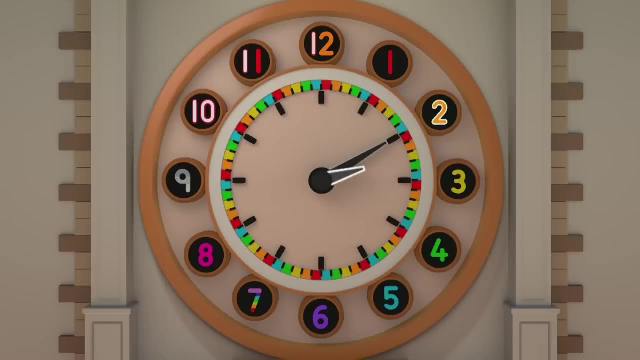 Tells you the minutes of the hour. Say the hours, then the minutes, And that's what time it is. So that big two there. For the hour hand means it's two o'clock Two and a bit, And for the minute hand means it's two. lots of five minutes. 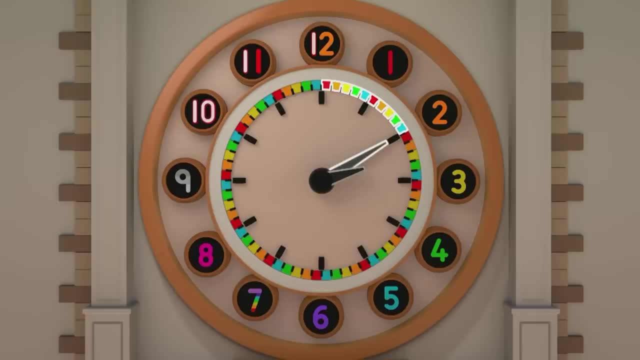 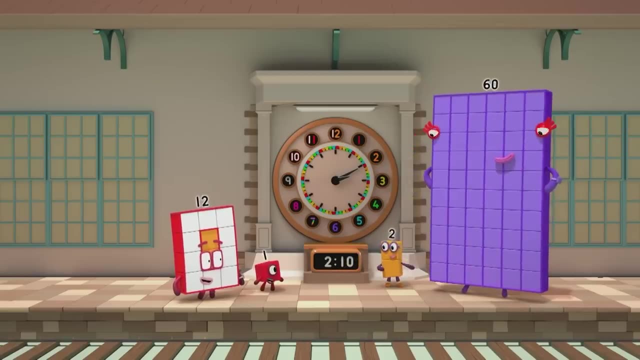 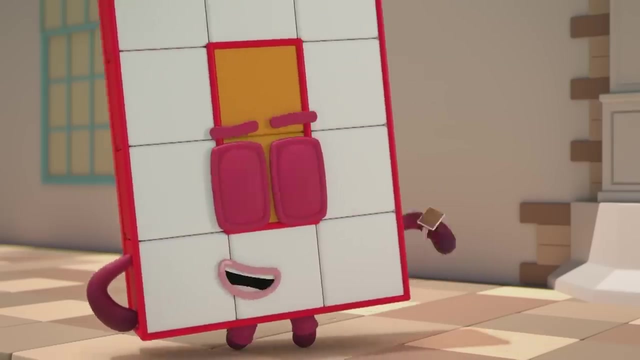 And two fives are ten. So this clock says two, ten, Ding, ding ding. We have a winner. I can do it. I can tell the time. Yay, Well, done Two. I'll get this clock back to the right time. 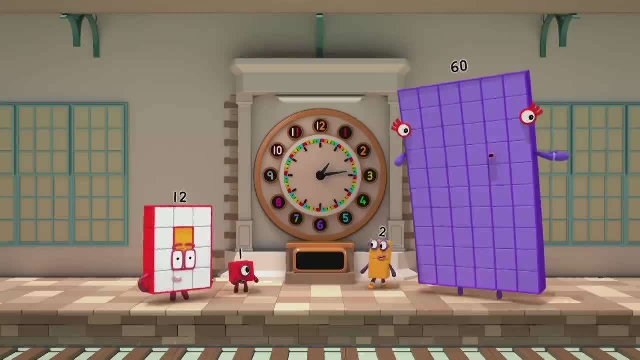 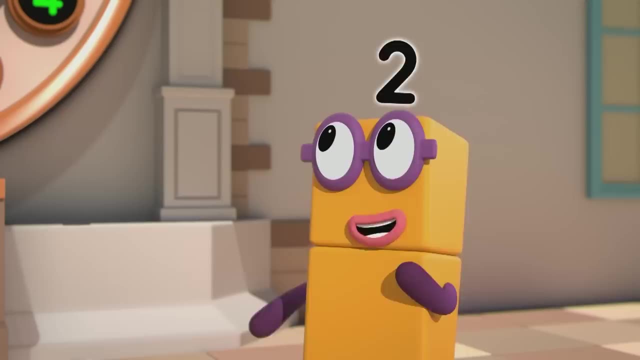 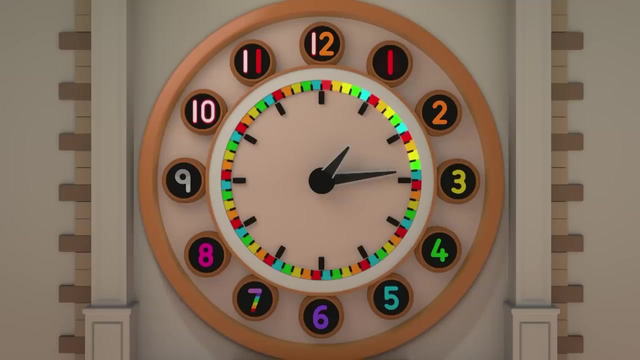 And you might like to know, There's an express train on platform two, Leaving at one fifteen An express train. Then we can still make it to the talent contest, And the time now is one ten, eleven, twelve, thirteen, fourteen, One, fourteen. 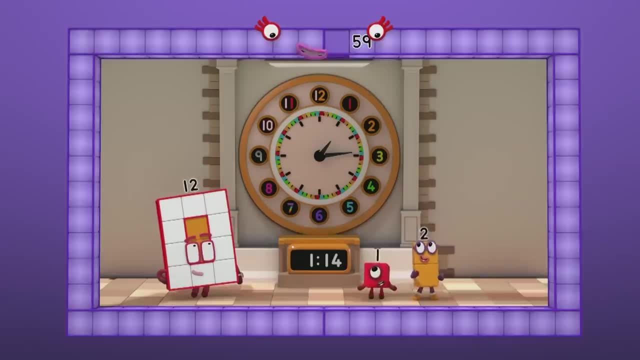 Our train leaves in one minute. A minute, how long is a minute? As soon as you begin, it is ticking away. Each tick and each tock is a second. The sixty, to check on my blocky display. Fifty: it's time to get nifty. 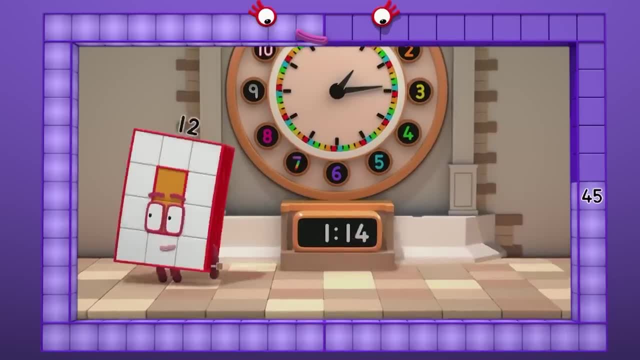 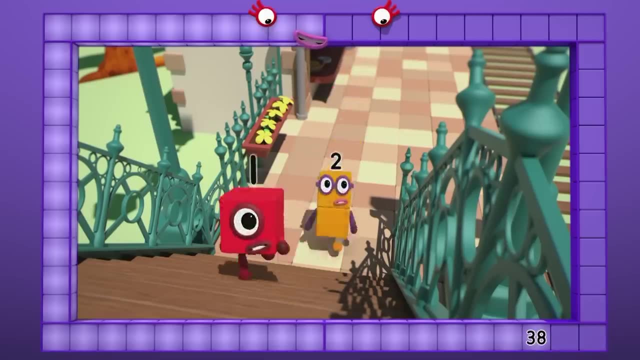 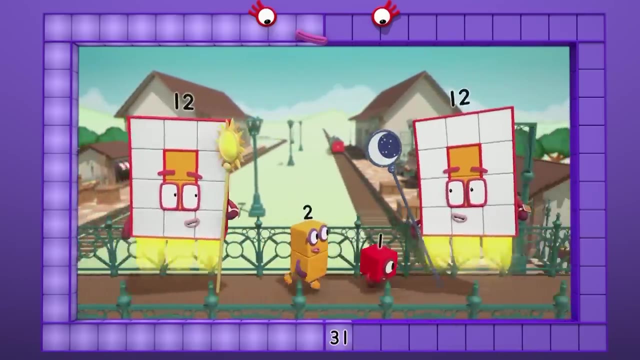 We need to move swiftly to catch that express. Let's hurry, come on and let's scurry. I'm starting to worry We'll have no success. Sixty seconds in a minute. Sixty minutes in an hour. Twelve hours from midday to midnight. Twelve from midnight to midday. 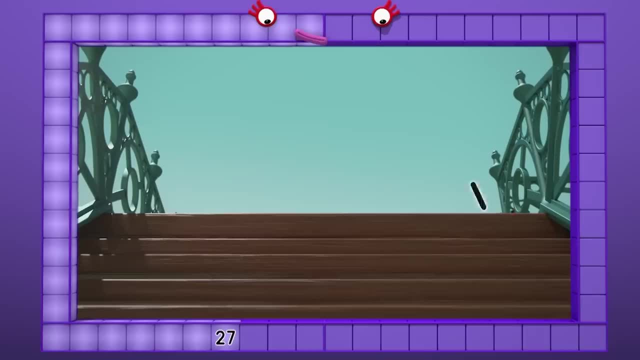 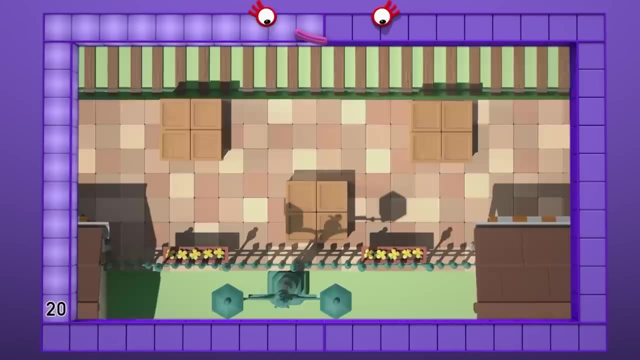 Halfway A minute. how long is a minute? No matter how you spin it, it isn't that long. So breathe. you could just paint a leaf, Or eat a small peach, Or sing a short song Together. each minute's a treasure We're sharing forever. 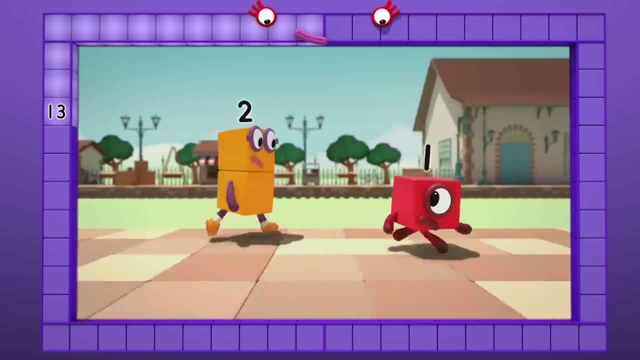 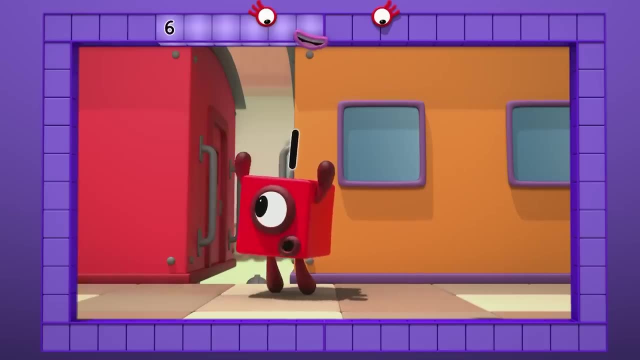 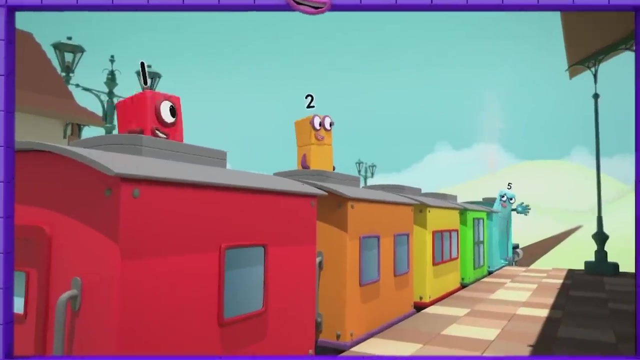 Whatever the news, we'll make it. I know we can make it, We can take it, But let's not mistake it, There's no time to lose. Twelve hours from midday to midnight, Twelve, from midnight to midday, Sixty minutes in an hour, And now we must get underway.